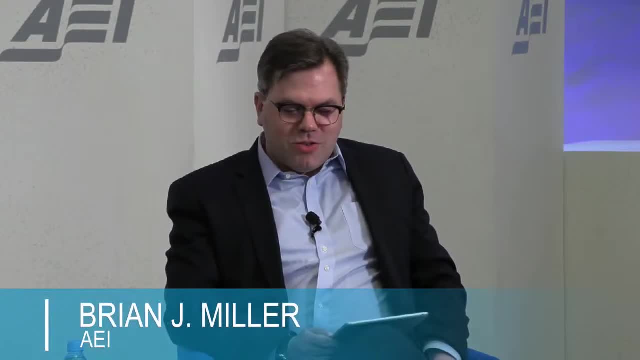 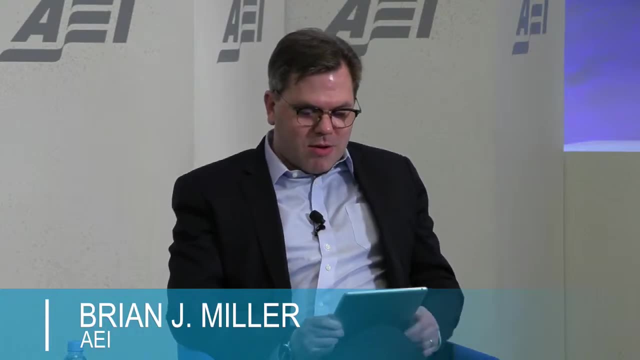 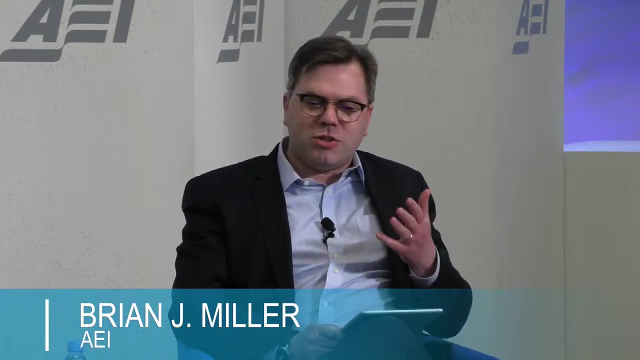 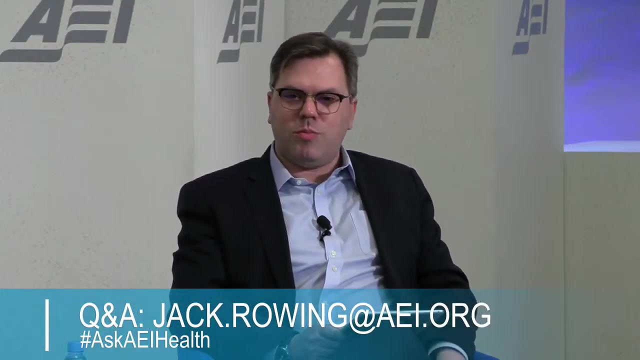 It's like a 747, with manual controls and no autopilot, flying around the world nonstop. So when I think about automation and AI, I think about its ability to transform medicine, be it making sure that I don't have to type notes because it could be automated, automating review of medical records to help approve services faster, augmenting clinicians or even automating elements of clinical practice. 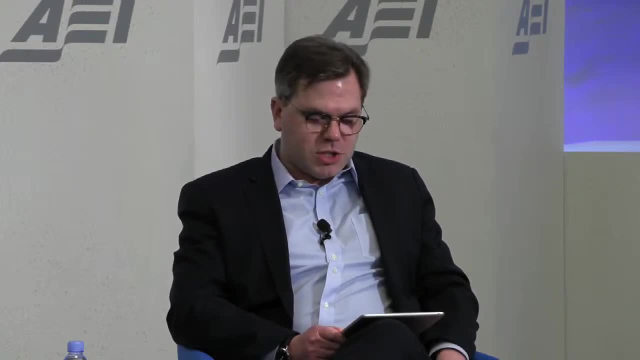 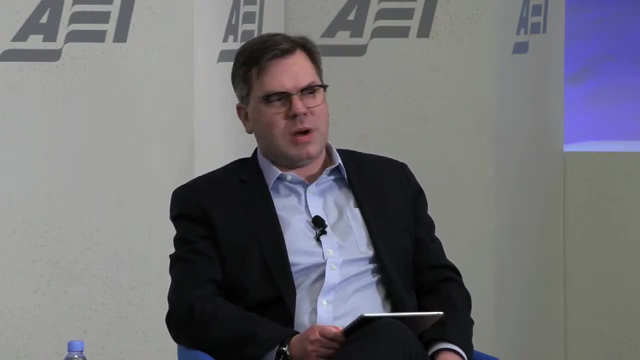 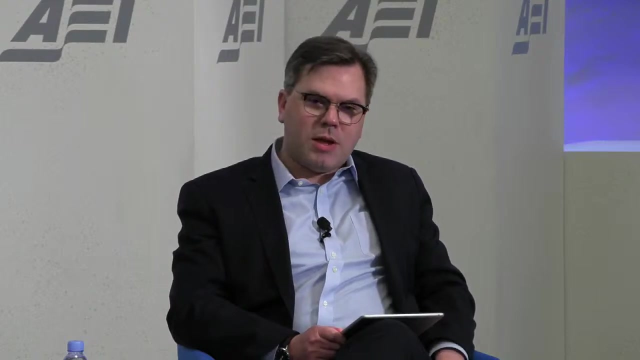 Like pathology or dermatology, to allow the physician to be more efficient, And so our industry has had flat labor productivity growth for over 25 years in the hospital sector. So I look forward to technology transforming this in a positive way and promoting mass-produced, mass-customized health care for patients. 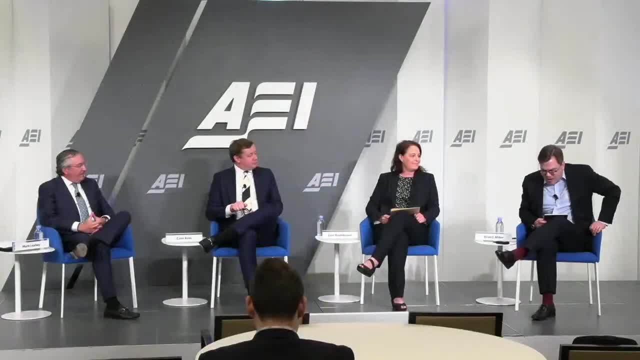 We have a great panel here today. We have my colleague Jane Bombauer, who's a professor at the University of Florida. She's an expert in the law school. She's an expert in free speech and First Amendment issues. We have my colleague Colin Rahm, who's the public policy lead for Andreessen Horowitz's Biotech Venture Fund. 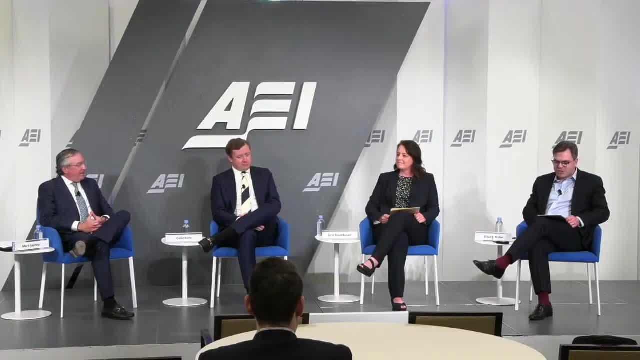 He worked as a senior advisor for the former FDA commissioner, Stephen Hahn, under the prior administration and also worked for the Senate Health Committee. And then we have my good friend, Mark Leahy, who is a bundle of energy and creativity and is the CEO of the Medical Device Manufacturers Association. 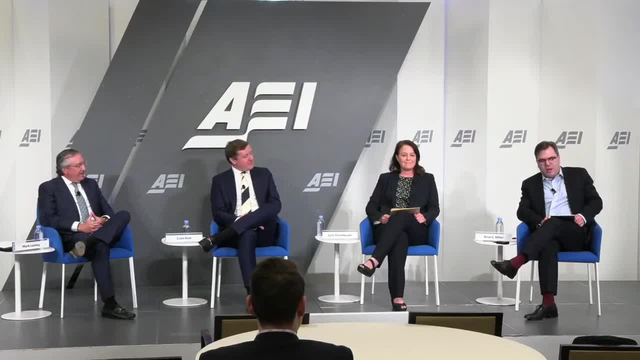 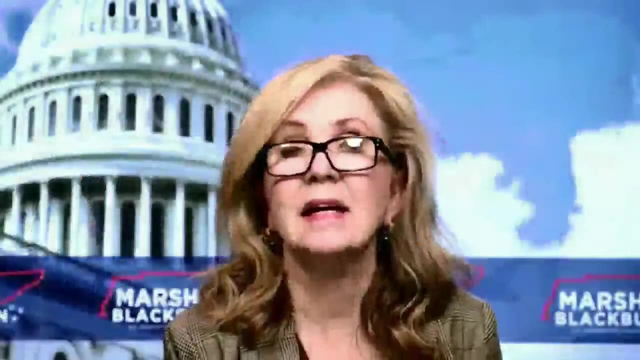 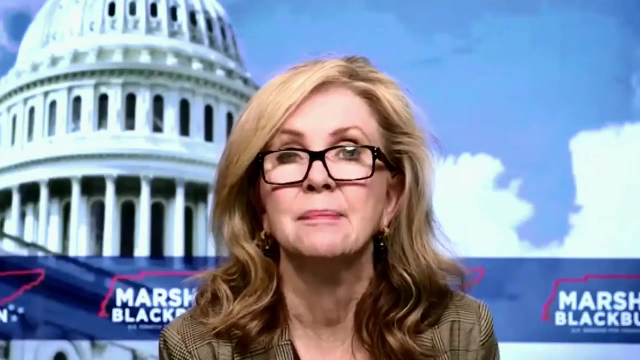 I'm also pleased in that we have some intro remarks from Senator Blackburn of Tennessee, from the Senate Finance Committee, on artificial intelligence and health care. Thank you, Dr Miller and AEI, for organizing this panel today. I wish I could be with you in person, but I'm not. 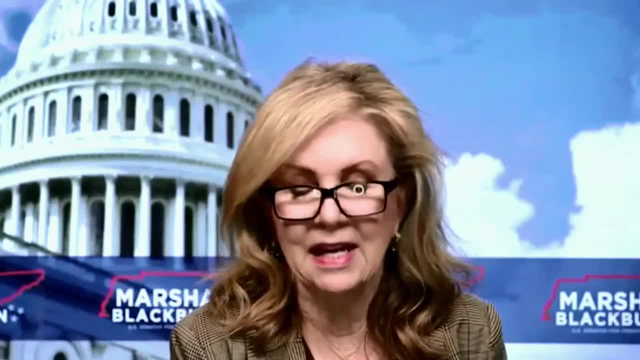 Having to come to you virtually today and I am placing my hand on the liberties. I'm not talking to you. The go talk. Thank you very much and have a good weekend. Thanks, Star, HE continue. Bye, bye everyone. Bye by everyone. 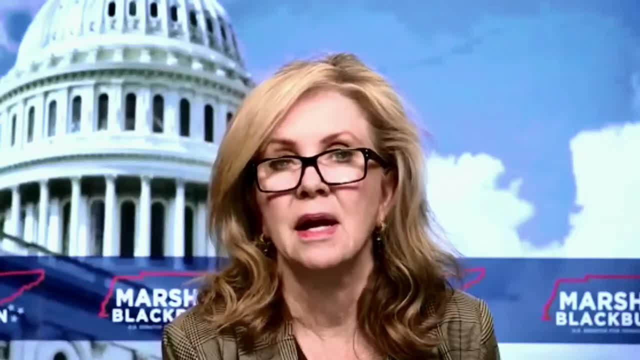 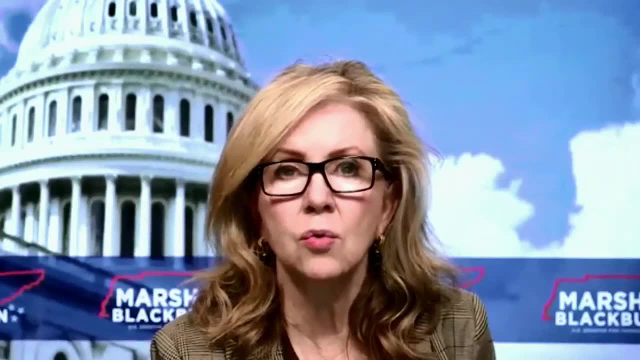 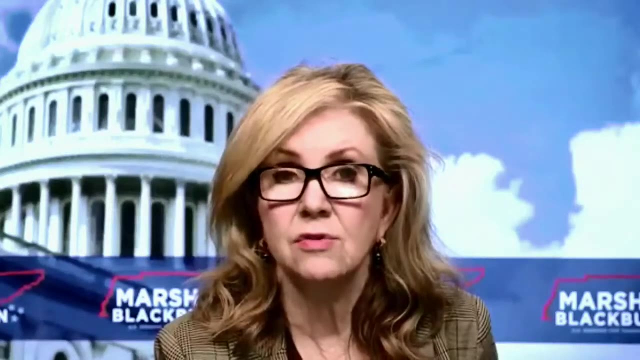 Bye, Bye, bye, Bye, bye. anyone Bye forhand, Bye forhand too. I appreciate the topic, as we're talking about AI in healthcare and the impact that this can have on so many different areas: disease analysis, remote surgeries, predictive diagnoses. 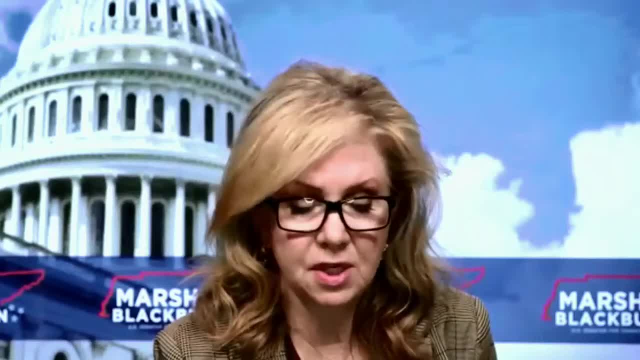 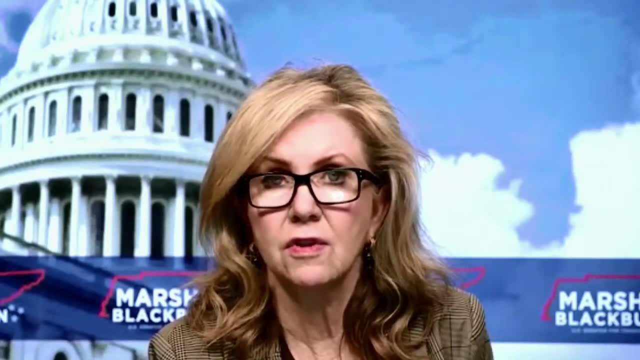 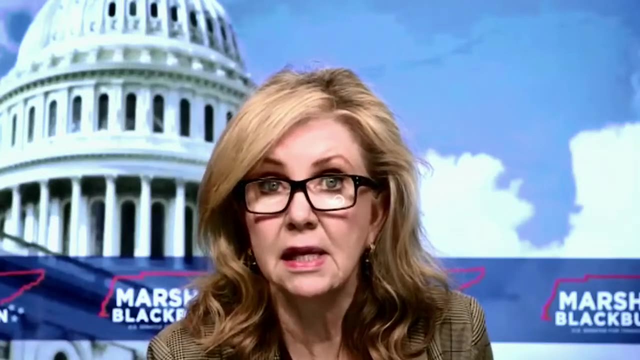 all will make a difference and yield better outcomes for our patients. Technology. what we have seen is healthcare technology over the last 15 years has made a tremendous impact on our citizens and has helped lead to some of those better outcomes I have heard from. 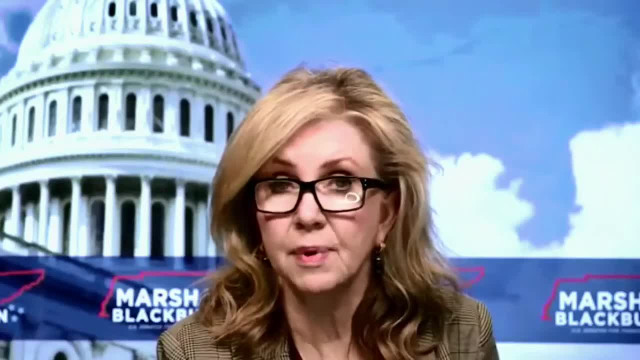 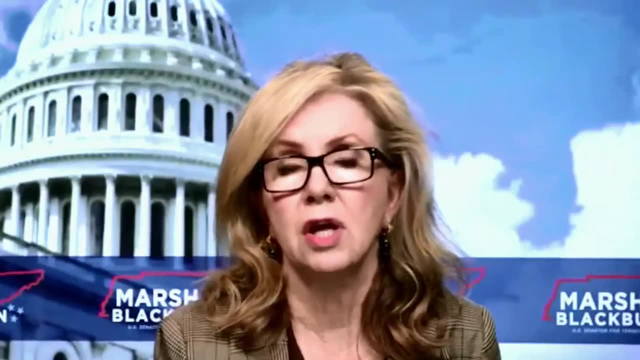 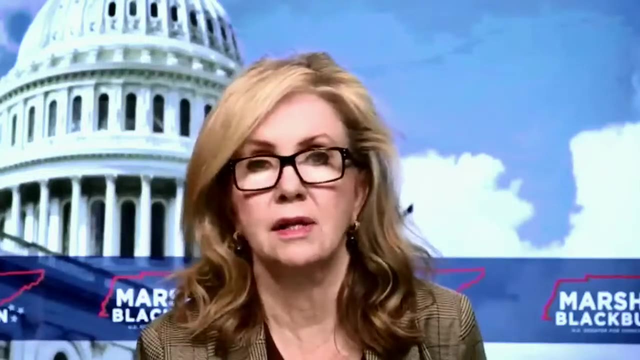 so many providers and hospitals and device companies innovators that are in Tennessee that they are always looking for new ways to use technology and to ask that all-important question: what if we tried this? Or what if we did it a different way? And what they've learned is they. 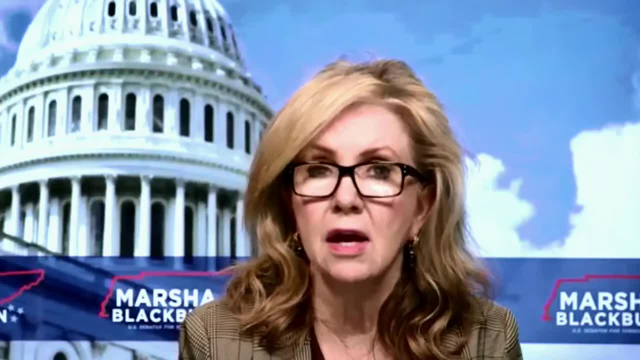 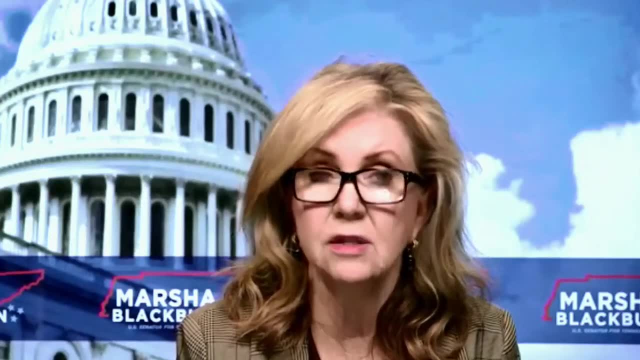 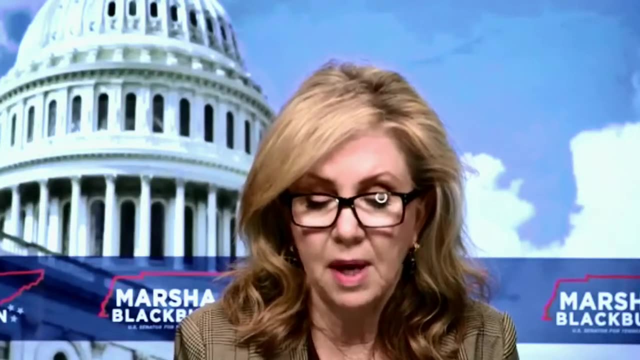 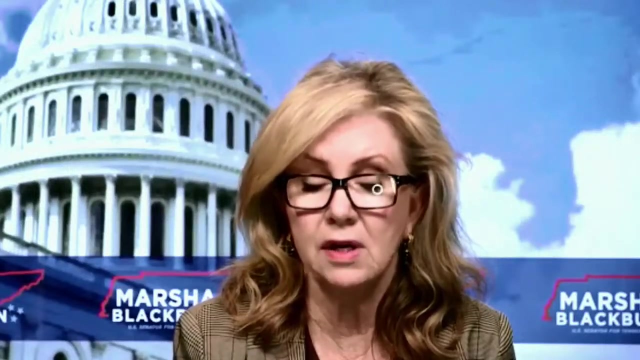 can incorporate AI into their healthcare models and protocols and many times, help get those better outcomes and do it in a reduced timeframe, which, of course, we know is better for the patient. I know that you all are going to look at several topics today. One of the things that we're going to talk about today is the automation of administrative tasks. 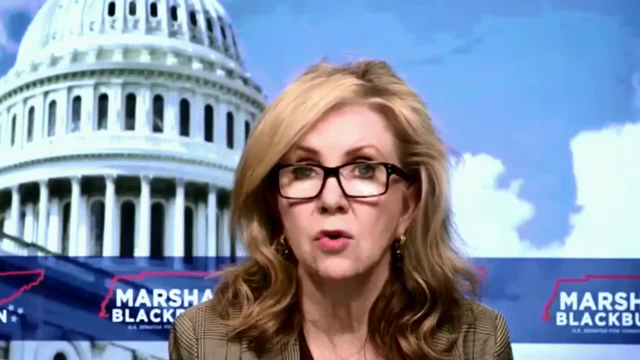 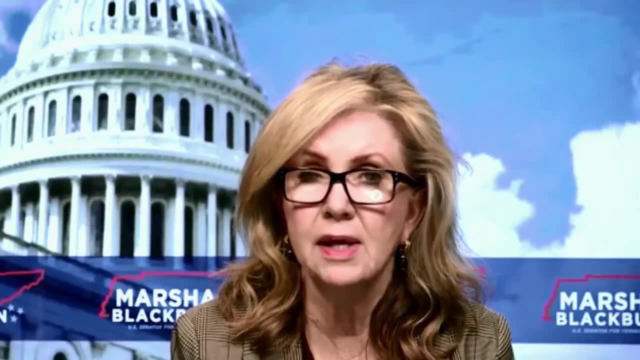 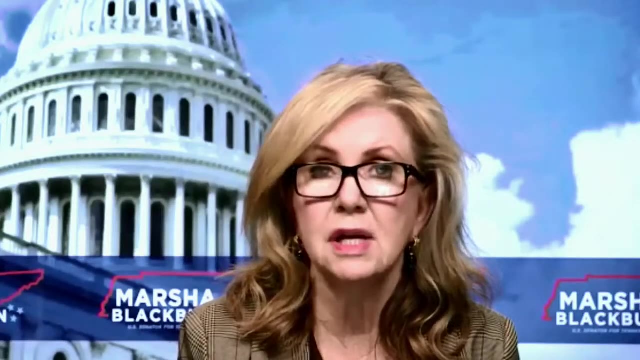 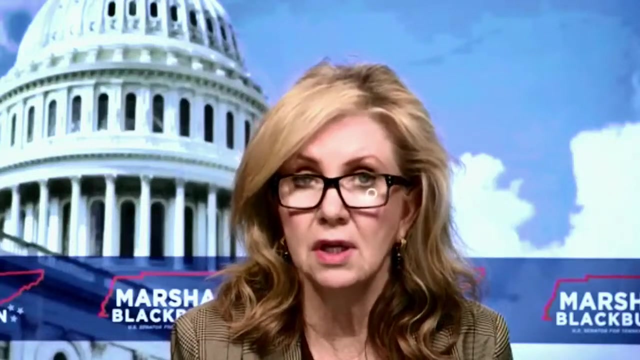 so that providers are spending less time on compliance and more time working with the patient, talking to the patients. Also, you'll have a discussion about the ways that physicians can use AI to achieve those better outcomes and how programs like Medicare can support those better outcomes. If you have a question, I'll dial it back to you. 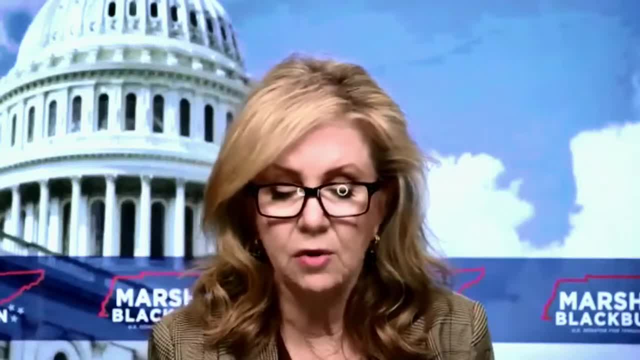 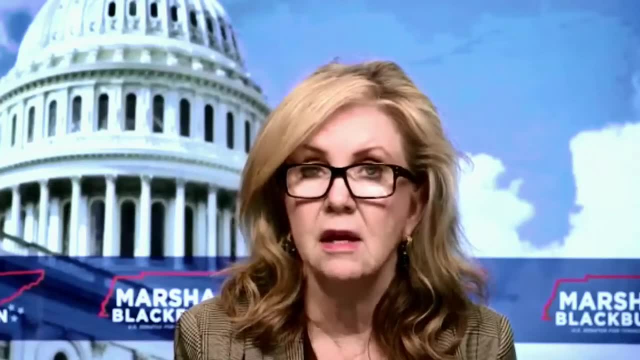 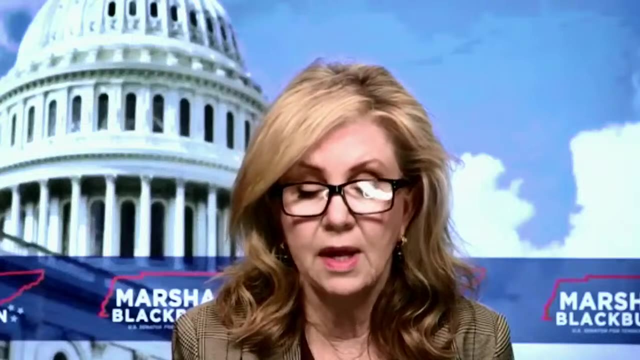 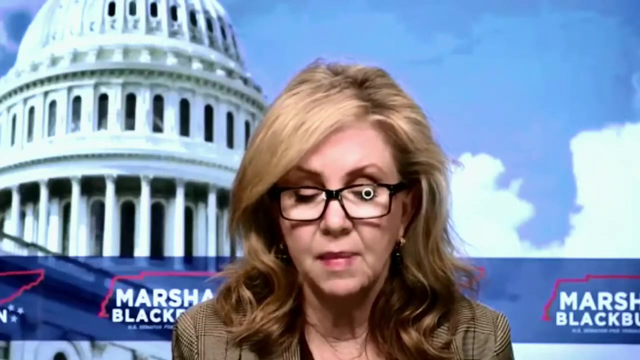 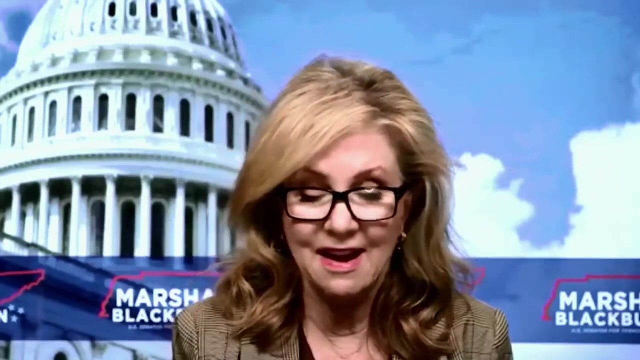 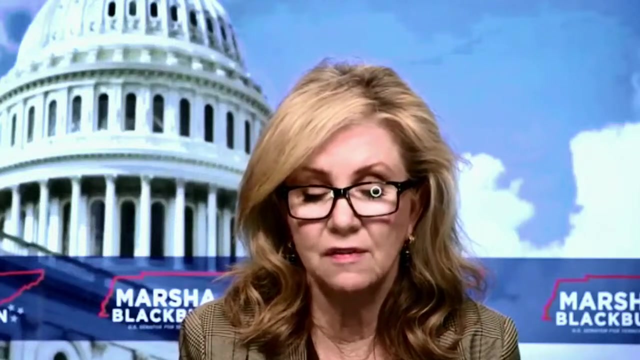 I wonder what role has medication technology played in the pandemic, particularly when it comes to Authorization Act or, as we call it, MACRA? Everything's got some abbreviation, doesn't it? And MACRA was in 2015,, and it really started that shift from fee-for-service to value-based care. The care model has improved outcomes, It has reduced cost, It has elevated patient care quality And we have more work that we're needing to do as we look at alternative payment models and address reimbursement challenges, especially for our rural and underserved communities. 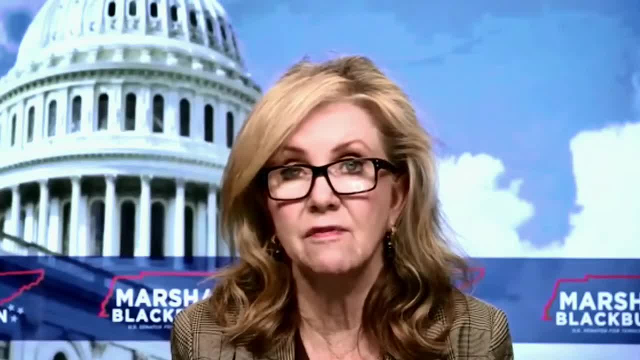 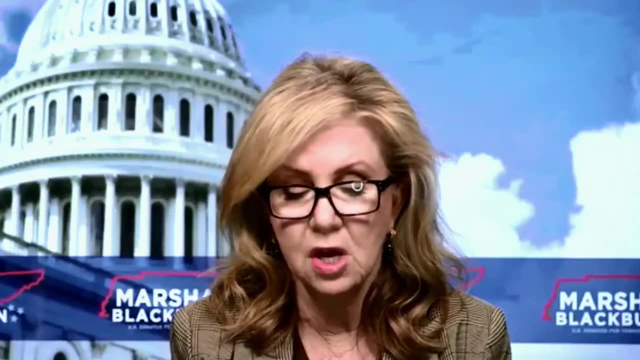 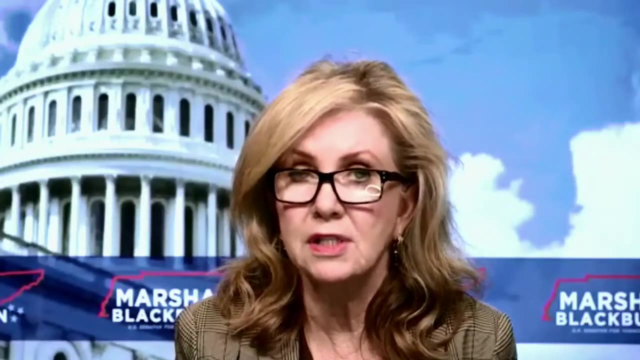 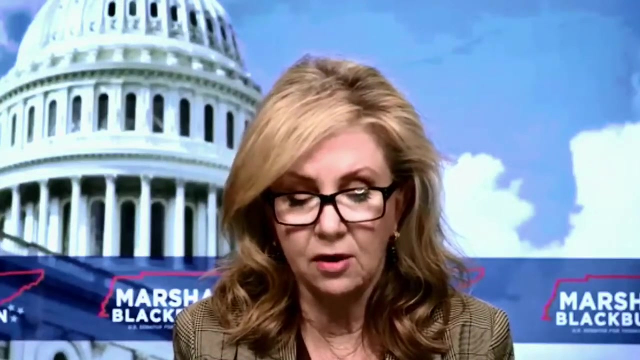 And that is why I have joined a Senate Finance Committee working group that will explore and propose policy solutions for stable physician payments. Thank you, Things that are going to be predictable and consistent, And we'll propose necessary updates to MACRA ensuring sustained access to quality for patients. 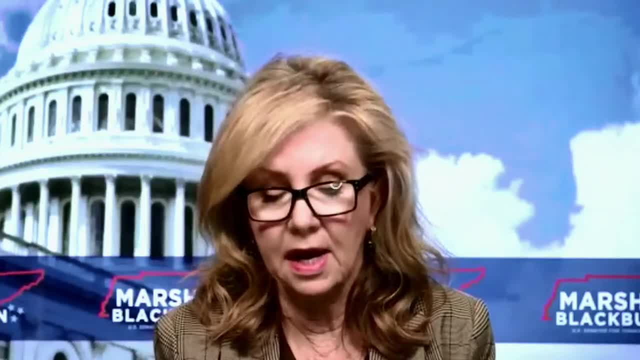 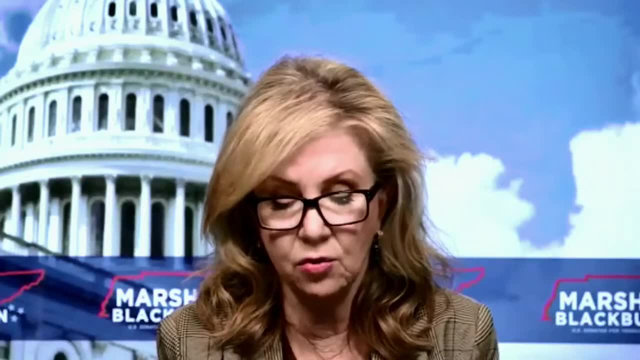 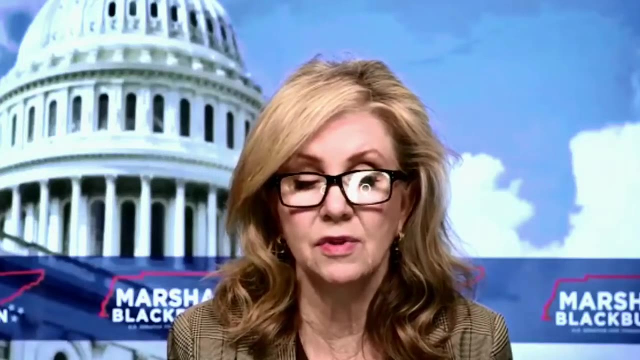 How Medicare reimburses providers for AI utilization will be at the forefront of the conversation that my colleagues and I will have in the working group, And we would appreciate hearing. We'd also like to hear- from you, because you're the ones with expertise on this issue. 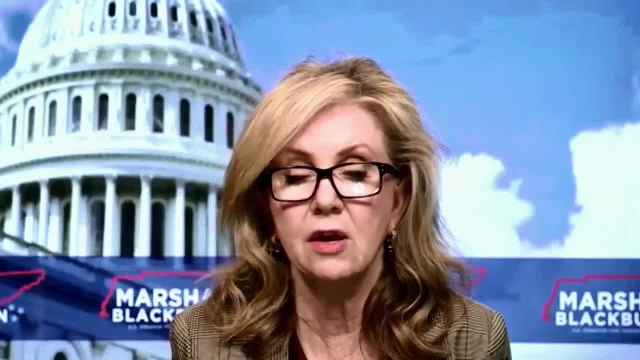 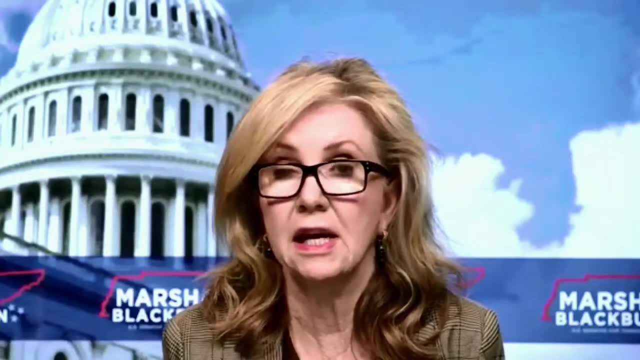 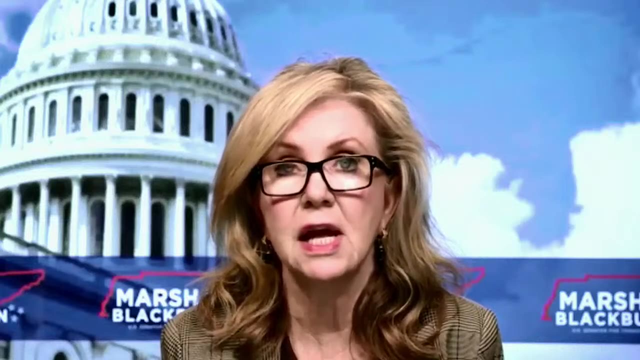 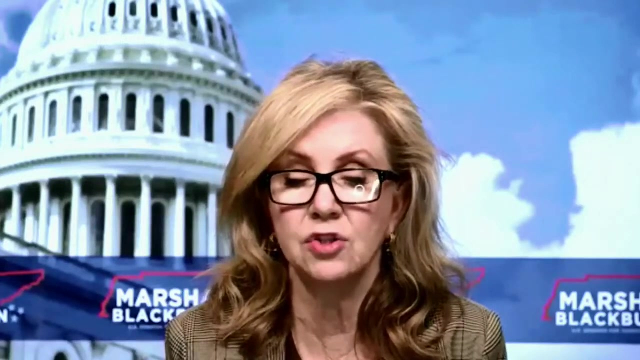 The integration of telehealth and virtual care has become instrumental in providing more accessible healthcare services. Telehealth's ability to overcome geographical barriers and facilitate timely interventions has proven to be invaluable. I'm looking forward to hearing insights on how we can leverage virtual care. 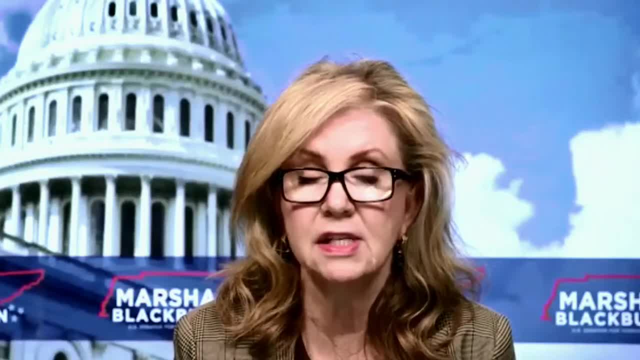 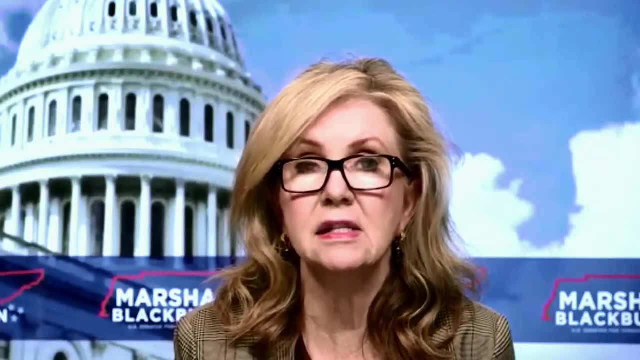 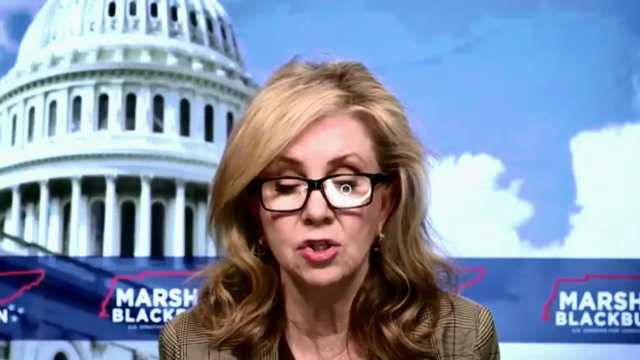 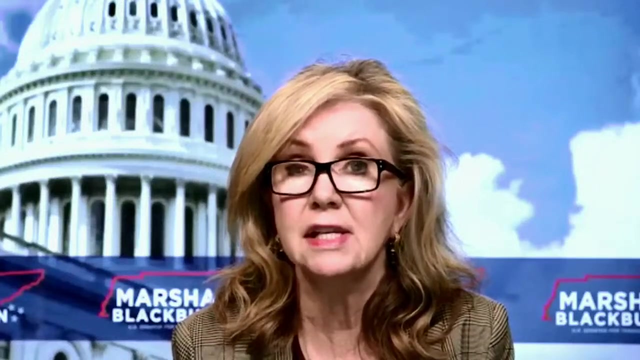 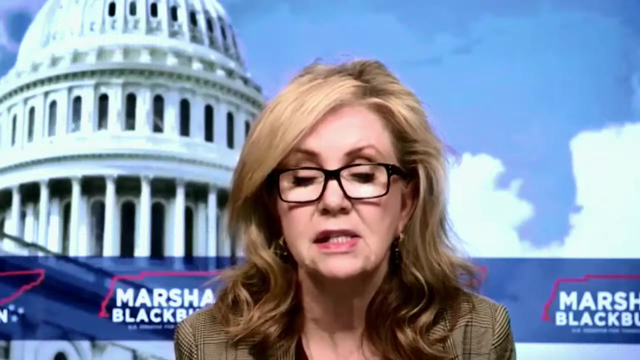 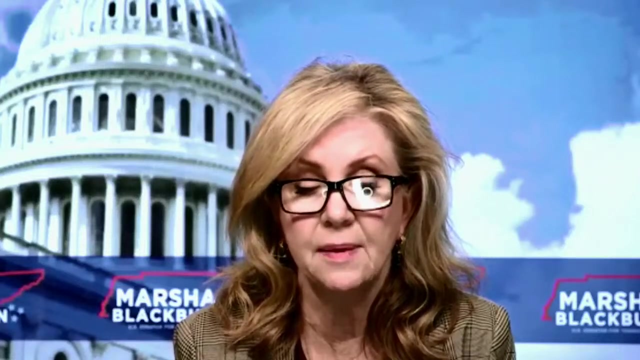 and remote patient monitoring technologies in every setting, and discussing strategies in scaling these innovations, especially in AI. The growing emphasis on regulating emerging technologies requires careful consideration of AI's unique challenges and the opportunities From diagnostic support to predictive analysis. AI holds significant potential in transforming patient care and operational efficiency. As we discuss, 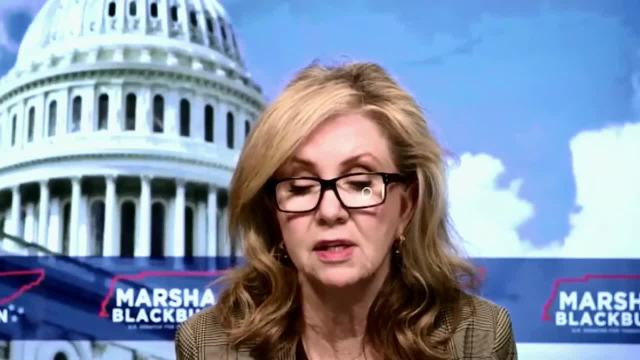 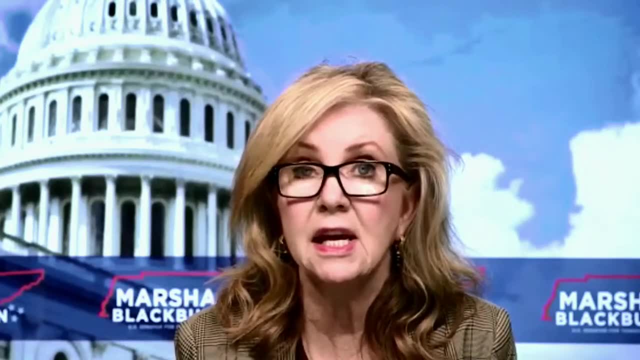 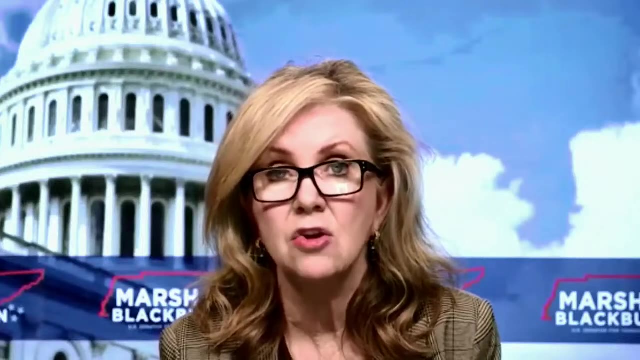 let's focus on how we can leverage AI for positive transformation while addressing ethical considerations, including privacy and data security. I encourage each of you to see the next slide. Stay in touch with our office. You will find me at blackburnsenategov On social media. 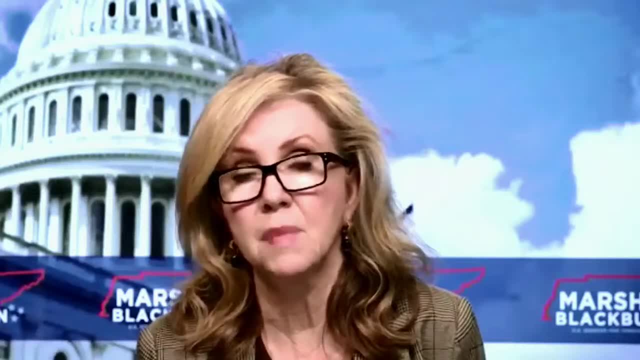 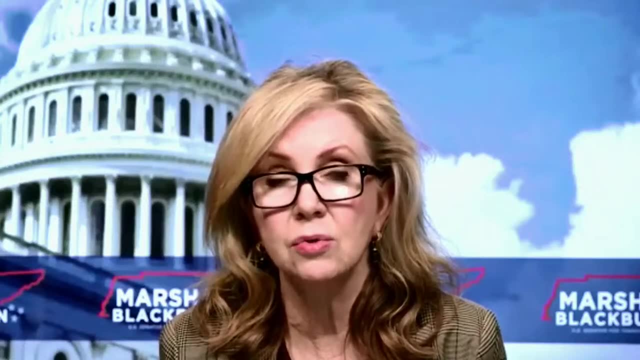 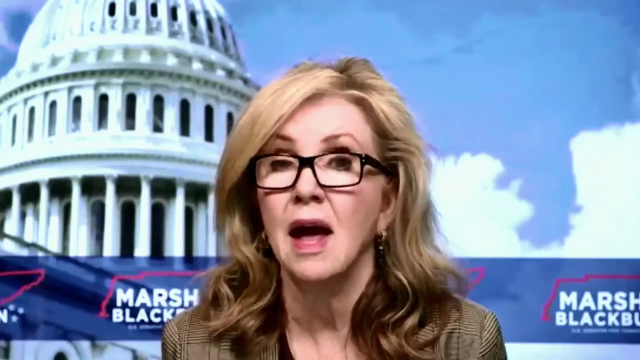 I'm at Marsha Blackburn. It's important that members of the Senate hear from you and realize the work that you are doing to solve some of these problems when it comes to payment models, when it comes to value-based care and when it comes to better outcomes for your patients. 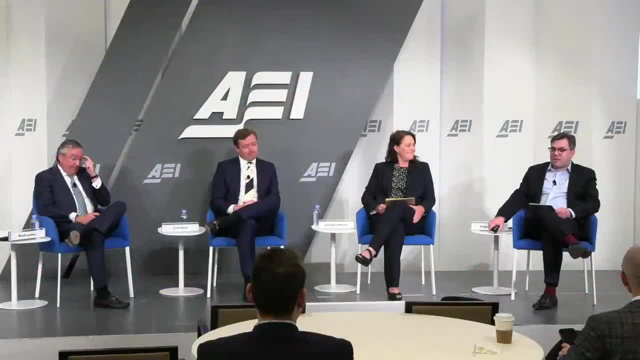 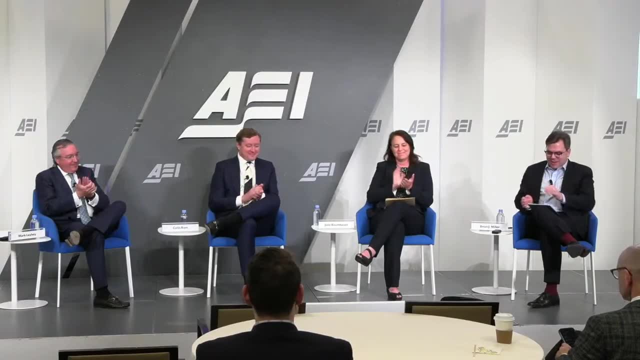 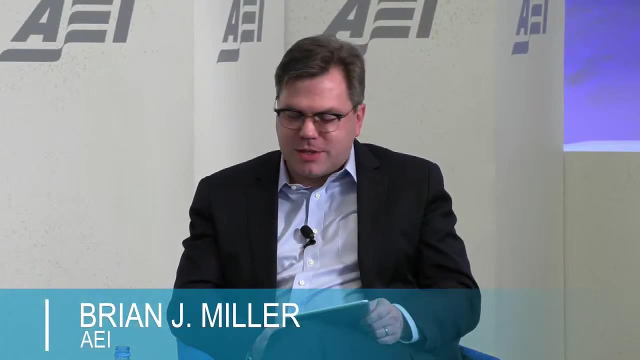 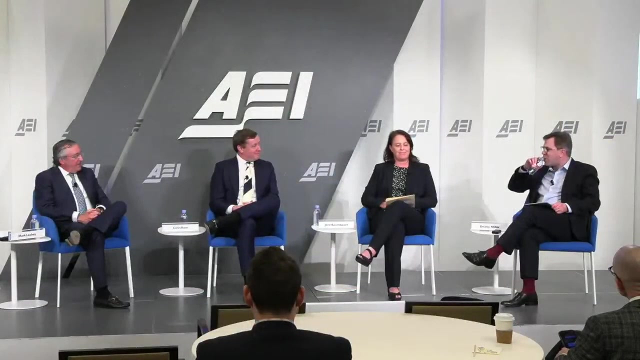 Thank you. Just a round of applause for her Apologies that she could not join us in person. I'd like to start with intro remarks from each of our panelists, starting with Jane. Okay, So Brian introduced me as a free speech or First Amendment professor, and so you might. 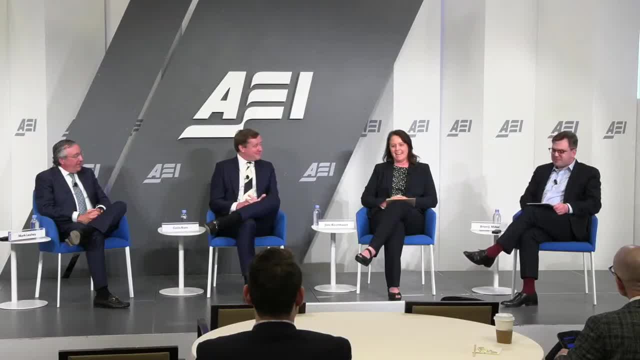 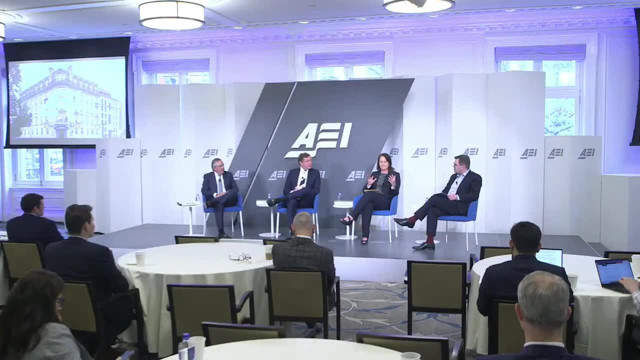 be wondering what I'm doing on this panel. So I come as a useful, hopeful and useful outsider to the field because as a First Amendment specialist and also a torts professor, I think that's important too. That'll come up a bit. I tend to see the whole regulatory 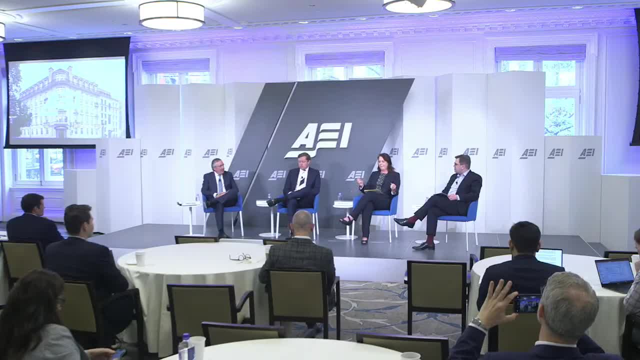 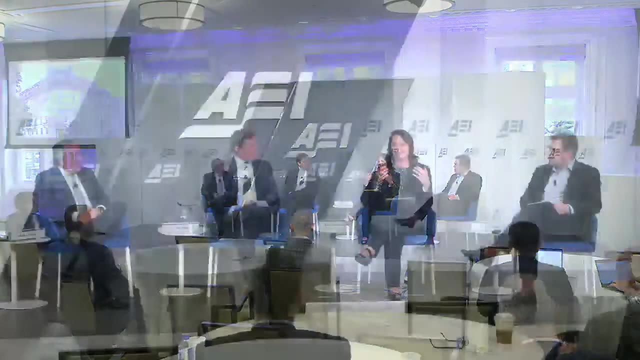 operation that's currently in place very differently. So, on the First Amendment side, a lot of the – not all, but a lot of the AI applications that I think we're the most excited about are the sorts of things where an AI tool takes in and analyzes data and then spits out much. 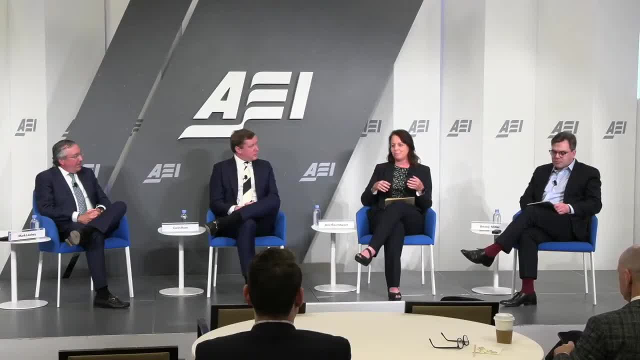 much more information. So you know whether it's a decision support tool or a diagnostic tool or a treatment recommendation system. these are all forms of speech. It doesn't mean that they're not risky- Of course they are. There are risks presented with this type. 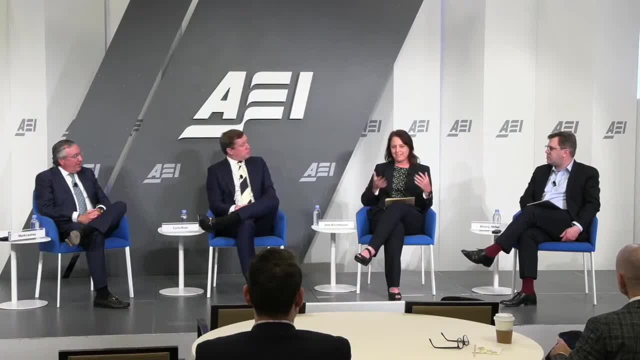 of information. If a diagnosis is wrong, it's probably the most obvious example. But the harms come from the, you know, expected reaction of a listener. Okay, And so that means we're still in the domain that free speech law has been tackling from. 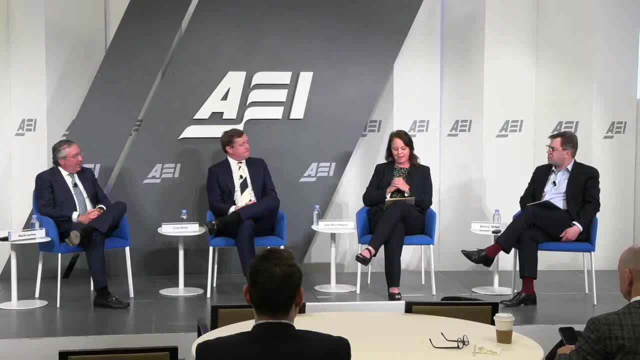 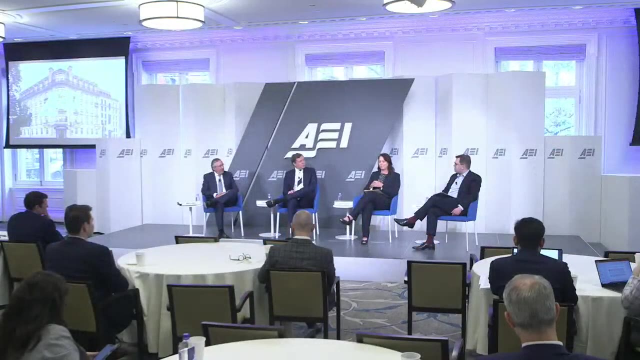 the beginning of the modern First Amendment era, And what that means is that regulation of pure speech products, which is what I think many of these tools are going to be, has to be well-tailored to real-world and non-speculative risks and should probably follow some rules. 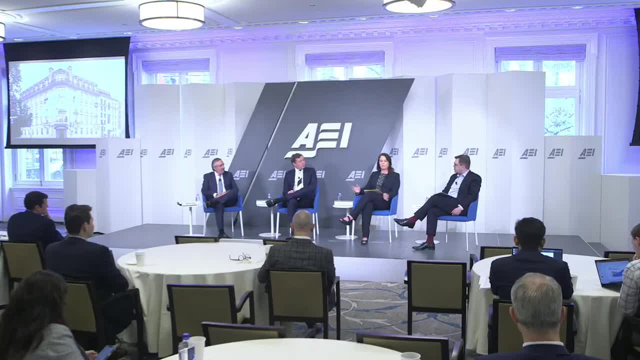 of thumb that have been developed in case law. Okay, And so you know we're still in the domain that free speech products, which is what I think many of these tools are going to be, has to be well-tailored to real-world and 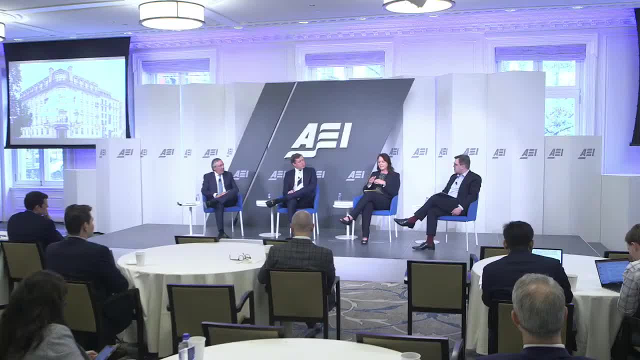 non-speculative risks and should probably follow some rules of thumb that have been developed in case law both inside and outside the First Amendment, and health law kind of interface. And then really quickly I'll say, as a torts professor I also see the direction that the 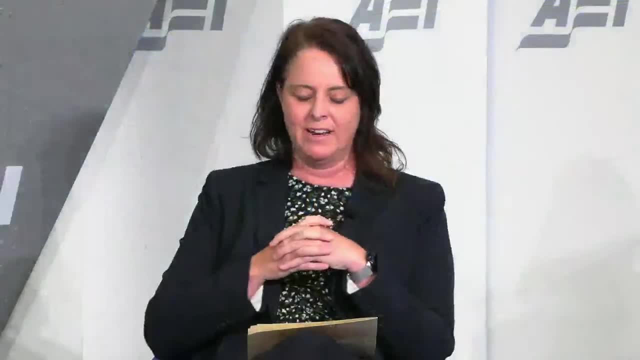 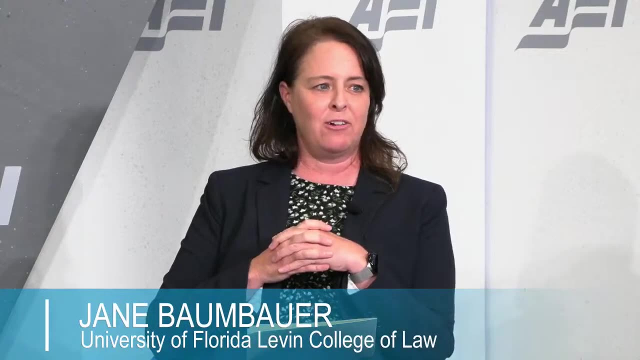 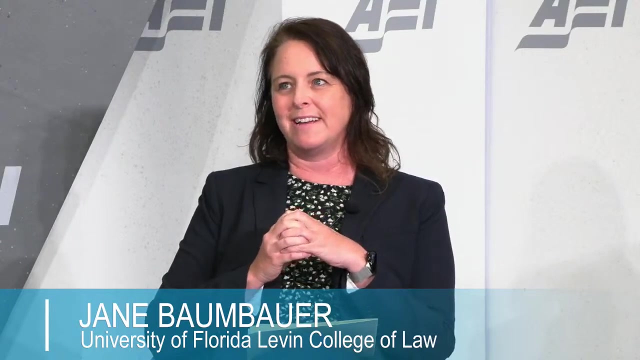 conversation has been moving in AI regulation as somewhat, if not troubling, at least kind of unusual compared to how we manage risk in most other sectors. So if you think about other products like cars, or at least you know- if you think about other products like 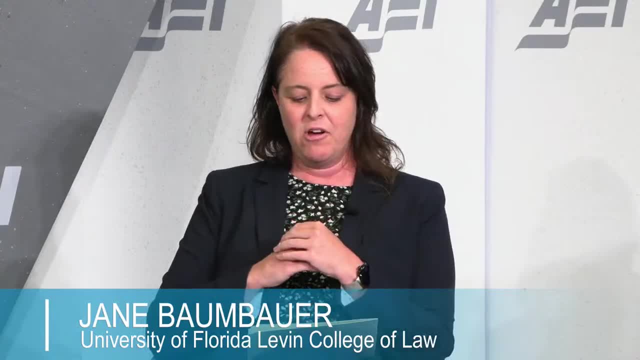 cars, or at least if you think about other products like cars- or at least you know car, or at least you know cars- or activities like running a railroad or something. all of these things, of course, involve both innovation and risk, And the system in the United States. 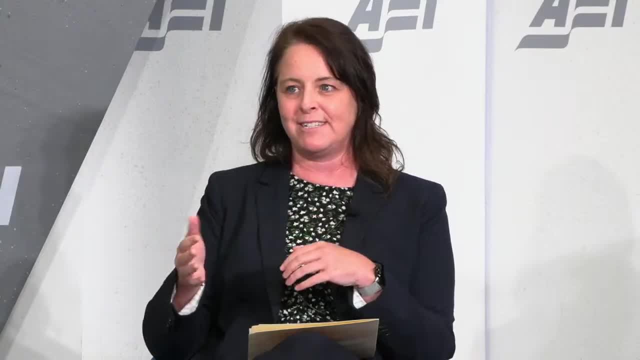 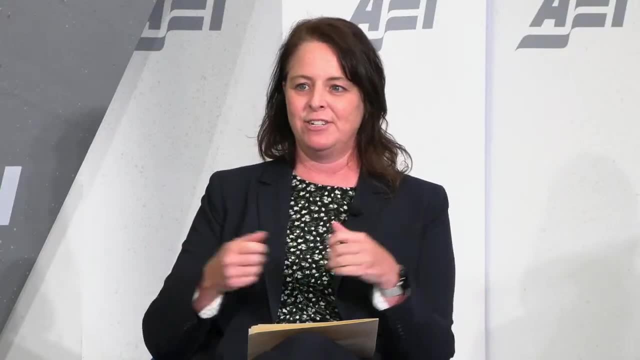 has historically been for X post and fault-based liability rules. So what I mean by that is: nobody says in advance whether you can or cannot do something. but if you do do something and you took on a risk where you know it was totally foreseeable that there'd be a. 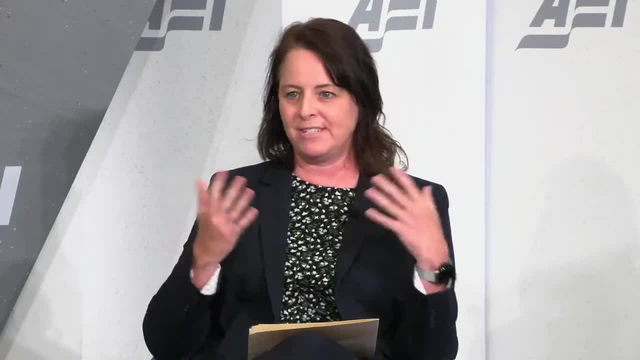 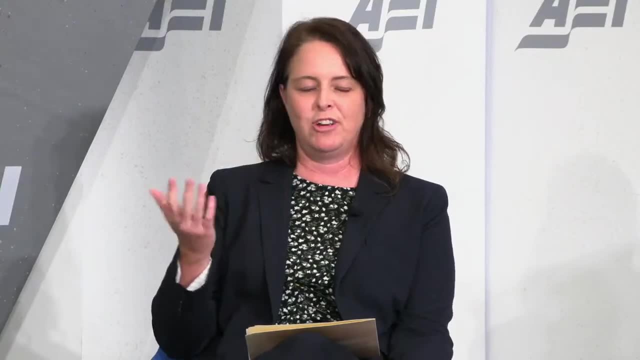 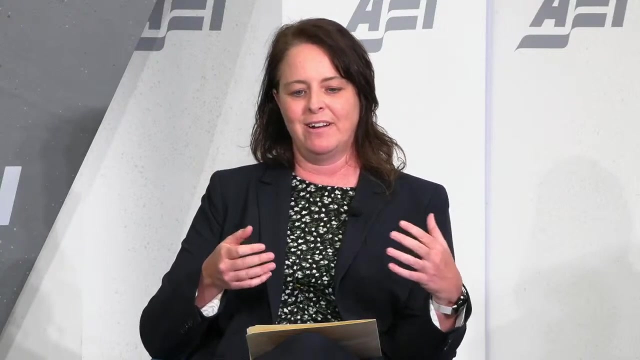 risk that could have been reduced through some cost-effective precaution. what would effective precaution then, and only then? will you actually have to pay, change your product or whatnot? Drugs have always been a special case because of the inherent uncertainty of not only among 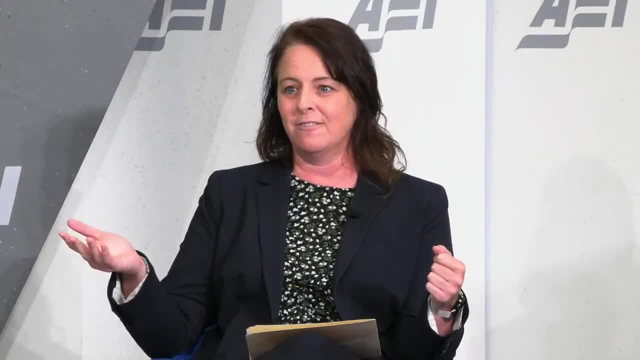 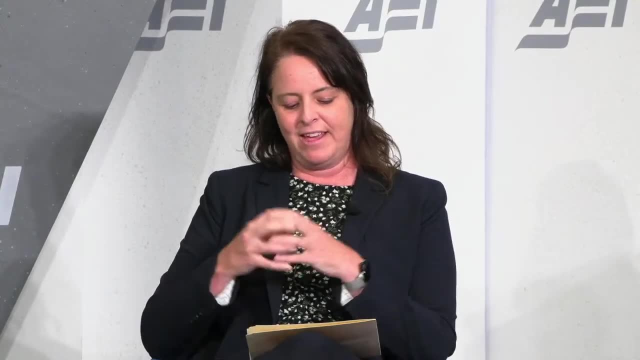 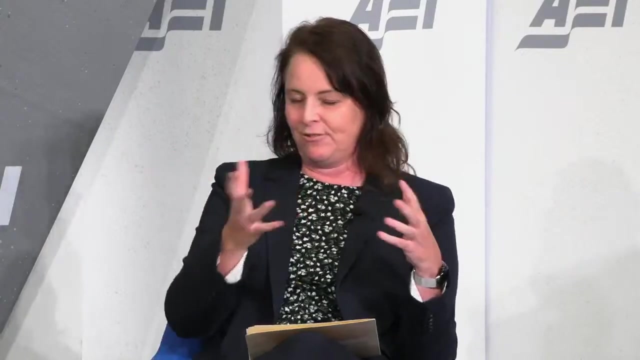 the consumers or doctors, but even the producers themselves, about what types of risks are going to emerge and whether the benefits are as good as we hope they will be, And so I think the tendency has been to slot AI into a drug-like model or devices sort. 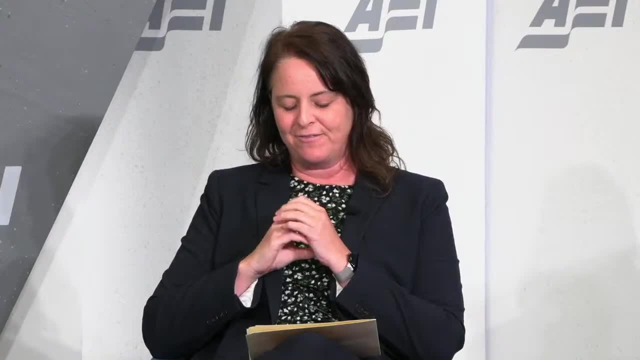 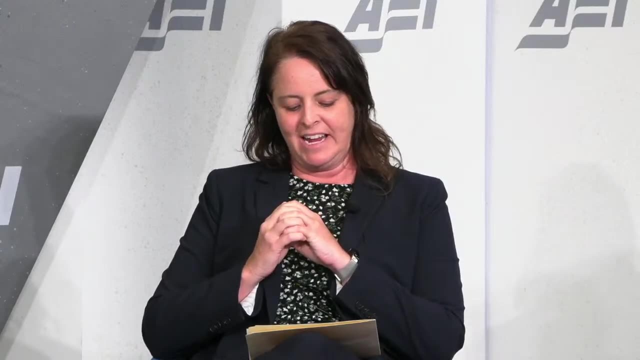 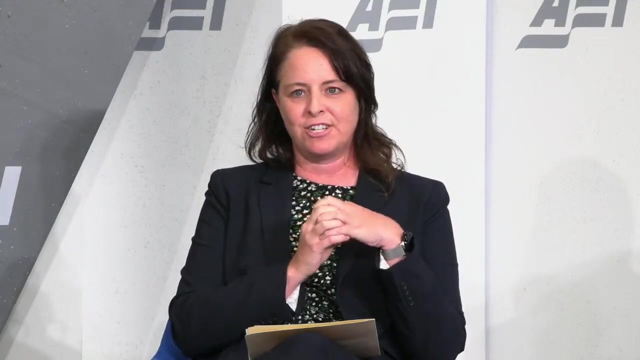 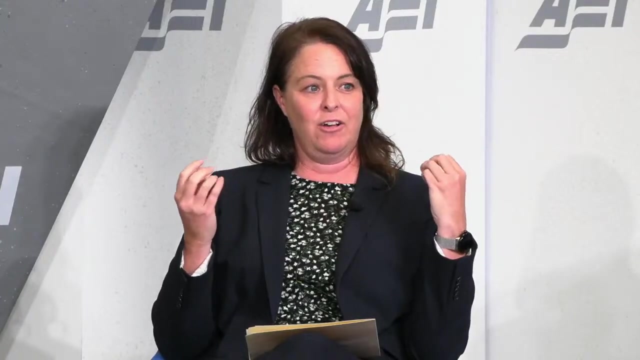 of also follow the drug-like model, out of sort of an abundance of caution and an understanding that we don't quite know what the risks are. But there are serious opportunity costs to treating AI under this kind of precautionary approach, Whereas a more open system where new entrants can first of all work out for themselves that. 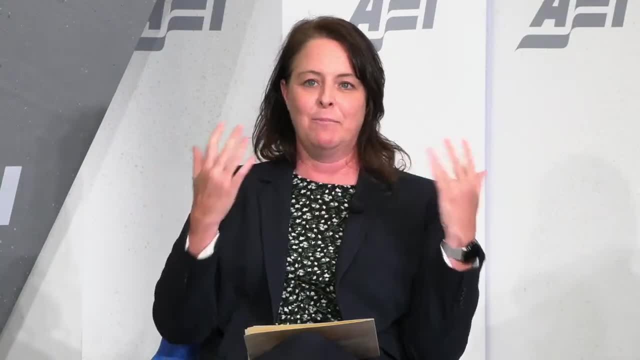 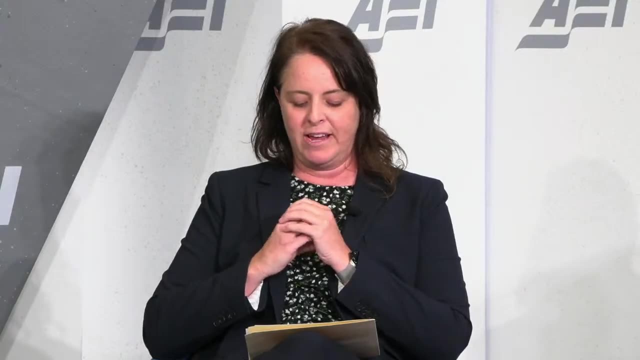 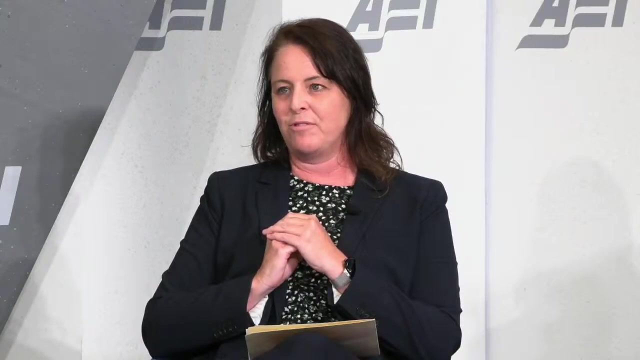 they're not at too much liability risk. do their own testing, but then go ahead and roll out and try their products out in the real market rather than having to wait in a very long line for pre-clearance. I think the benefits of that approach are going to be significant. 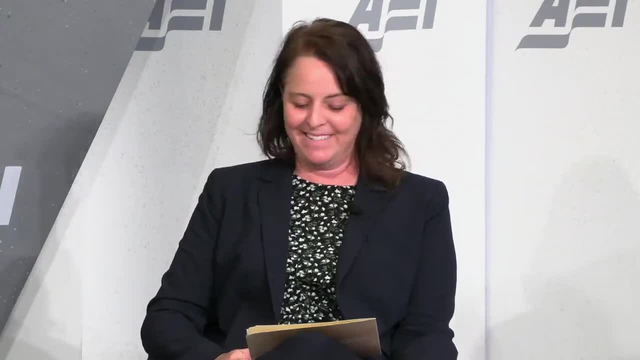 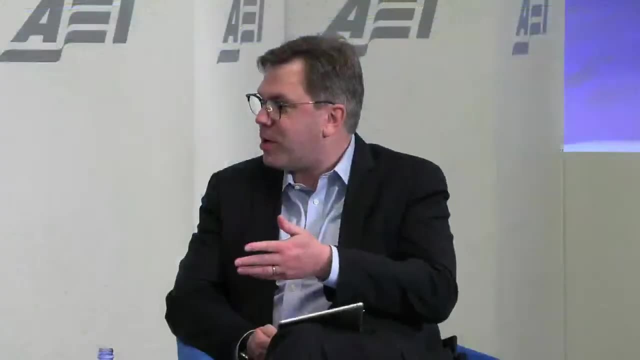 and the risks can be managed. So I'll leave it there, Thank you. And two sort of comments in response to that. One is I did watch. we talked about non-speculative risks. I did watch Terminator in preparation for this panel. 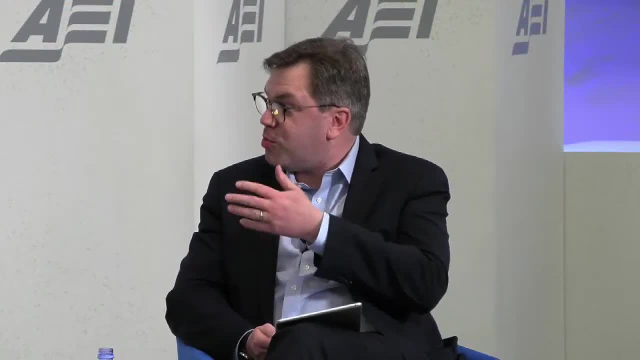 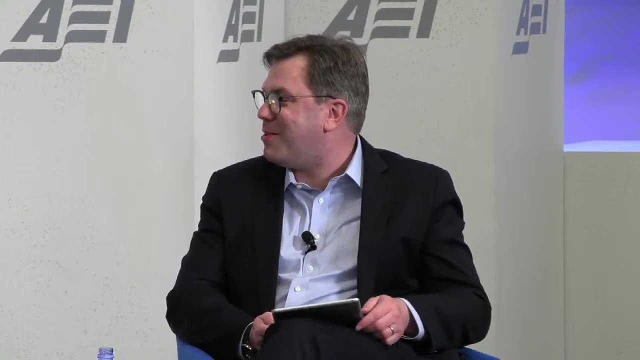 And then my convertible, which I drove here, did go through pre-clearance- obviously all components did- before it was on the market. Yeah, it was pre-clearance reviewed by a regulatory agency before it all ended up on the market in 1999.. 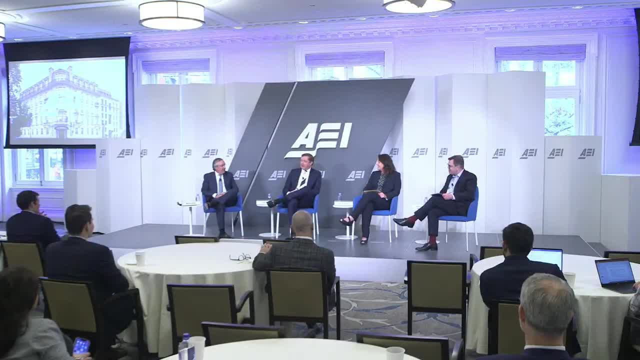 Colin. Thanks, Brian. I'm Colin Rahm. I'm head of public policy at Andreessen Horowitz, a Silicon Valley-based venture capital firm focused on technology and its integration across every sector, from financial services, pure tech, consumer tech, business to business. 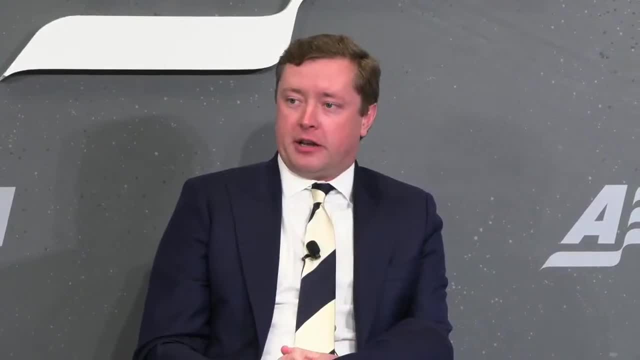 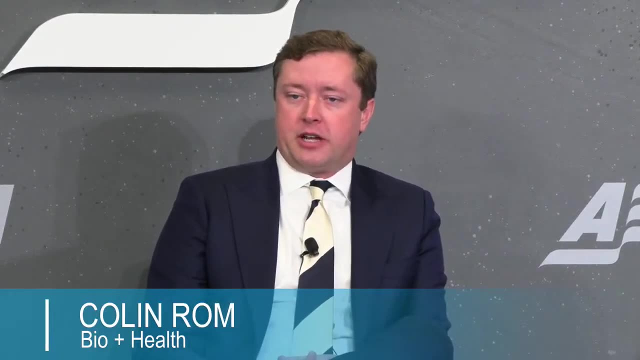 And our most recent. we have crypto. and then we also have American Dynamism, which is focused on technology integration into American preparedness, And then I'm here to represent our life sciences and biotechnology practice, One of the things that we've been focusing on, and it has been really central to our 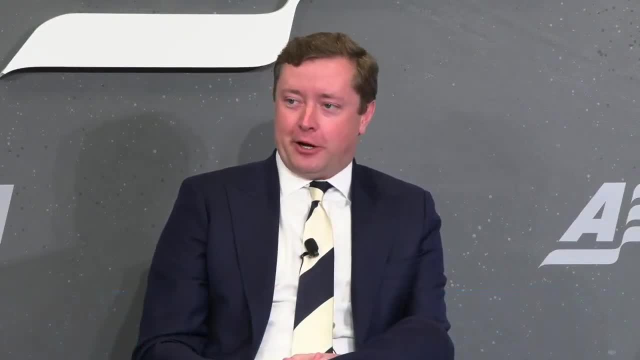 interest in playing a role or at least having a voice. Our opinion here in DC is: artificial intelligence has been central to the investment thesis in our life sciences and healthcare practice since 2013.. Our practice was founded by Vijay Pandey, who was the lone computational data sciences. 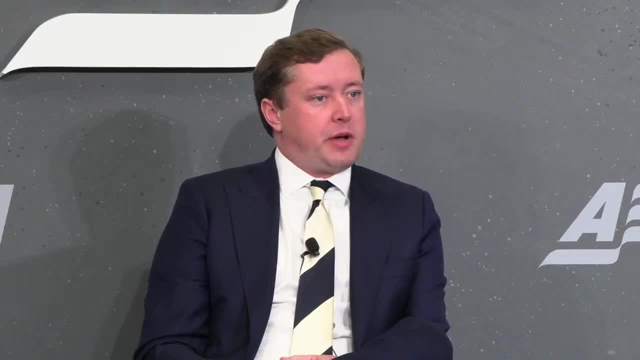 and biology. he ran the lone computational and data sciences biology lab out of Stanford in the mid-2000s and then has started to see that integration long term. So I think, as we're seeing all this new interest, or what seems to be new interest- from Congress, 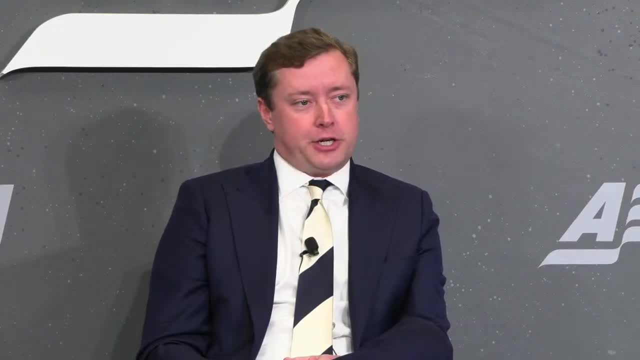 and regulators around how to regulate this new technology and its integration. we've largely had the opinion that this is not new and largely you're just seeing this new kind of interest because people haven't been familiarized with its impact and how it's already being. 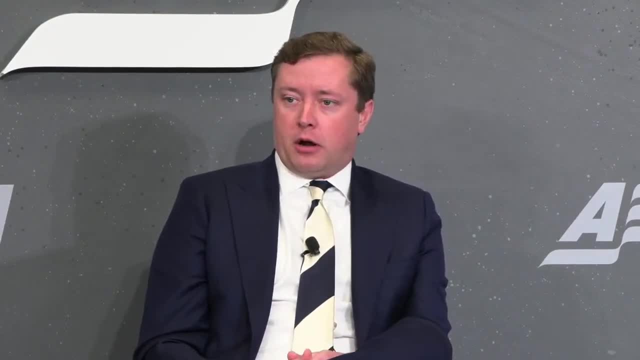 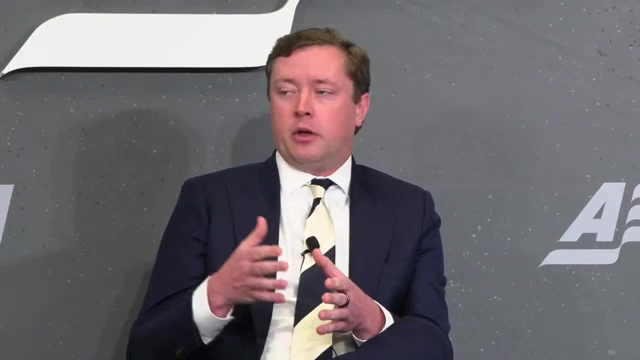 deployed today. So I think one of the things that we're focused on and are very much trying to get involved in is to help regulators and lawmakers understand what the promise is, what this represents to patients, what it can represent to the cost curve in the healthcare system today. 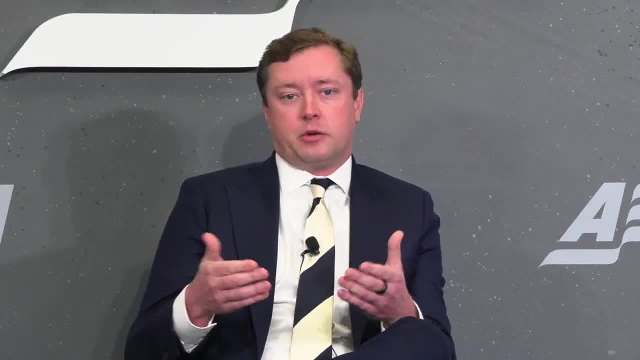 and how deployment of these technologies are going to help basically create a better future. Thank you, Thank you, Thank you very much. I think that's really important. I think that's a really important point, and I think that's a really important point too. 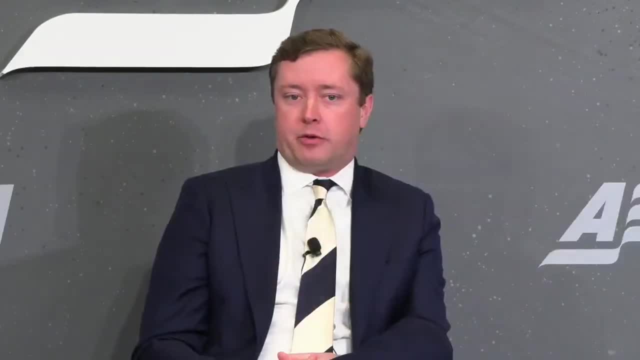 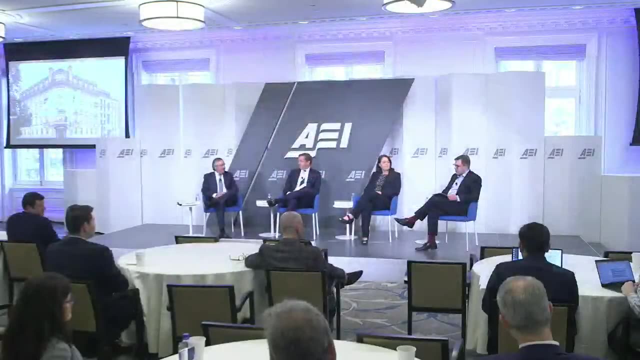 to see how we can actually create a system where caring for patients becomes more human and allows for patients to get direct care from their providers and allow for technology to provide more personalized care. So excited for the conversation and I appreciate the opportunity. Thank you for joining. and I would say it's replacement of components of clinical staff. to allow them to then do other things like the average. if a primary care physician did all the tasks they were supposed to do, they do the study every couple of years showing what their day would look like, And so the average primary care physician is supposed to do all the tasks they were. 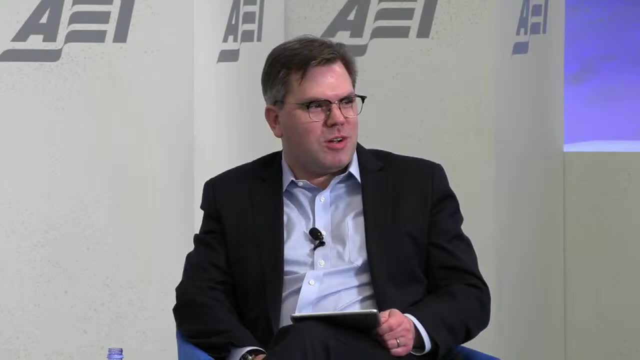 supposed to do, And so the average primary care physician is supposed to do all the tasks they were supposed to do, And so the average primary care doc would have a 27-hour workday. And so my answer to that is: thank God for technology. 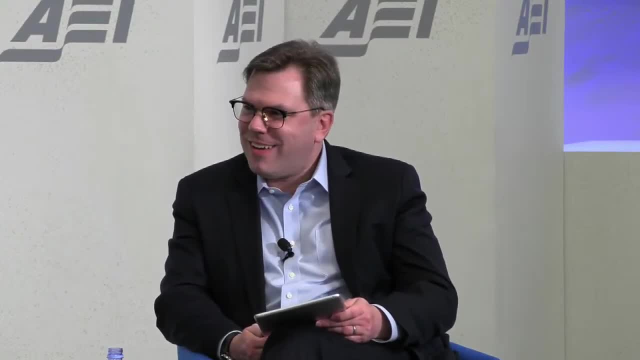 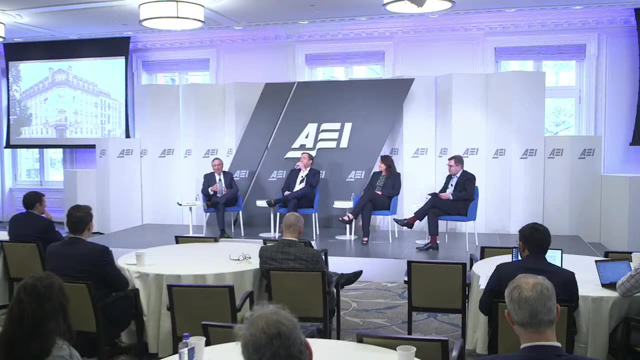 Mark Brian, thanks, Good to be with you, and all of you as well. Mark Leahy, I've had the pleasure of running the Medical Device Manufacturers Association for over 20 years. We represent about 300.. Start off primarily small, mid-sized venture-backed companies, but we do work with some of the 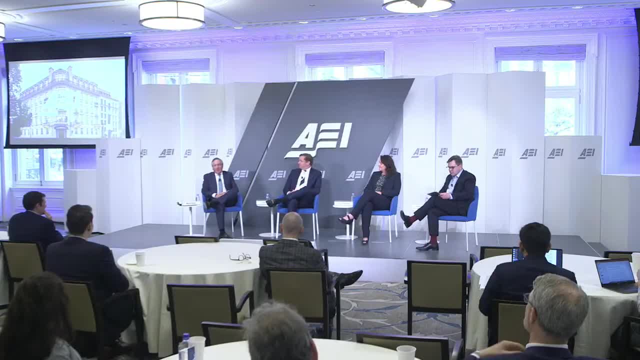 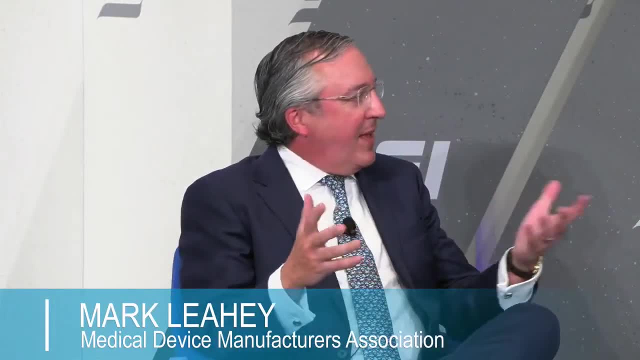 larger companies and our mission is to provide timely access to safe and effective products for patients. Colin, you were saying that you've been involved. You know your firm's been involved in investing in the thesis in AI for the last 10-plus years. 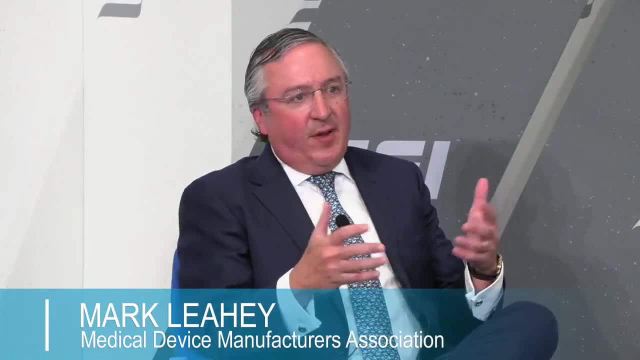 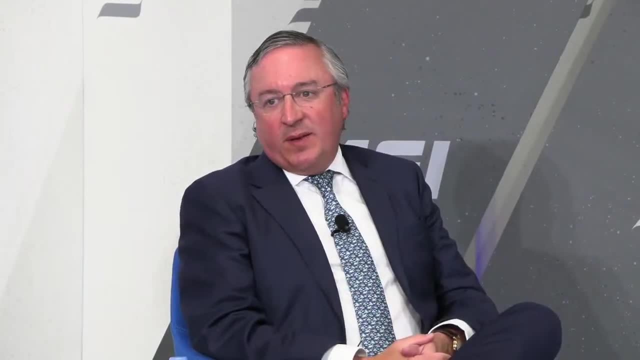 And I think it's important to level set here. for medical devices, CDRH authorized the first medical device with AI back in 1995.. So this is not a new story in devices as well, And in fact today there are over 700 medical technologies that the FDA has authorized with an AI component to it or software as a medical device. 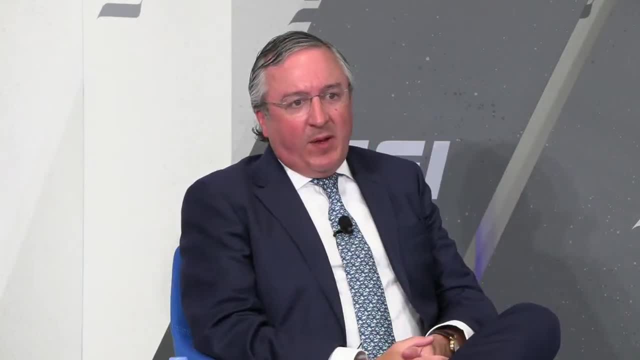 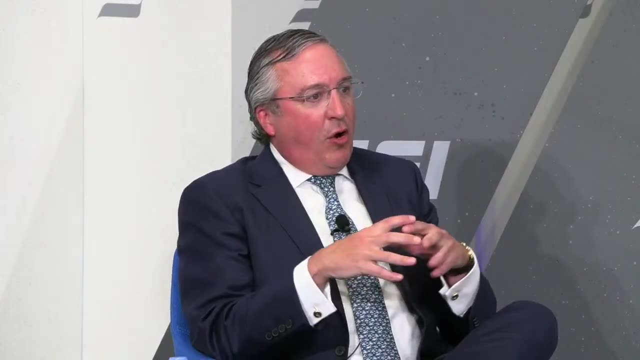 There's software in a medical device too, so there's some nuances there. But I think you know we share, you know we've seen the impact it's had for diagnostics, for monitoring. a great opportunity I think our overarching kind of lens here is do no harm. 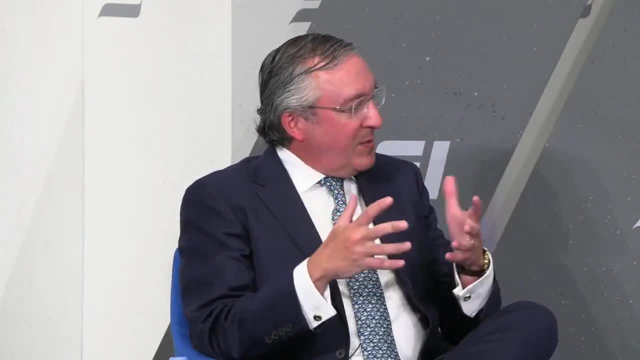 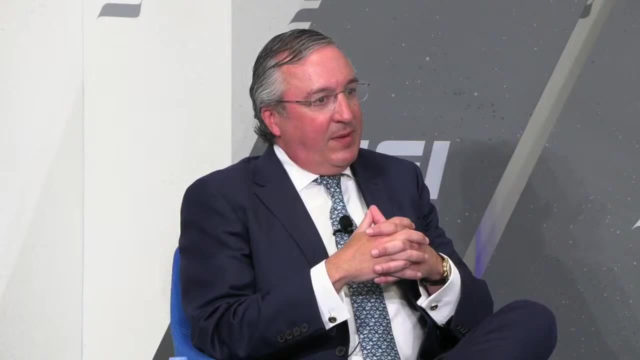 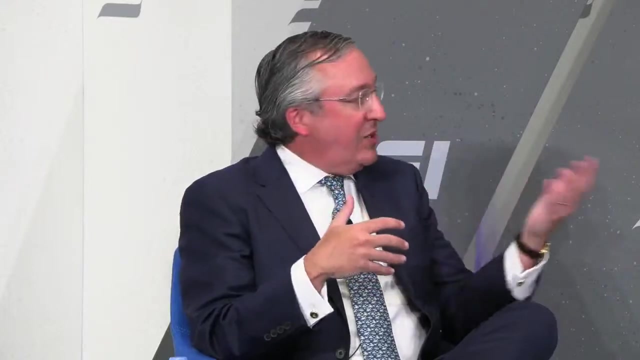 You know we've had a good- not perfect- at the FDA, but we'll get into some of the specifics where it's kind of worked well. There are a lot of other federal agencies now who are interested in the government about AI And I think kind of as a core tenant here we don't want to see things that are layered on top that would run in conflict or could slow that patient access to these. 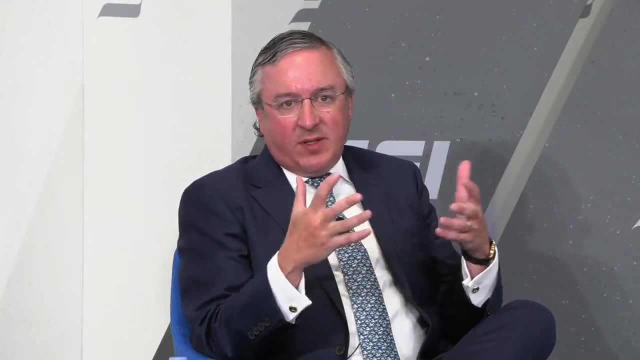 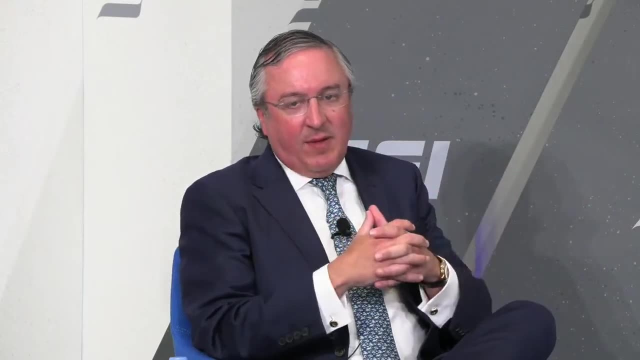 And I think it's also important to take a risk-based approach. You know that's what CDRH does You benefit. It's not the theoretical risks, It's the probable benefits. outweigh the probable risks and keep that as kind of the focus. 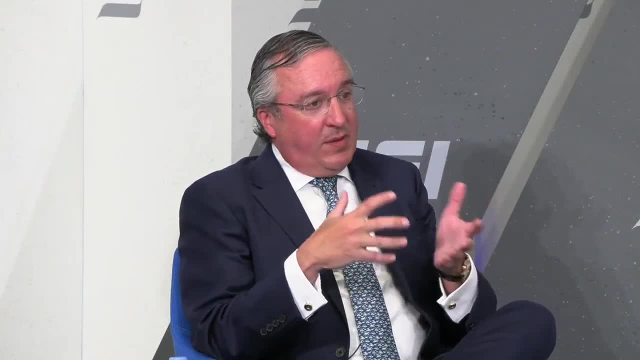 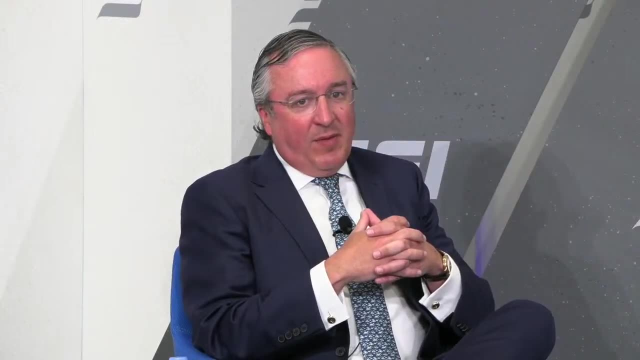 And again I think to FDA's credit, there's some tools in Congress as well that they've tried to move forward to provide some flexibilities, But certainly more is needed And on the overall value perspective, I think that's the other piece where it's one component is to have that well-worn or clarity on the regulatory pathway. 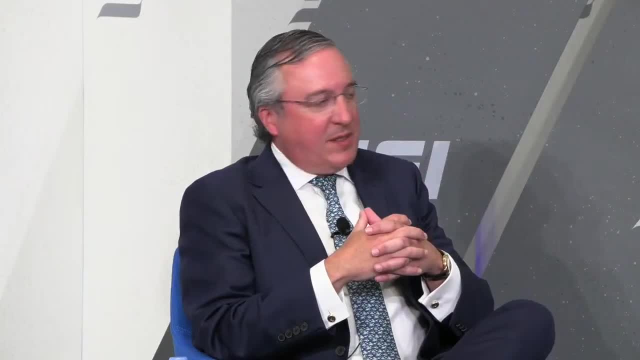 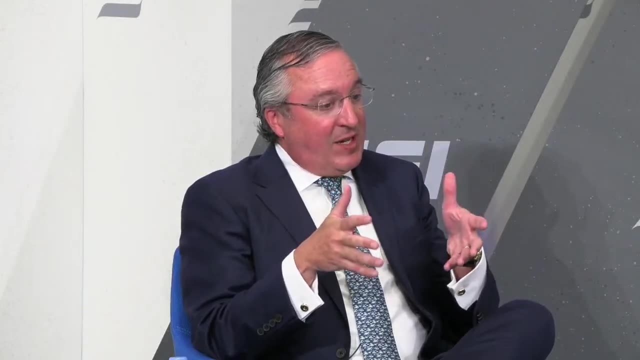 But if these technologies aren't valued appropriately in the health care system, that's going to impact investment and adoption. So a lot to chew on here, but great, great potential and not even potential. great impact today, but certainly more on the horizon and happy to be here. 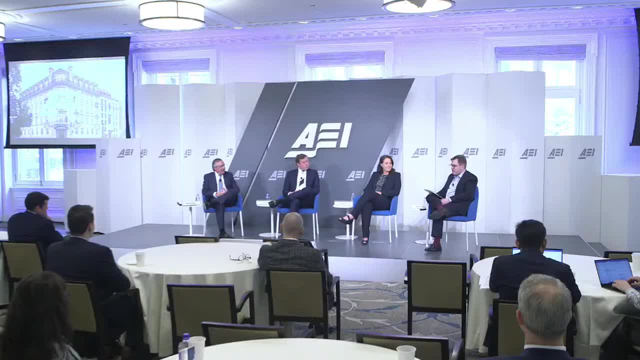 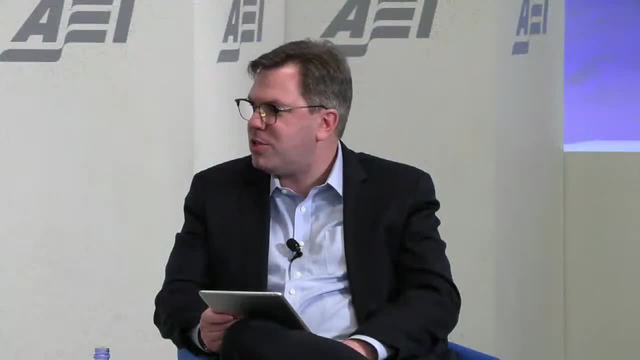 Thank you And Jane, a question for you. You've argued that many AI applications that we have, or the development of those products, is a form of free speech and that the government might be constraining or regulating Free speech by regulating that software. 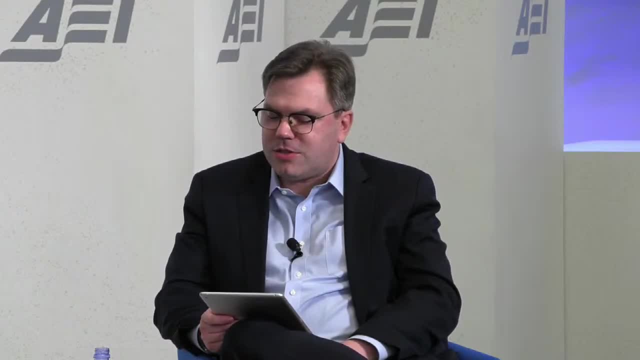 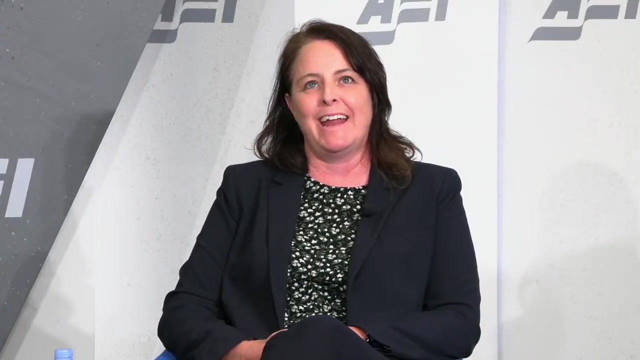 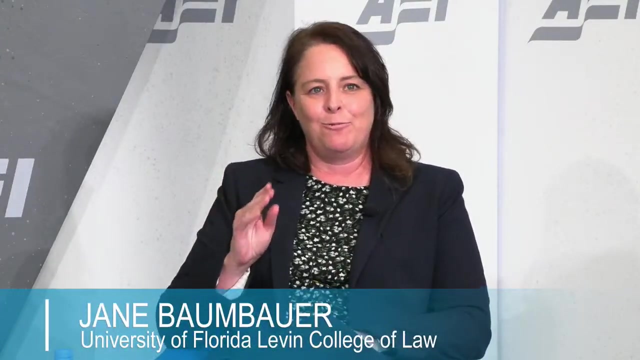 How do you think that free speech law is going to intersect with the regulation of medical AI at the FDA? Yeah, so I set up some of this in my intro remarks, which probably went a little long, but but maybe it would help to explain how I came to be talking about health technology at all, which was my experience. came through a few, a few really salient examples. 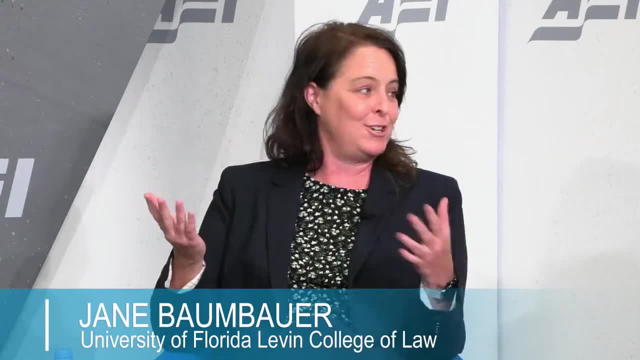 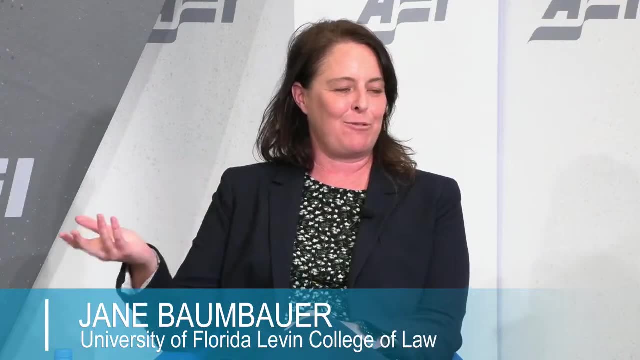 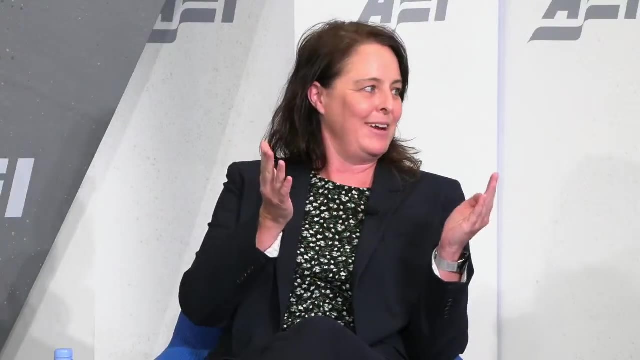 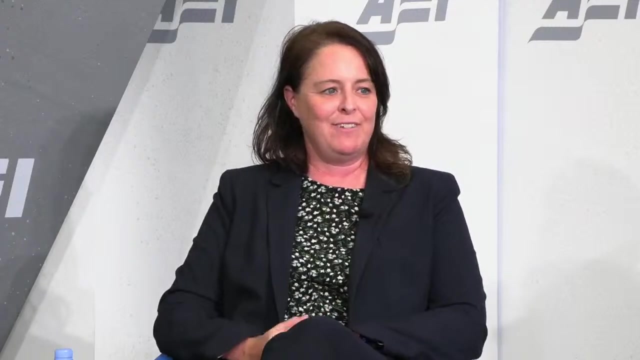 One was 23.. And me, where I had all as a, as a consumer, I had already done my kit- and and 23 and me was was in the process of providing feedback on genome wide association studies. So they were basically just linking my you know genome to genome sequencing, to known GWAS and then and then providing feedback. 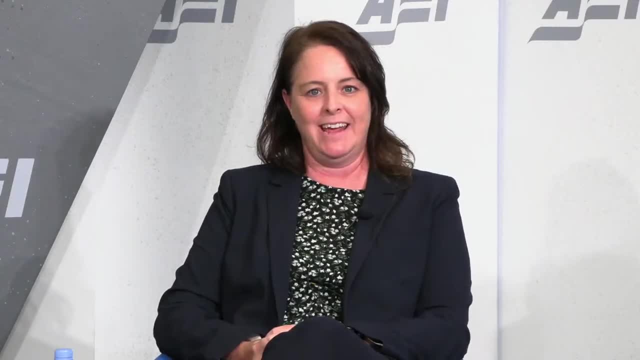 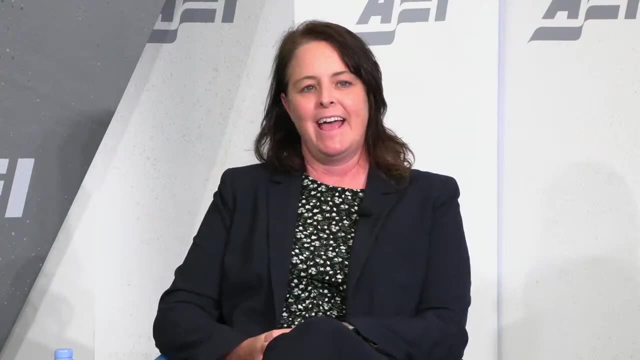 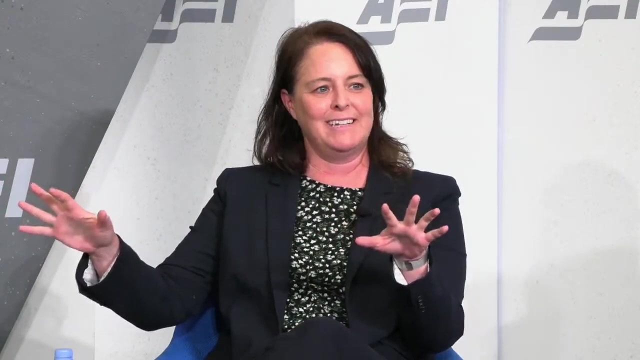 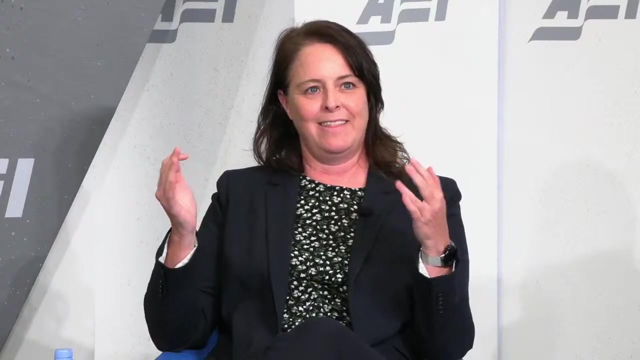 And that, of course, got interrupted by FDA, by an FDA letter, And and, And, And. since then, 23 and me has been going through the clearance process, and so that got me thinking. well, this is strange, because information already exists, you know, in two places. and then, by connecting the two sources of information and telling me what I could learn about myself, that made an other- otherwise, you know- consumer product turn into a medical device. 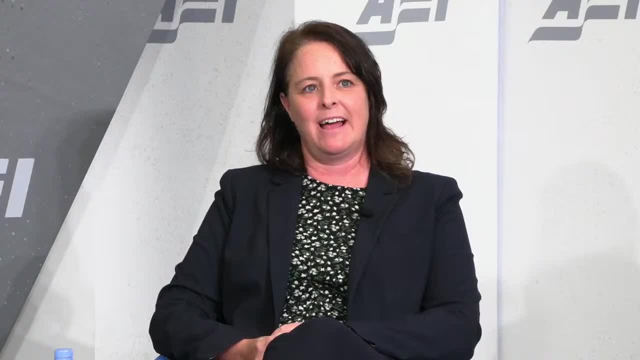 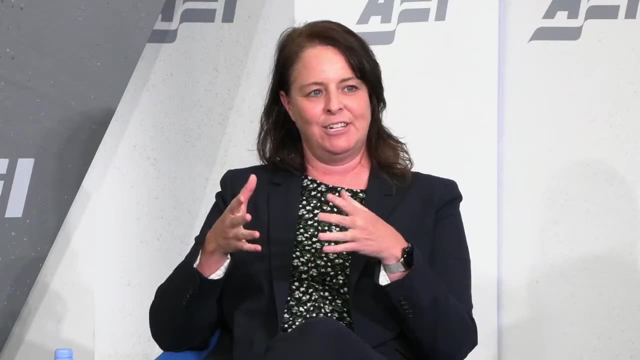 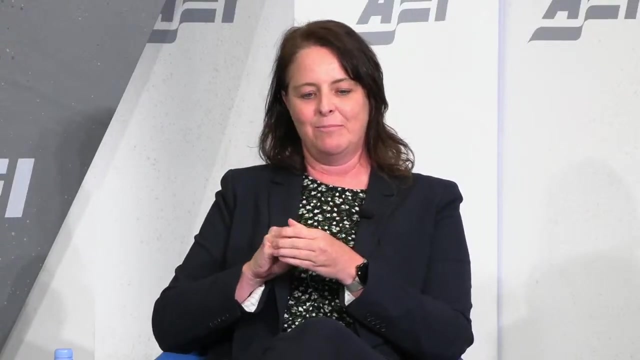 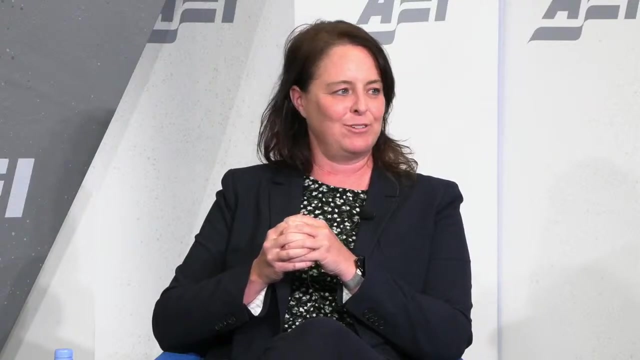 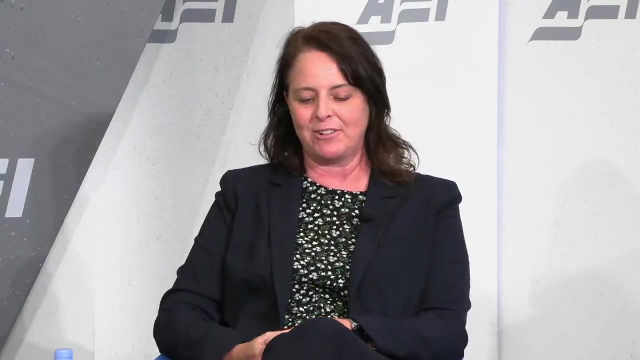 And so so it's interesting, I think, That the gateway into becoming a drug or device has to do with, first of all, how you market it, so that in itself is kind of a very speech salient point of time, and then also that any device that attempts to give actual diagnostic information well, and then it needs to be giving it diagnostic information or some sort of medical information. 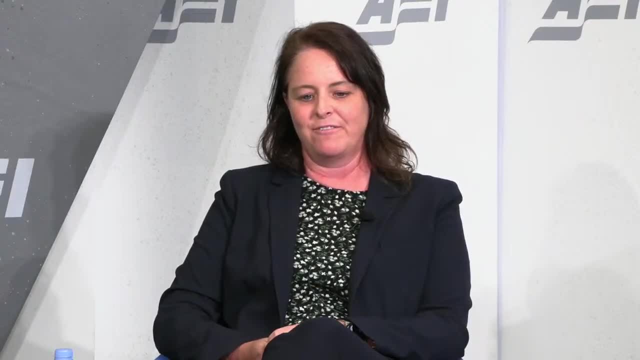 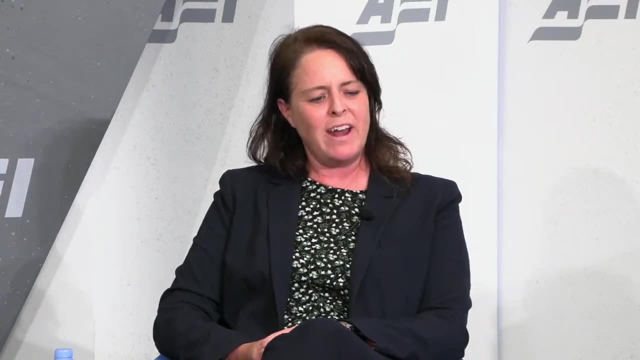 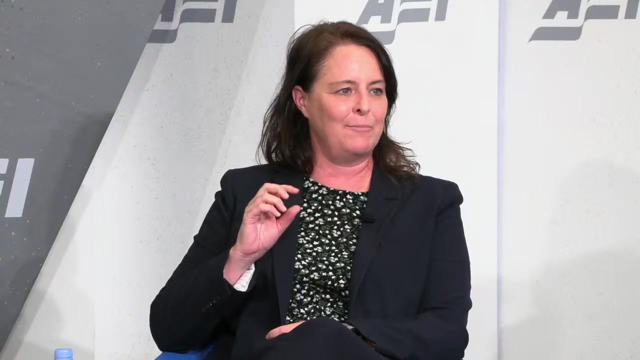 So then then another example came, in the form Of a mole doctor or mole detector- I'm forgetting what the name. now It was an app, though, that was not as good at at detecting carcinoma as as, as a, as a dermatologist, but better than a primary care physician. 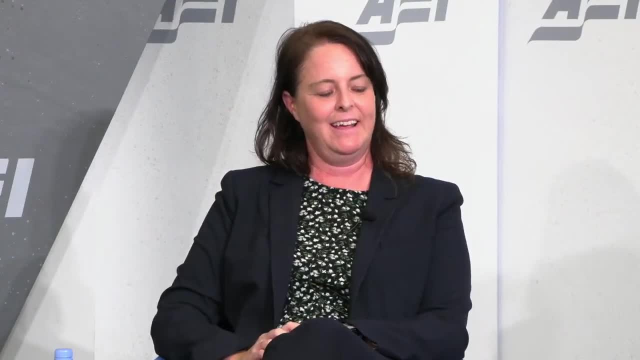 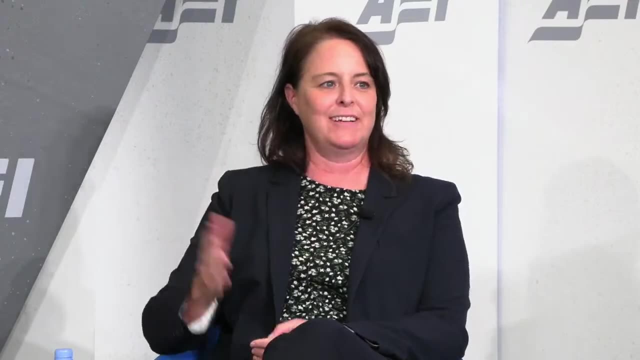 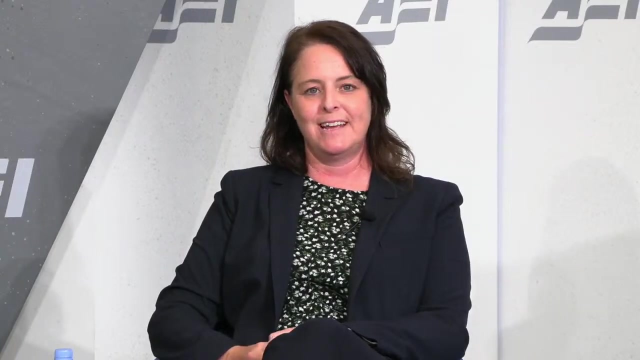 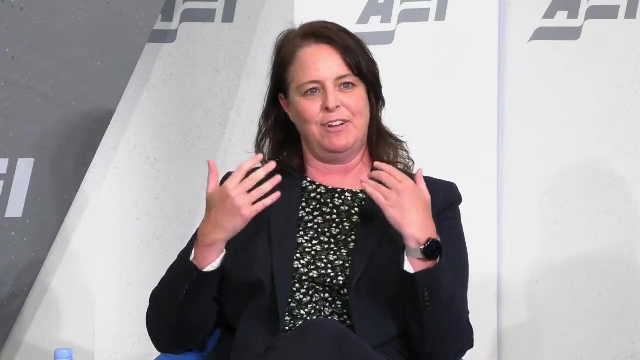 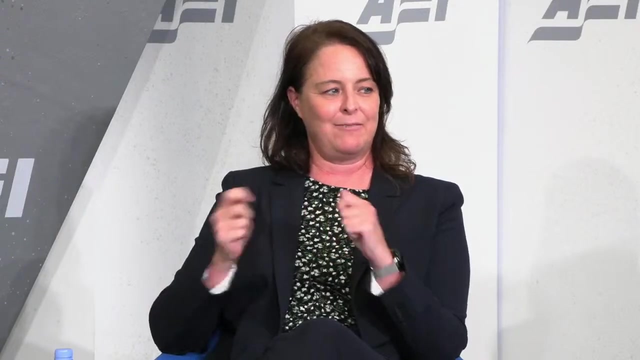 So so, but the FTC- FTC, not the FDA- went after the app for marketing itself As something that's useful for the purpose of self diagnosing your, your moles, because it had not. you know, it was insufficiently substantiated And this too seemed to me to be very strange, again from a First Amendment perspective, that the risks actually seem quite low, because we think that the proper comparison is to somebody who maybe goes to a primary care physician. 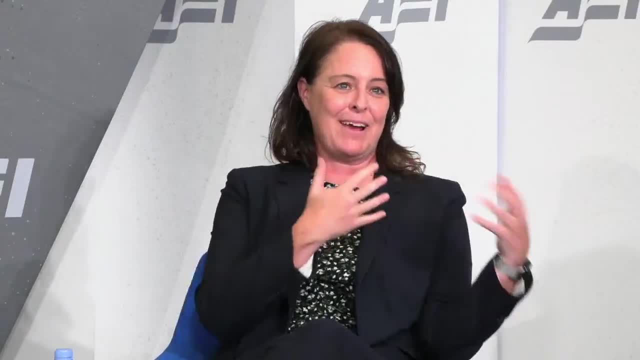 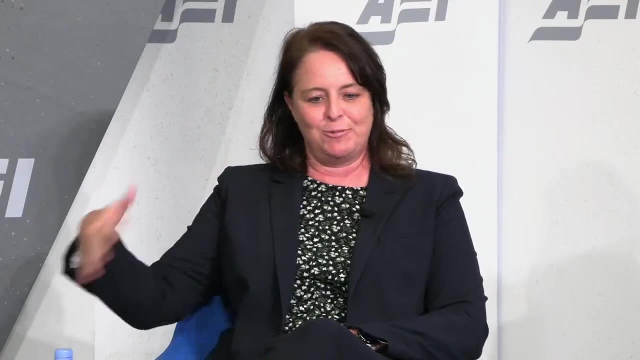 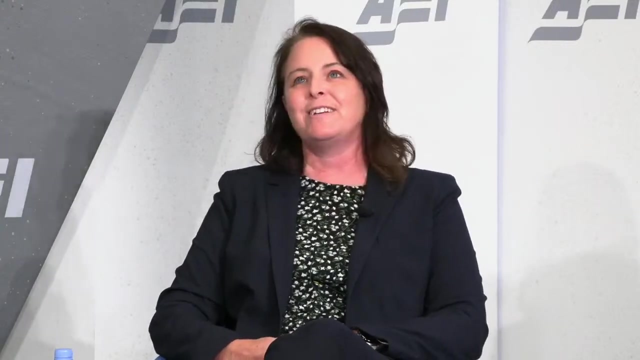 Maybe doesn't go to any physician at all, right, So compare the outcomes To that patient to to what life is like. you know the distribution of outcomes for for someone who has access to the, to the app, And then I don't read. the third example, though, is Google. 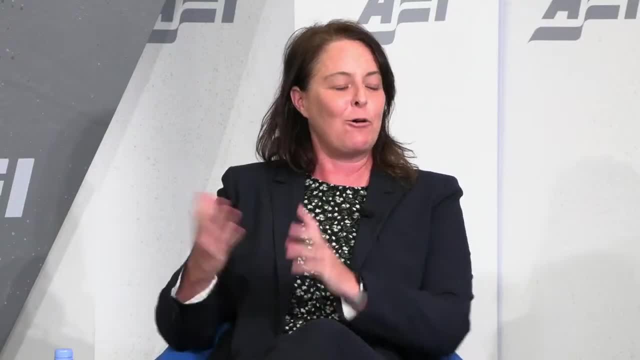 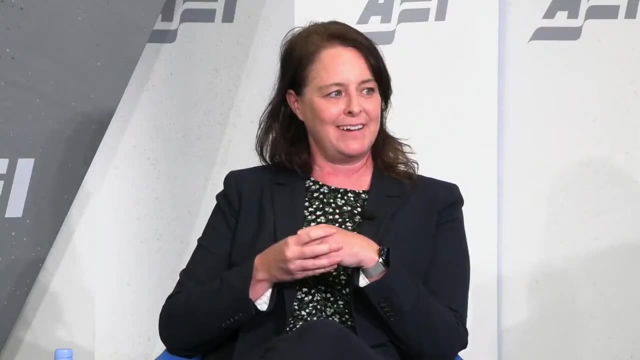 So everyone Googles their symptoms to try to get a diagnosis. And the only reason that Google isn't a medical device- or at least the Google search bar, I should say, isn't a medical device- is because it doesn't market itself as it it knows. 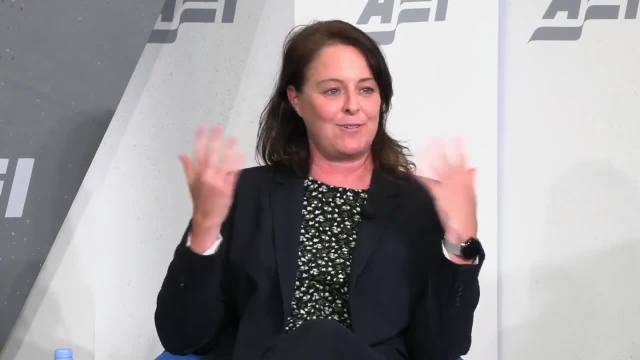 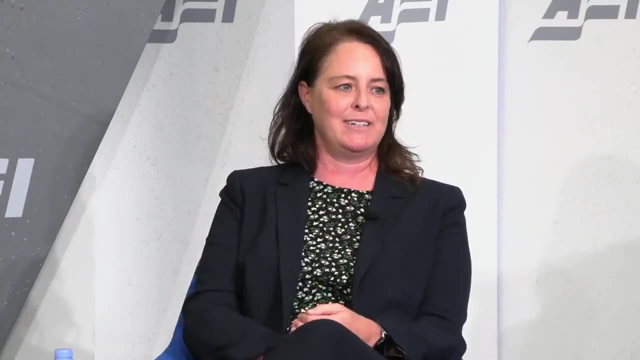 Of course it knows that people are Googling, They're symptoms, It even keeps track of flu trends and whatnot. But everything about the regular, you know the regulatory apparatus only applies once there's marketing. So I see speech in two dimensions here. 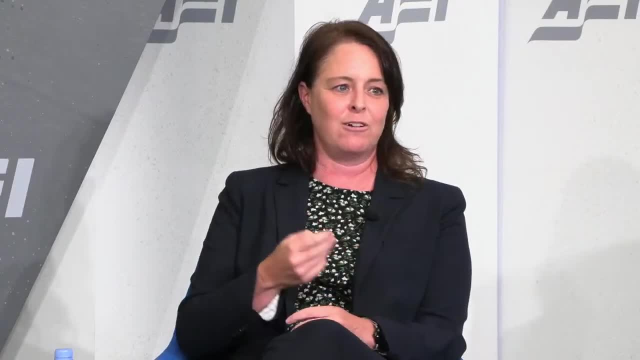 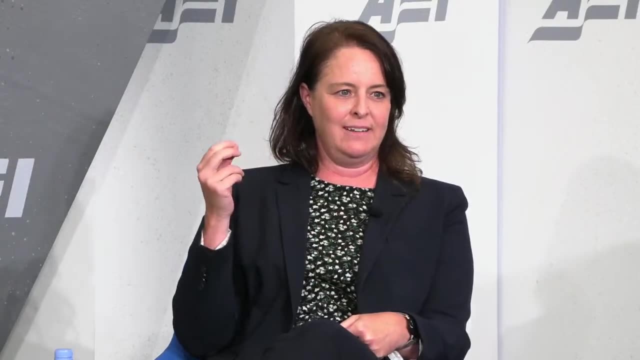 One is The output itself is not a physical force. By the way, I do want to contrast that with some ai that might be actually, you know, making decisions and then doing some sort of control- a laser, or or physically sending a laser attack. 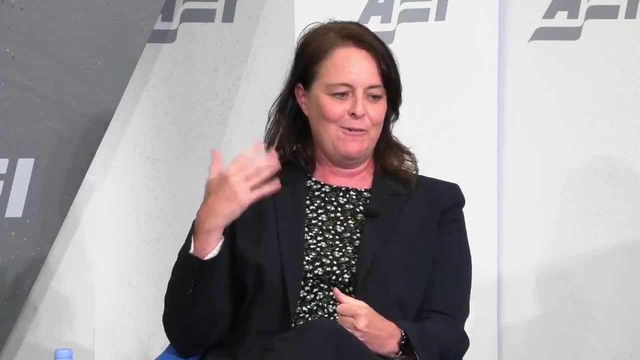 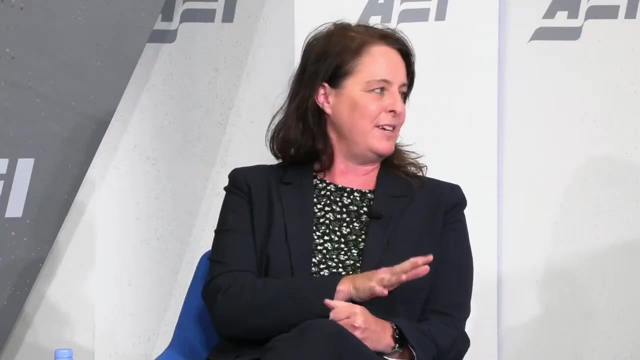 So it's, it's a, it's a total control. You know, I, I, I I've had, I've had, I've had electric pulse or something. Those I think could safely be understood as non-speech products or speech and conduct or something. 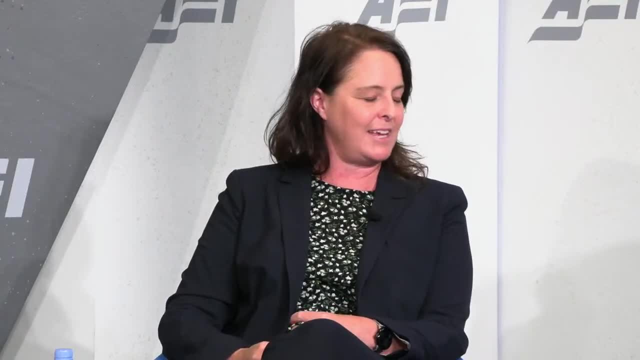 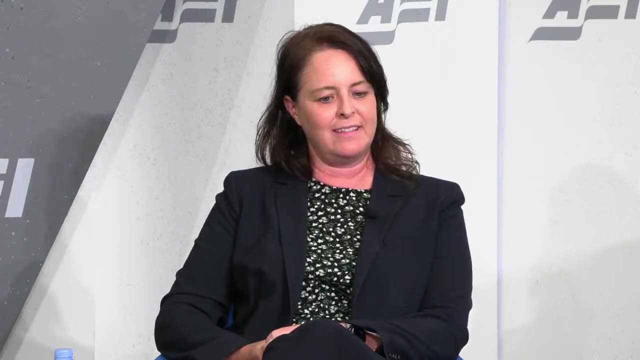 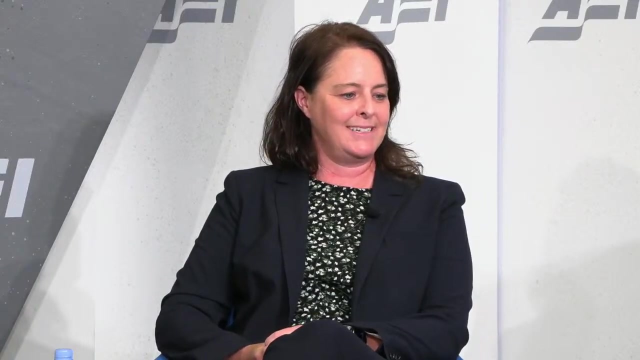 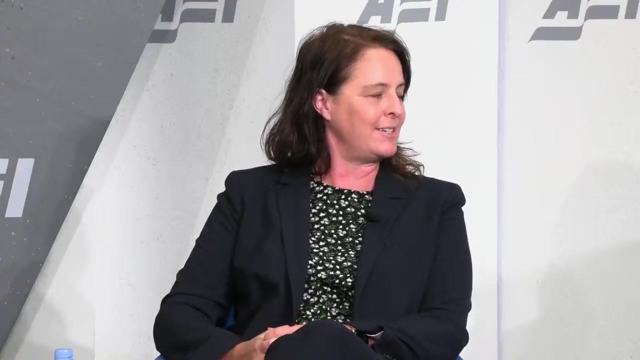 But for information output apps it seems really obvious to me that there is First Amendment coverage and the FDA. you know the FDA has gotten into First Amendment trouble before many times And I think it will happen again if they don't recognize the First Amendment limits. 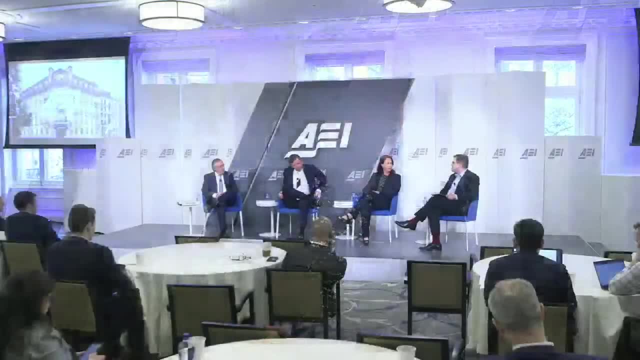 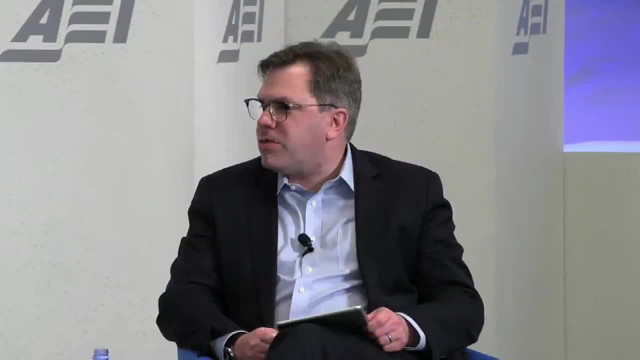 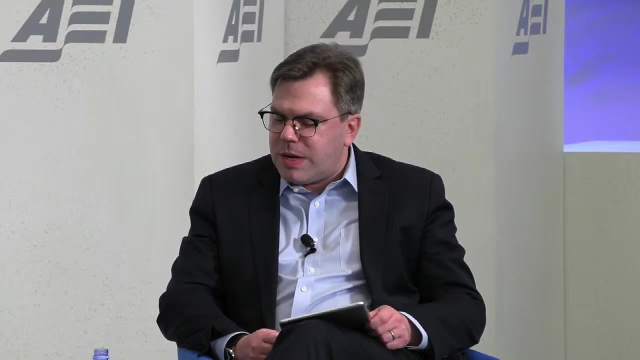 on this area, So it sounds like FDA's attempting to expand its authority. from your perspective, I guess the question is is: how would we reconcile this with the current FDA device regulatory framework as applied to software and its risk-based, the risk-based regulatory framework? 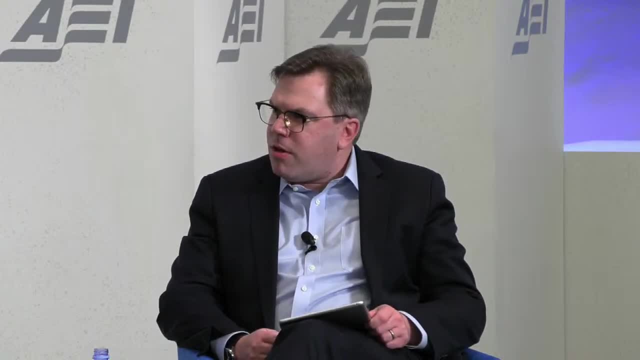 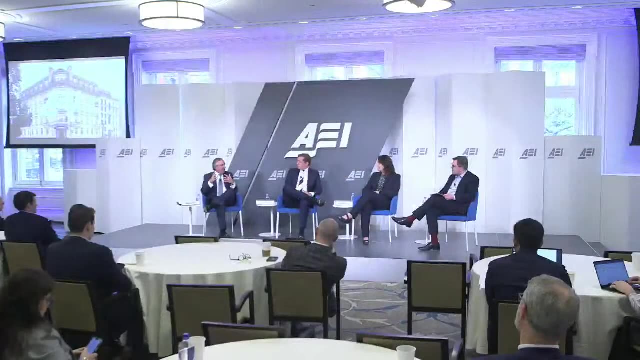 that CDRH uses for devices. Mark Colin, I didn't know if you had any thoughts along those lines. Right, I mean, there is a. you know, this is an area where people have been trying to grapple with what the software that's used in monitoring. 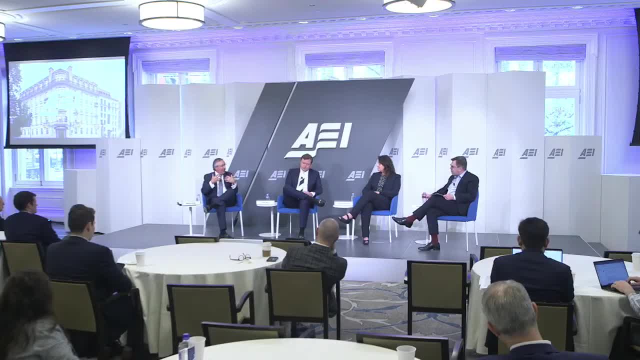 that's just kind of a wellness play, which is just kind of informing the patient, versus something that needs to have greater accuracy for, you know, determining diagnosis or pathway forward. You know, I think, with all due respect, to simply say all right. 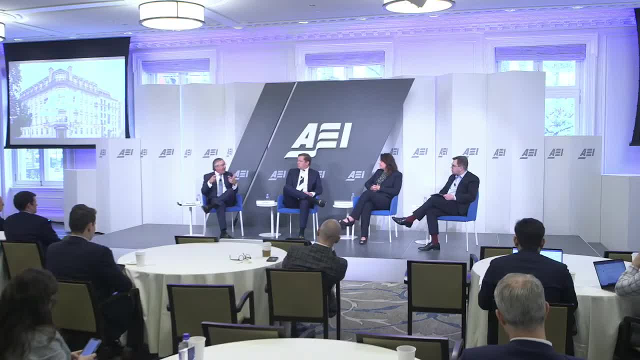 It's the First Amendment. I mean diagnostic. you know the accuracy matters here And I think you know we certainly wouldn't want to say, all right, nothing gets looked at, because it's all speech that's out there. 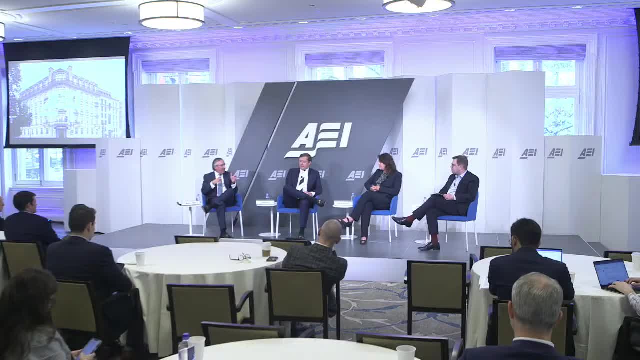 It's reformulating it, Because if something's not accurate, then we certainly don't want people to rely on that for the purposes of clinical decision-making. If it's you know how many steps they're taking or other things, and it's truly just for. 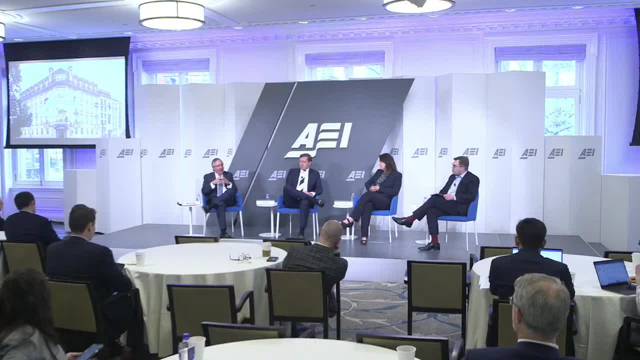 so I think there's. there has been a lot of effort to try to draw that line And I think on the the far ends, it's easy to ascertain: all right, this is in scope, this is out of scope. There are some areas in the middle. 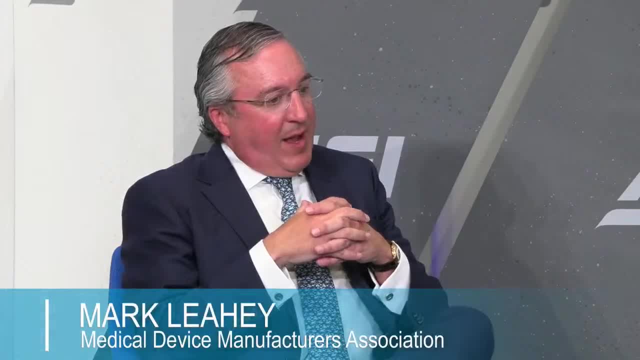 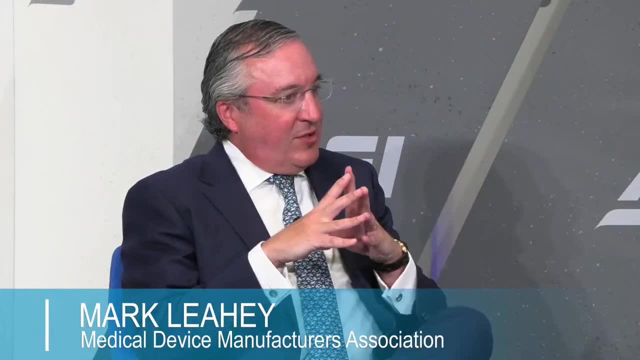 You know, I think when it comes to physicians and others, clearly around staffing and OR throughput, there's a ton of administrative efficiencies that can be leveraged here. that should fall way outside of FDA's purview. here, I think there's a huge opportunity. 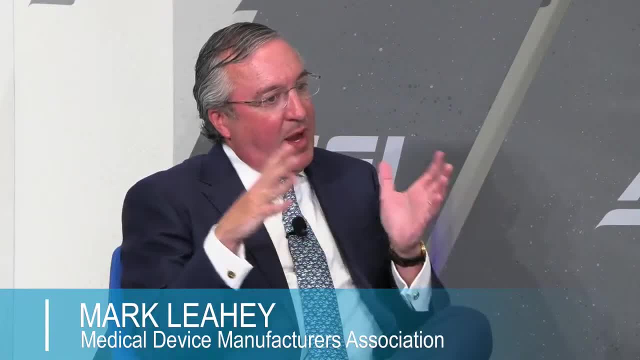 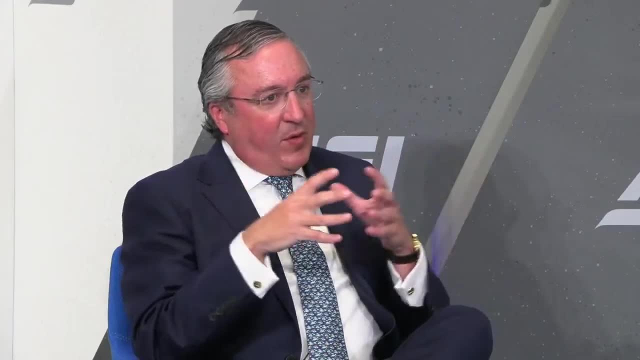 to drive costs out of the system through technology. I think when you migrate into the you know the more the devices that go into diagnosing, to monitoring I think most you know folks would want to ensure that they're safe and effective. 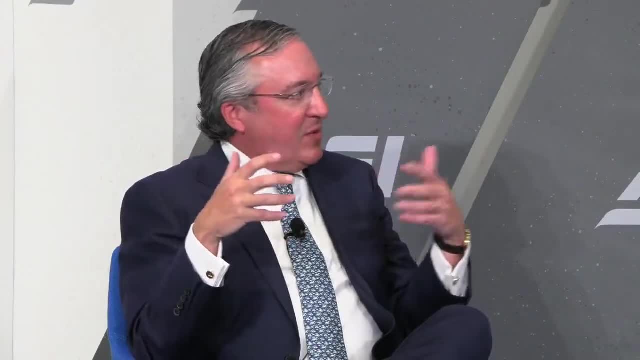 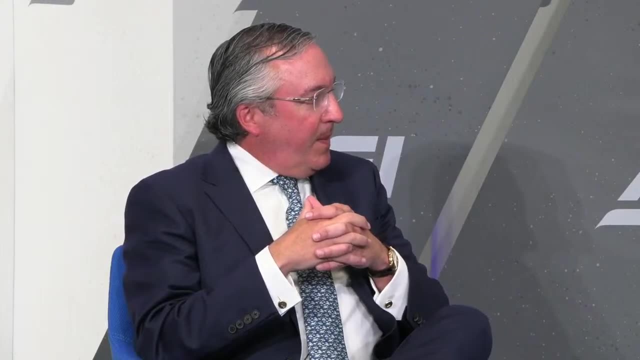 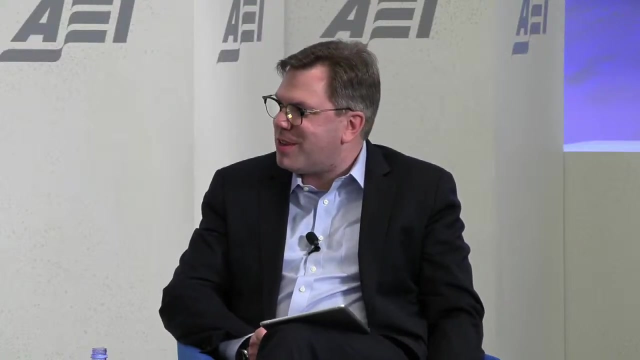 with the right regulatory touch, not adding time so that it gums things up and patients are being delayed access. So it's just that nuanced approach. So you know, something like automated surgery would obviously be a very high-risk device, Thinking about the movie Prometheus, for example. 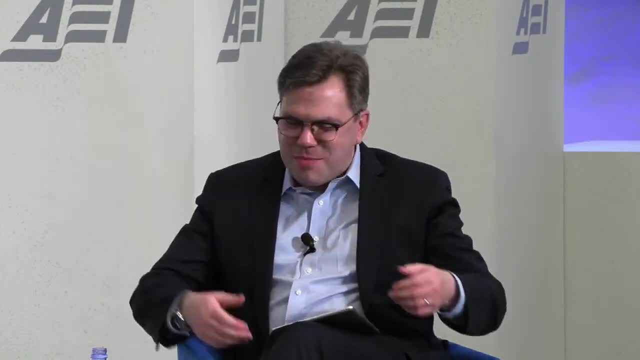 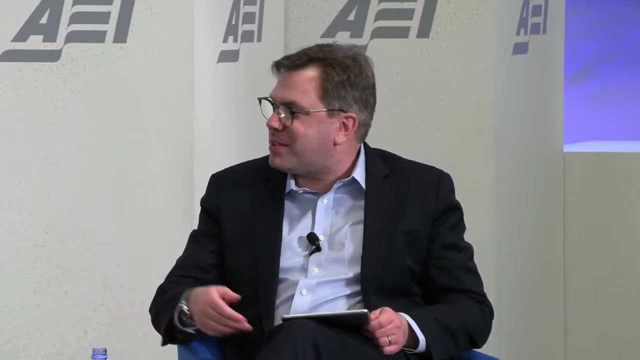 with the automated surgical bay that does the CT scan and then operates on you. you know that's probably 25 years away, but that's clearly a high-risk device Right now. it might not be high-risk in 25 years. Do you think that part of the problem is in looking? 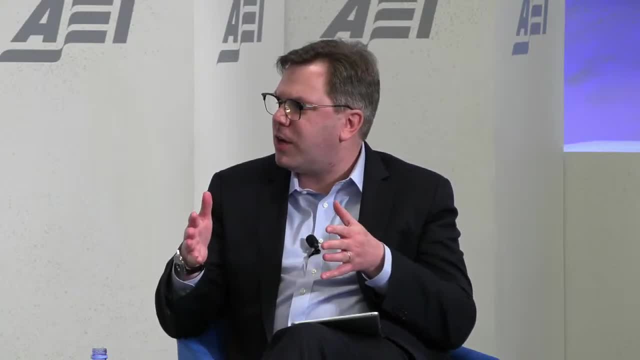 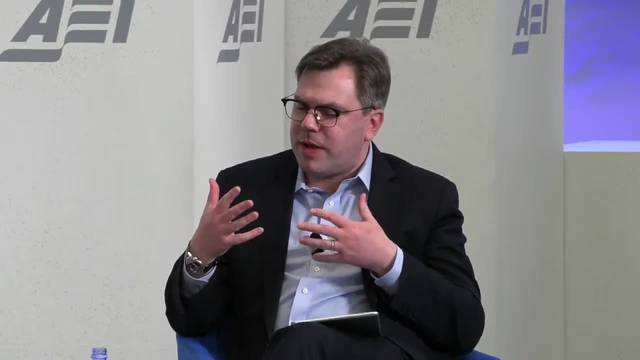 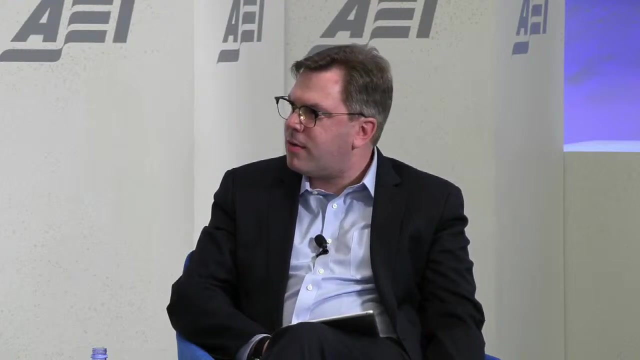 at what is a class one versus a class two device in the software and particularly AI context And, in answering that question, if you could provide some context for the audience about what those two categories mean and maybe the FDA's regulatory framework? Sure, So again there's a risk classification. 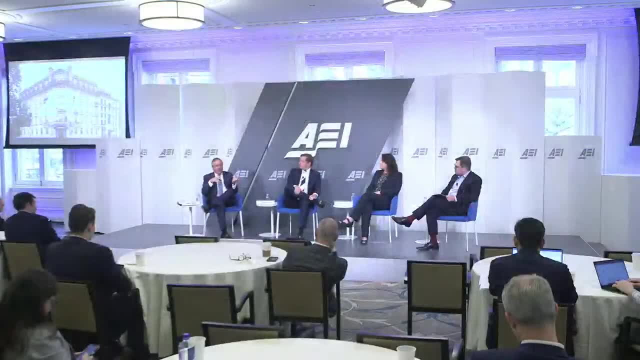 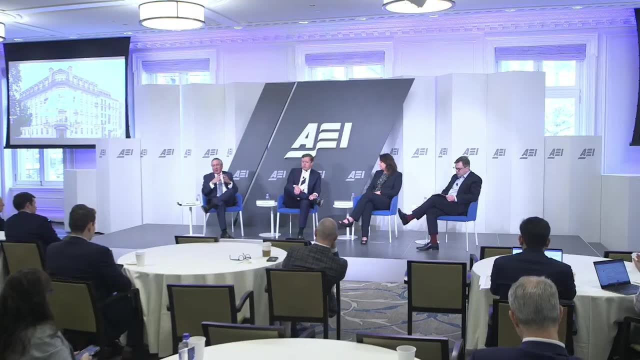 The FDA has class three, The higher risk. class one is the lower risk. class two It's kind of that middle and most fall in that class two area And there's varying levels. There are certain class one exempt products where you have to register with the FDA. 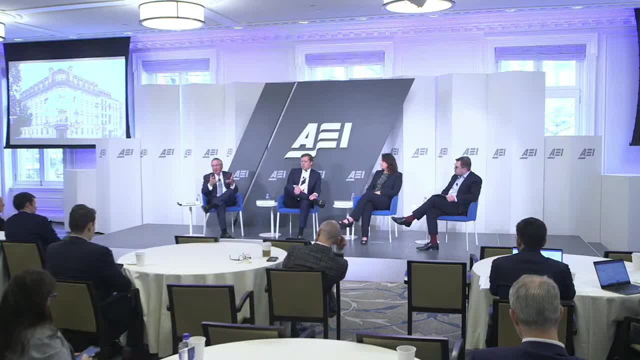 You have to have a quality system in place, But it doesn't require you to actually file a submission before you can bring those products to the market. On the class three in class two you do have to go to FDA and file that submission. 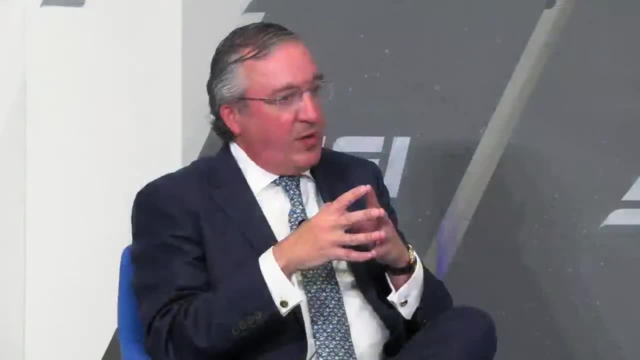 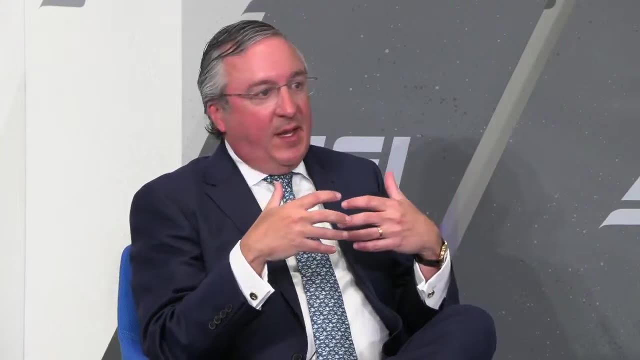 That could be kind of middle ground for some of these technologies as well, where you want to kind of have visibility as to who's doing this. So registration listing, You want to make sure they have a quality system in place And so aligning around those. 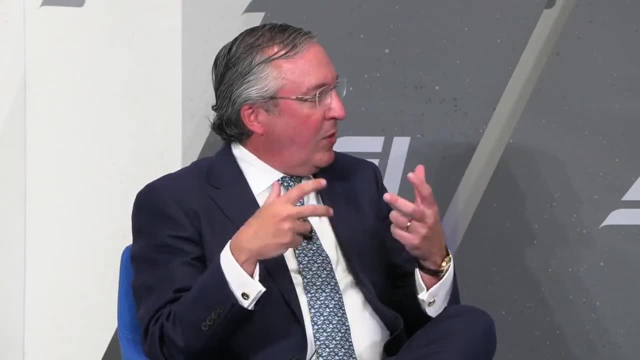 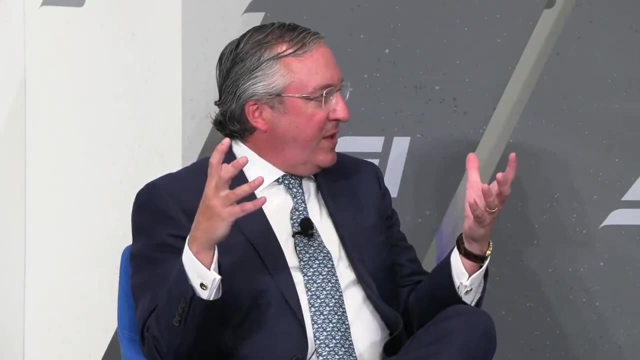 But if they're not kind of higher risk than a lighter regulatory touch, there are tools in the toolbox. So I think it really comes down to less about we need a whole new structure for this than how do we leverage the current tools in the most effective way. 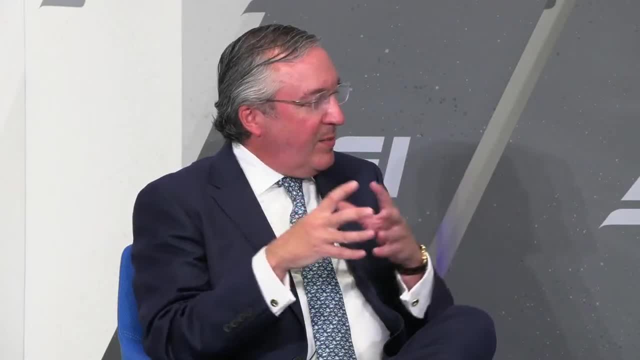 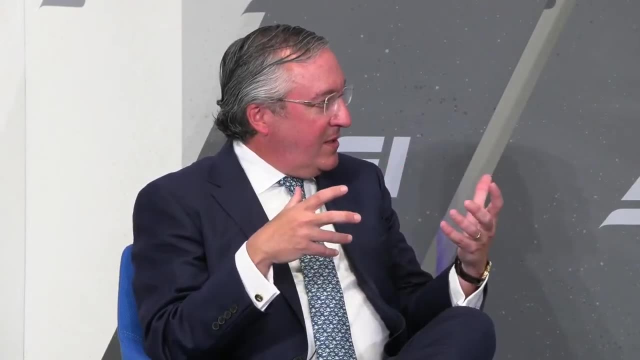 And again we'll get into the predetermined change control plans in a bit. But then on top of that are there targeted changes that, candidly, FDA was utilizing in onesies and twosies but felt if they wanted to adopt it more broadly. 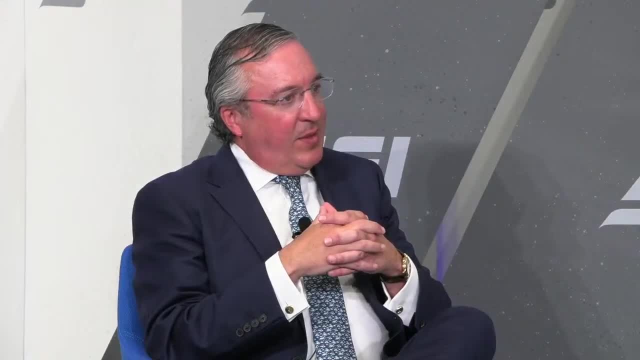 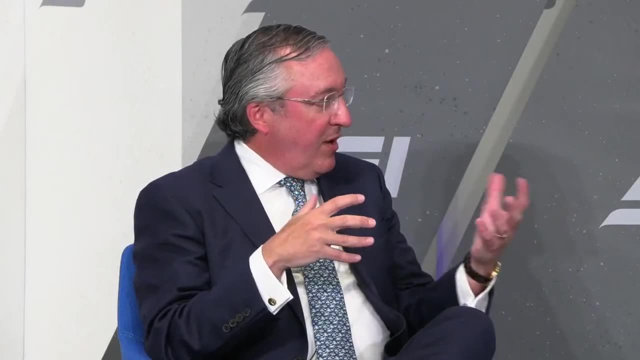 needed the congressional authorization to do so. So, long story short, there is a risk-based approach to how medical devices get through. It's supposed to be a least burdensome process as well, And so I think it's certainly appropriate. if there are folks out there who are suggesting that, listen. 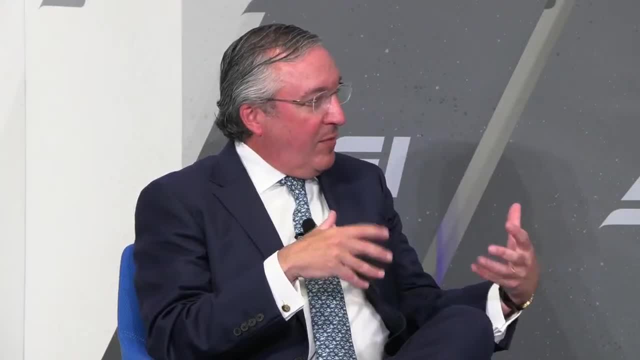 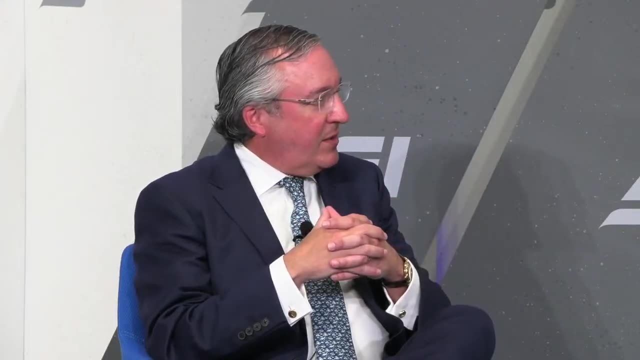 yes, we are a medical device, But it's on the lower end of the spectrum here. Maybe it could be characterized as kind of a class one, exempt Based upon the claims and other features of the technology. Yeah, and I think also that stamp of approval from FDA. 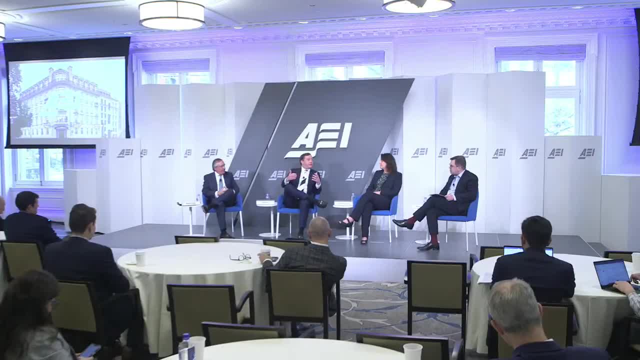 when you look at the startup community too, gives them an easier path to market And you have that stamp that allows providers, physicians and folks across the entire provider group sector to be able to comfortably feel like we can use this And it prevents that more difficult sales pitch. 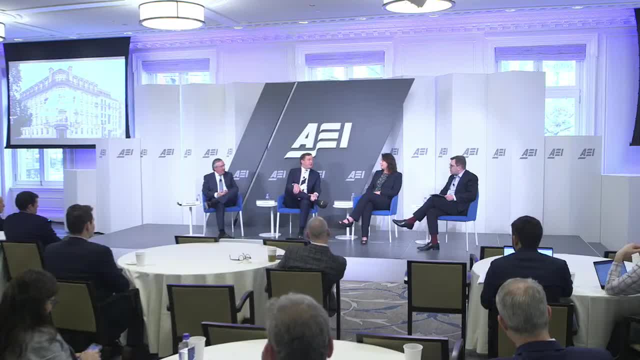 into some of the different provider groups in the hospital systems that may be less likely or a little bit more skeptical of the technology. So I think a lot of times effectively navigating that risk evaluation or mitigation strategy oftentimes allows technologies like the ones in our portfolio. 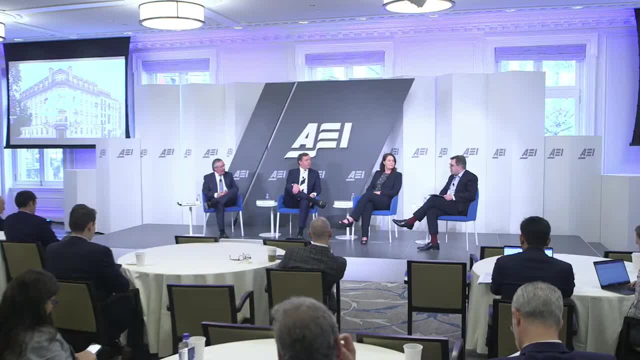 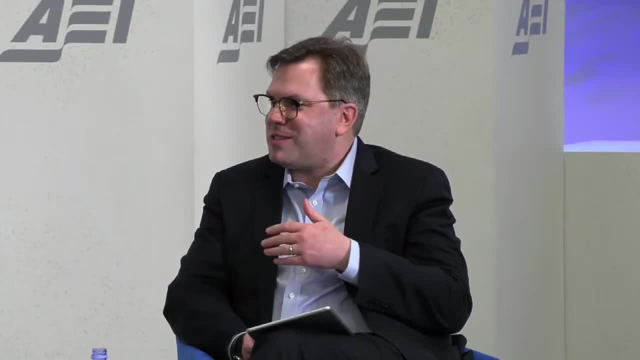 to more quickly navigate the market share. So one of the things that Mark mentioned which I wanted to ask you about is about conflicting regulatory structures across agencies, That we don't want to have agencies pile on top of each other so that technology innovators have to go. 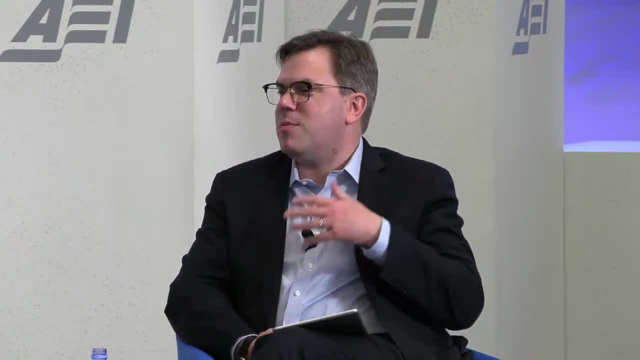 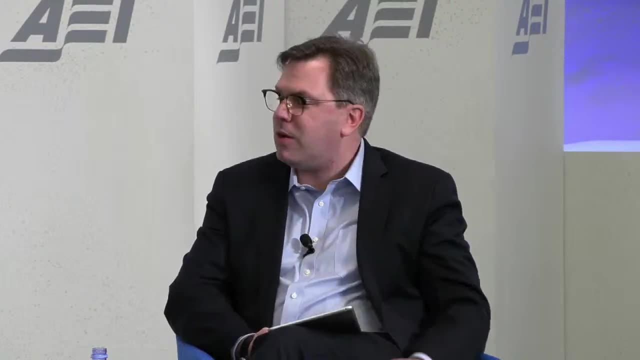 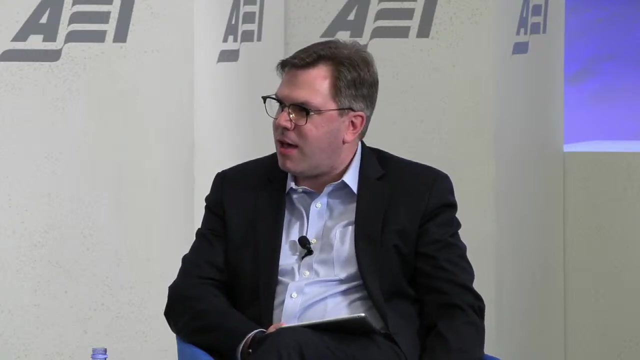 through three or four different agencies to get to market and then get payment And then finally it ends up in the hands of the consumer or the doctor or the hospital or the health plan or whomever. What do you think about the recent ONC rules around AI? 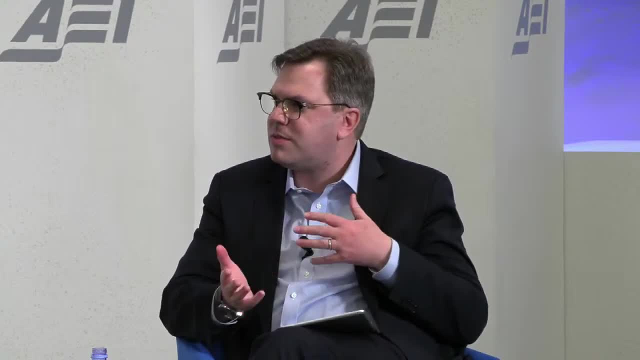 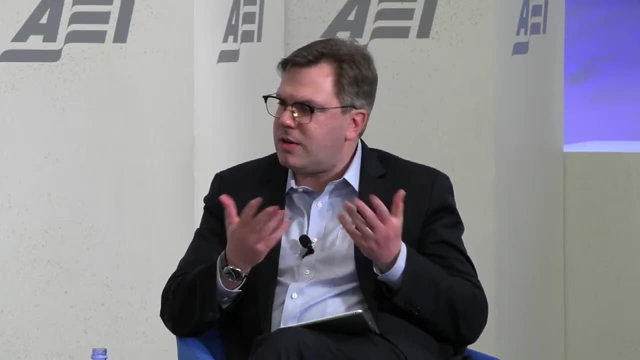 And do you think that those are producing conflict with the FDA? Are these agencies fighting each other for regulatory jurisdiction? I know that there's been a lot of talk about assurance labs. What are your thoughts? MARK ZUCKERBERG- Yeah, 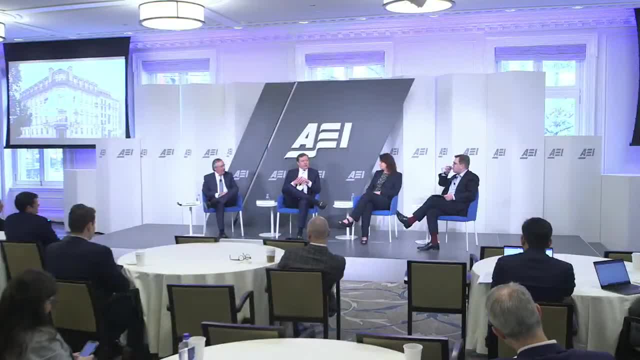 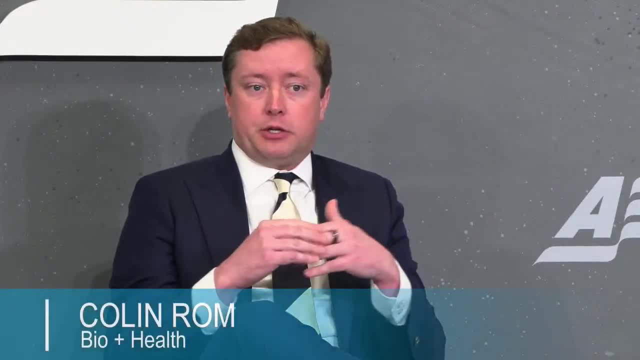 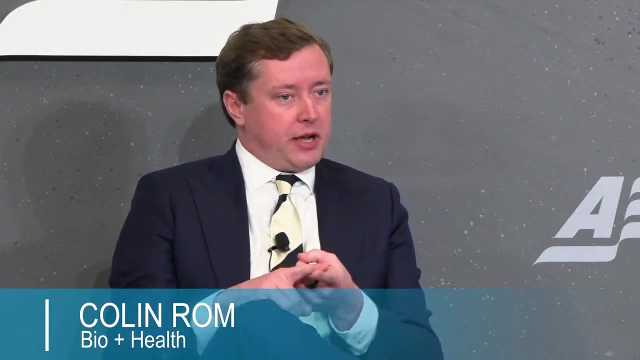 Assurance labs have largely been the biggest issue over the last year or so that we've been tracking really heavily. I think the idea of leveraging third party expertise is a huge opportunity for regulators and the companies that are innovating in this space to basically move through the process more efficiently. 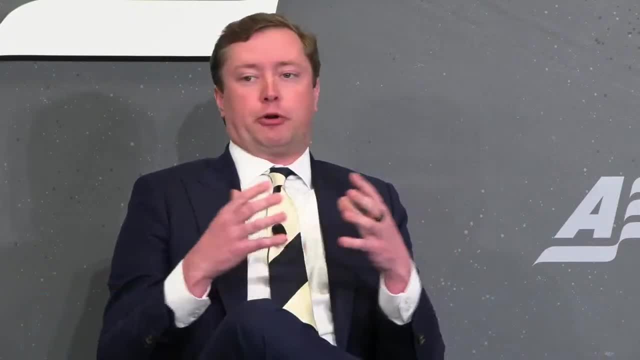 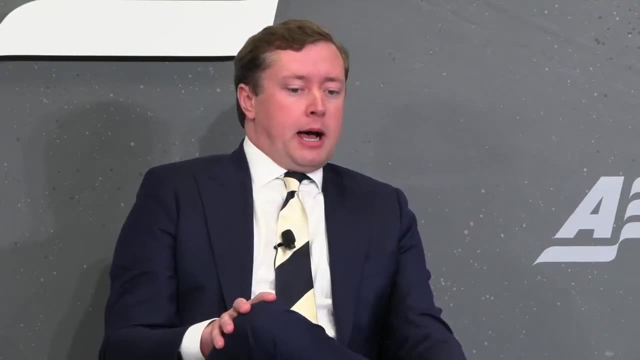 make it faster and not have to go through the entire process of basically recruiting new folks at FDA and new areas of expertise and what comes with the user fee process when it comes to that. But We're very supportive of the broader idea of assurance labs. 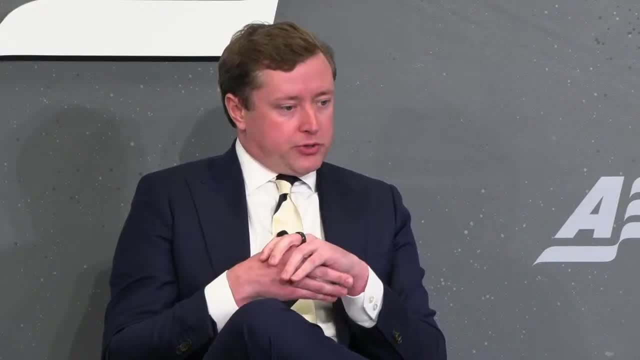 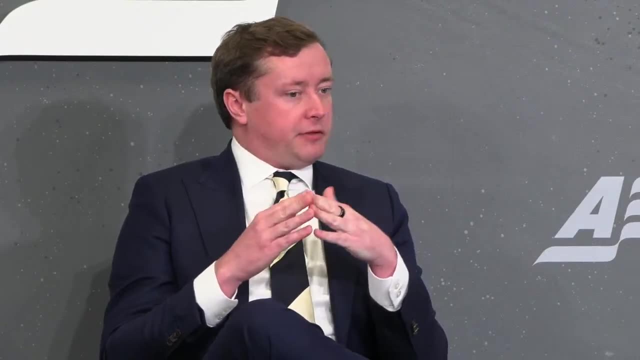 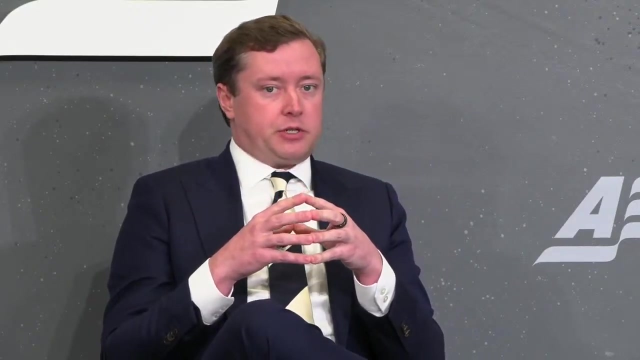 The concern that we have is the broader proposal and organization that has been getting a lot of support from regulators at the White House, from ONC, FDA, CMS would largely put a handful of legacy tech companies coupled with a handful of large hospital systems. 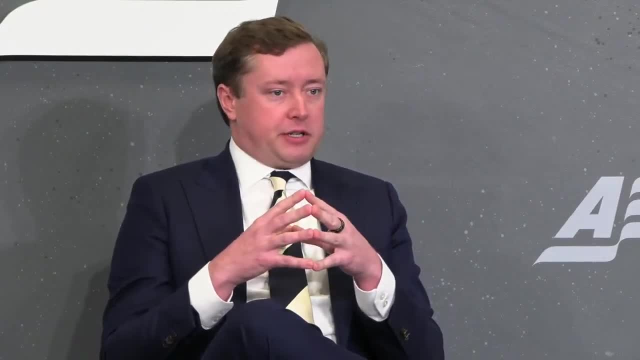 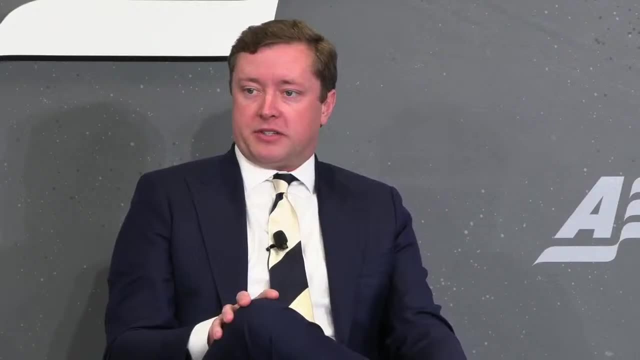 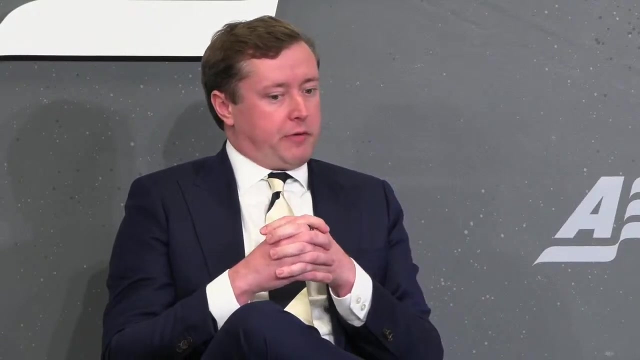 in control of validating the safety, efficacy, risk mitigation and bias alleviation of innovators or startups like the ones that we invest in every day, And I think this largely constitutes something that could potentially be a significant conflict of interest in terms of what that process looks like. 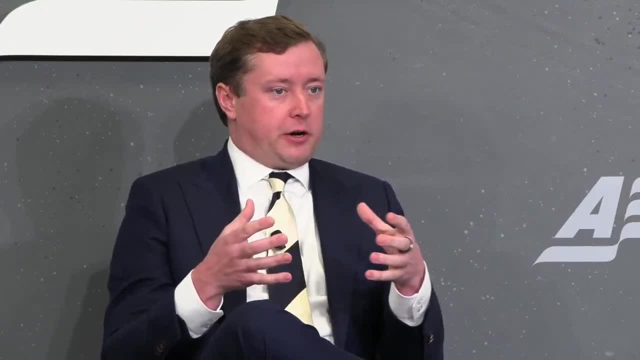 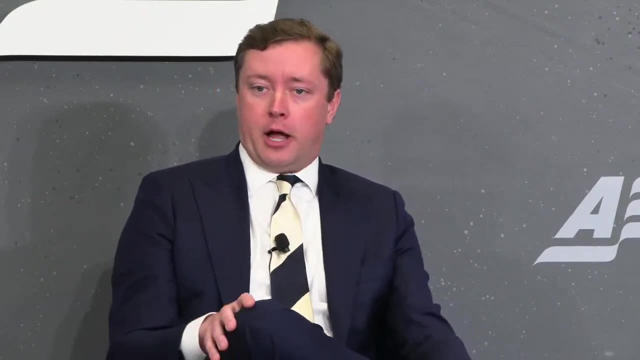 We don't ask companies that are innovating in the aerospace sector to send their technology to Airbus or to Boeing to create an appropriate line or level of safety to enter the market. So we've been tracking this really closely, working with regulators to share our concerns about what. 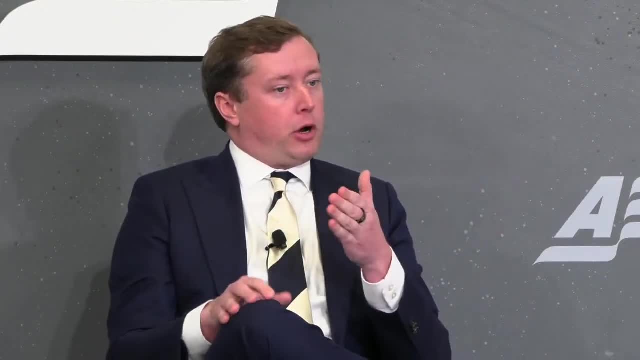 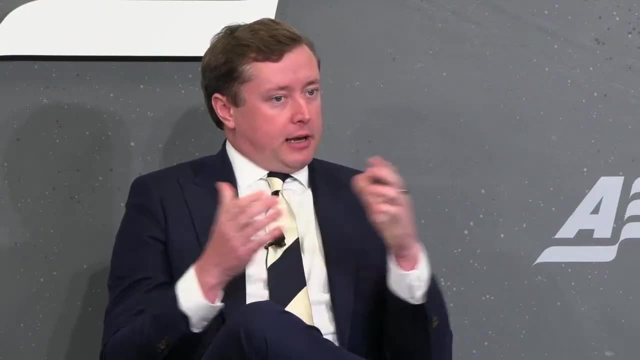 this would do in terms of creating a market or a go-to-market process that could be potentially anti-competitive. We've shared that, in the event that you end up getting into a system like this, you're going to end up seeing capital from firms like ours. 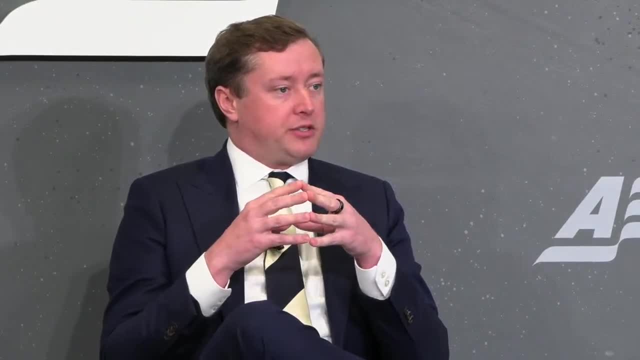 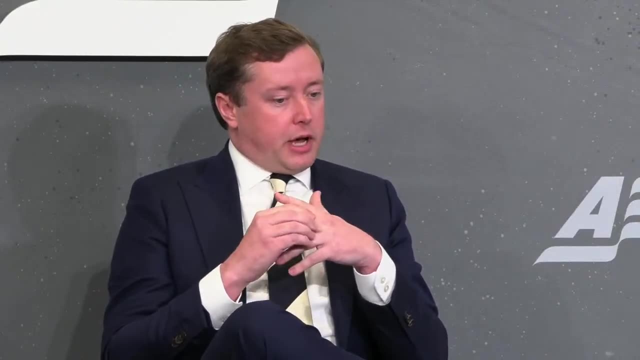 flow directly away from these technologies because of the regulatory process, And who's hurt most by that is patients, the health system and providers. So we've worked with them. It seems to sometimes fall on deaf ears a little bit, But I think the opportunity really here around assurance. 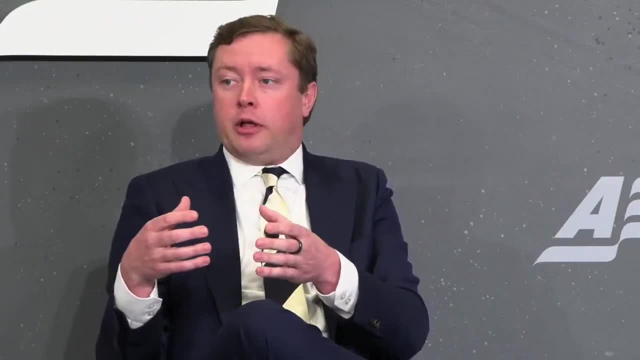 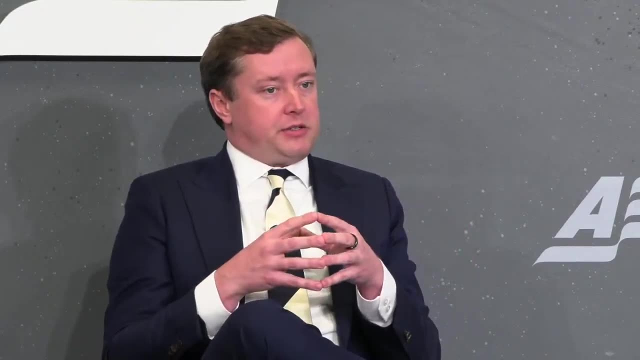 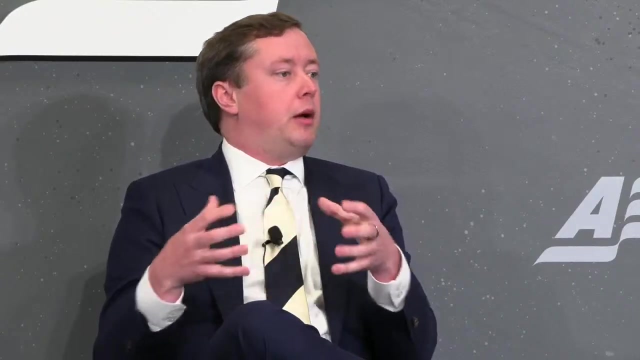 labs is a maybe different system or a different model that is, providing the tools necessary for different hospitals and hospital systems to validate against best practices and allow for them to start to integrate that themselves, versus having a more centralized organization that's making those decisions that's made up of the same organizations. that have AI incubator programs that are hoping to develop and commercialize in the same market as the companies that they're reviewing. So Yeah, Your thought would be having a choice of assurance lab models and then also having some decentralization so that hospitals can work as labs to test the technology. 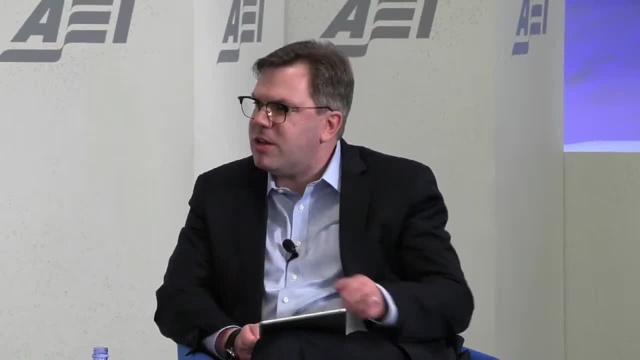 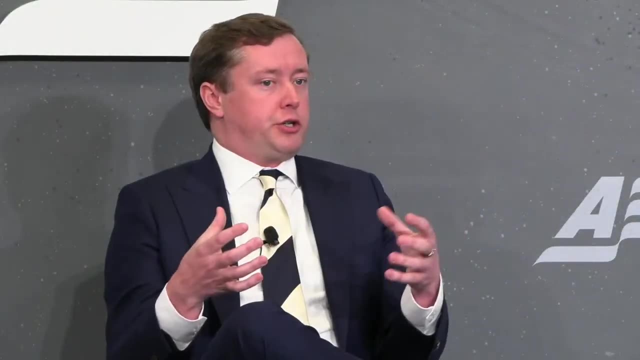 to continue to test and innovate on the technology that they are then integrating into their operations. Exactly, I mean eventually- you would want a system where every hospital is essentially an assurance lab, with the tools required and an understanding of the best practices of how to integrate this technology. 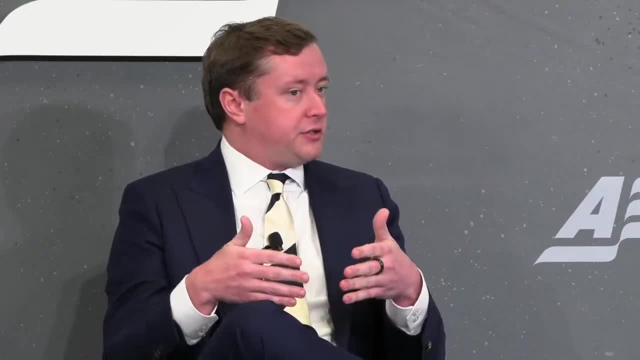 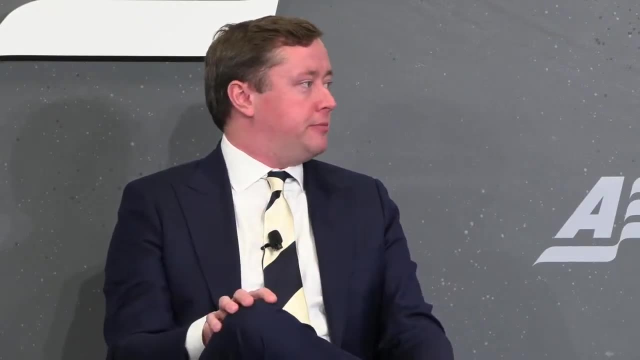 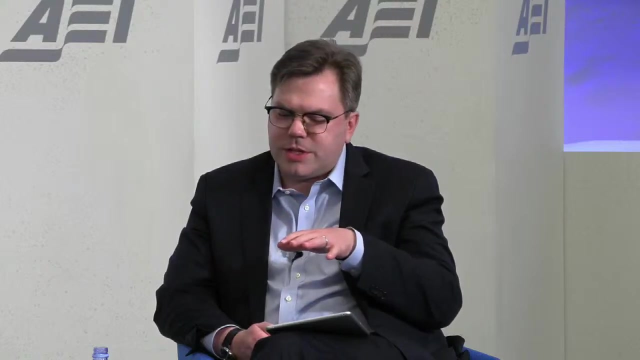 into their system and validate it against their own localized patient data, to allow for them to understand and make decisions around what's best for them and their patient population. So two questions. One first Mark in conjunction with thinking about assurance, labs and decentralization. what are the other things? 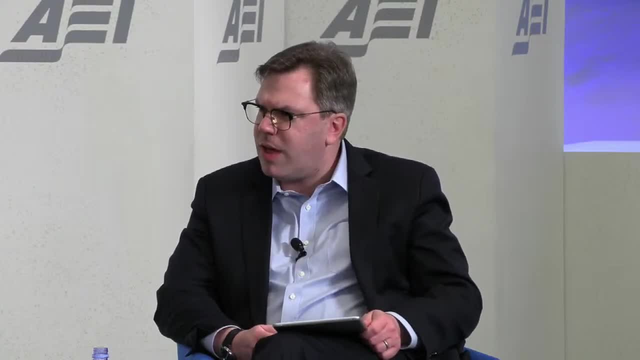 you think that the FDA should do to promote sort of the growth of AI, And how do they need to adapt their regulatory framework? I know that the FDA for many years- longer than I've been in Washington- has talked about voluntary alternative pathways, performance-based regulation. 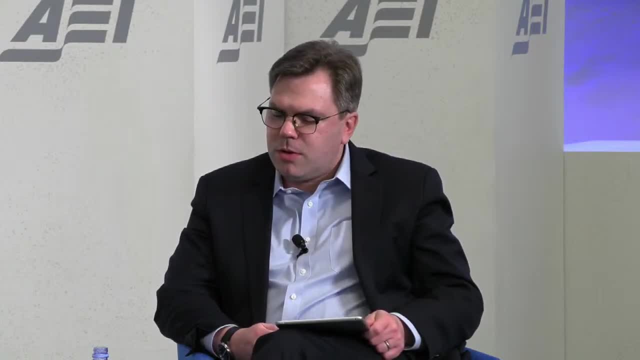 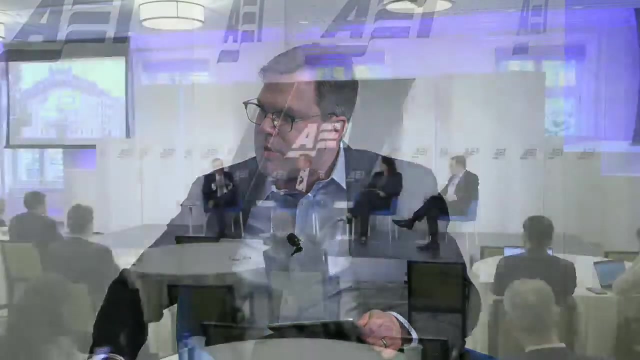 What do you think that the FDA should be doing to increase the efficiency of review, make the review more tailored to the innovator at hand, and then get those products into the hands of patients and doctors? Sure, Again, I'll give the FDA credit that they. 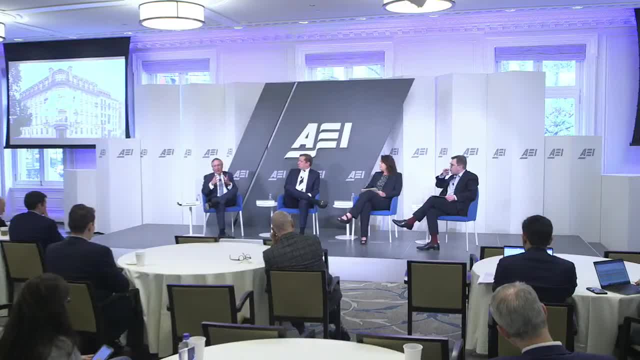 have been working on this for quite some time. As I noted earlier, just in 2022, Congress, in a bipartisan fashion, passed FEDORs, a number of FDA amendments, And part of that, I think, it's Section 515C. 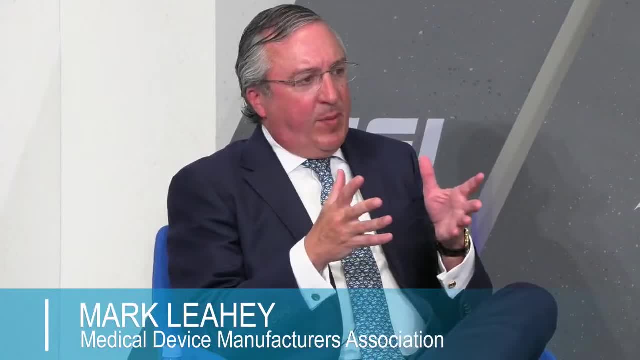 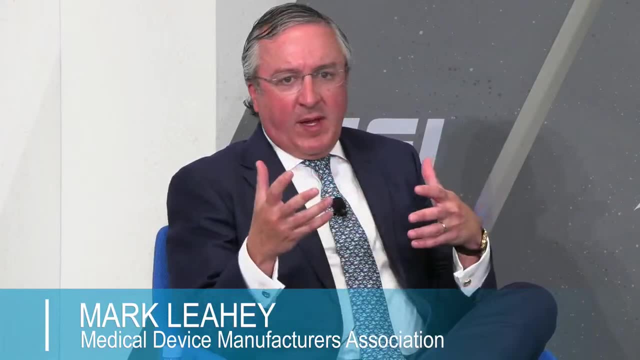 amendment to the Food and Drug Cosmetic Act provided the proposed change protocol plan that effectively, historically, you would bring your product to the FDA, They would review that to ensure it's safe and effective And you'd get your market authorization. And if you wanted to make changes, to that that were significant. that was an additive process And you had to have another filing. I think there's a recognition, in particular on software as a medical device, that there are known changes that you're going to need to make at the time. 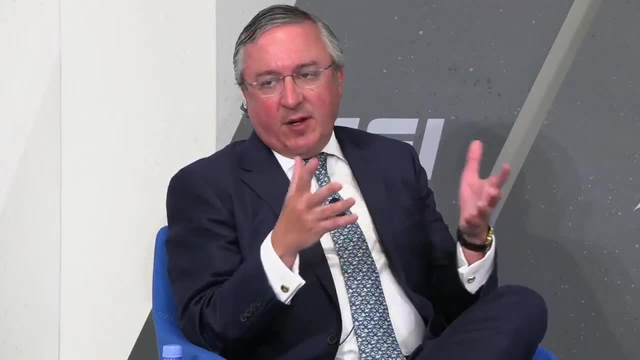 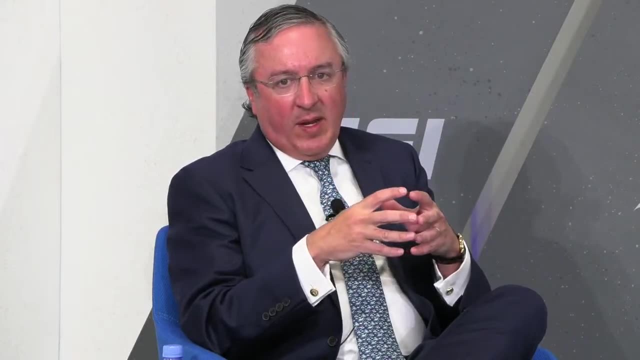 of your initial submission, And so, through this legislation, Congress authorized companies to come to the table with additional changes that they anticipated to make, And again there was an analysis of the quality system in place. The reasonings for those changes just couldn't change the indications for use and intended use. 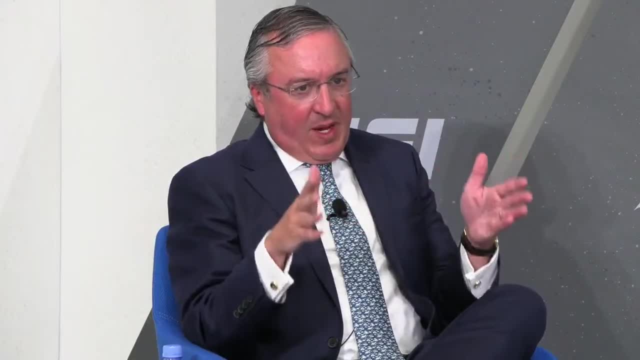 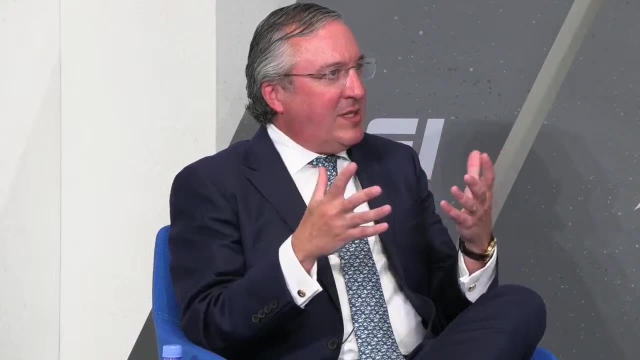 But provided as long as you stay within a certain kind of lane, those changes could be made without having to go back to the FDA. And so that has- and it's again early stages. I think they tried to. they've done it a couple times. 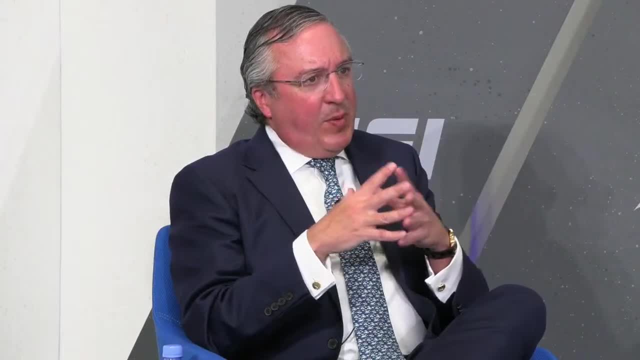 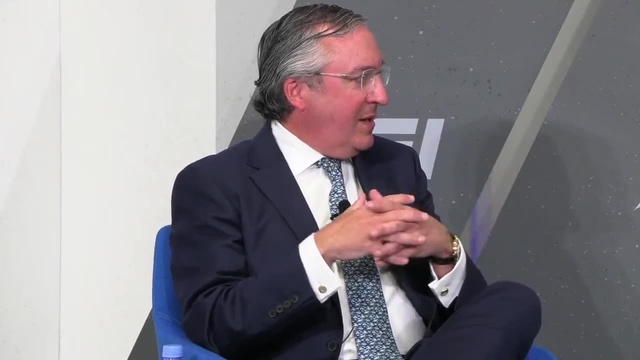 previously in the de novo in 2020.. But they put out a draft guidance. We filed comments. Congress has given them the latitude And, candidly, this is not just an AI machine learning. I think this is the PCCP. should be used broadly. 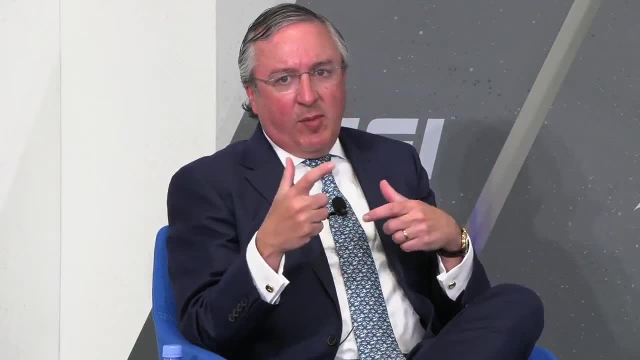 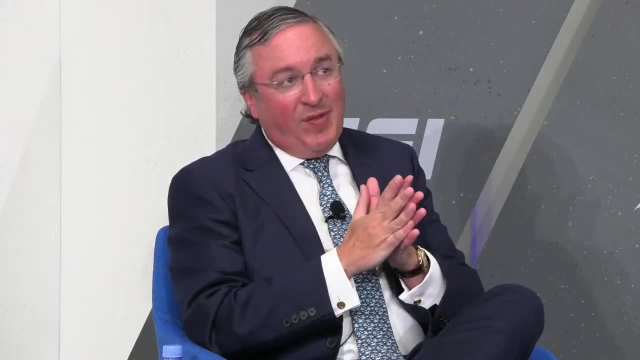 But here it certainly lends itself to more flexibilities for these types of technologies that maybe don't work within the traditional regulatory framework. A couple of years back, Maybe five years back, They were exploring this pre-cert program too, Again with recognizing that technology evolves quickly. 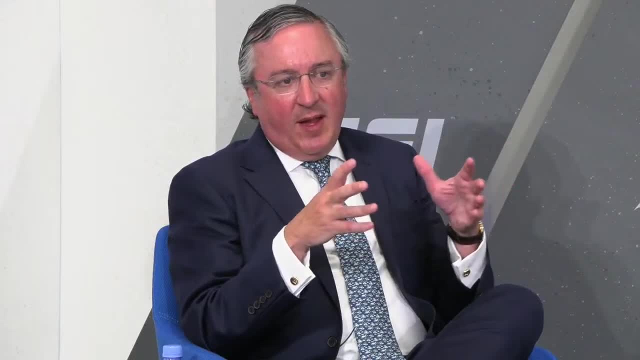 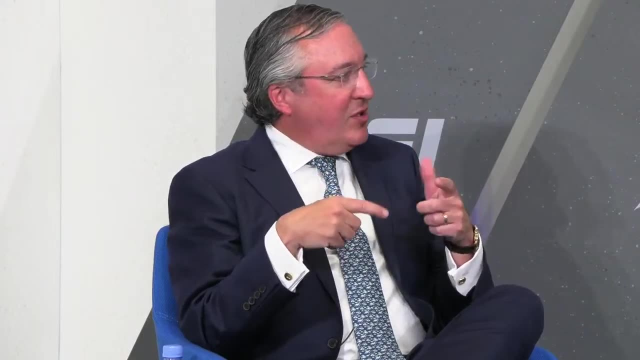 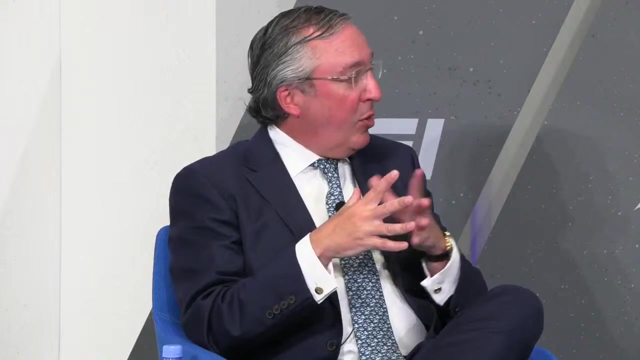 in software. could you have a pathway here that again, with companies who have a good quality system and proper guardrails, additional changes can be made more quickly? Ultimately, I think it was Senator Warren and Senator Murray basically sent a letter to FDA. 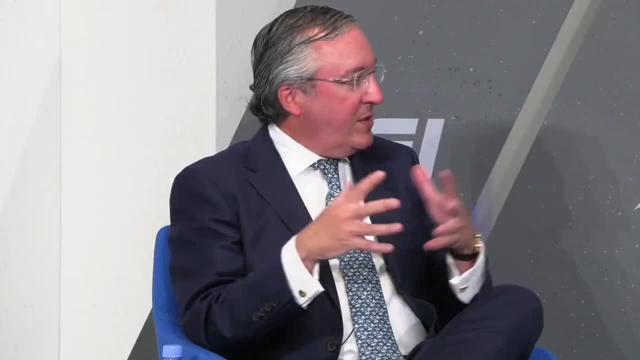 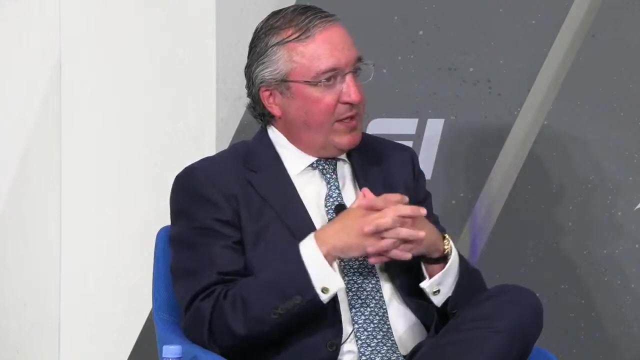 that their pilot needed to stop because they didn't have the authority to go beyond that and shift. different but related. I know in the LDT side there's been discussion of a lighter touch efficient review process for LDTs that maybe could be crosswalked here. 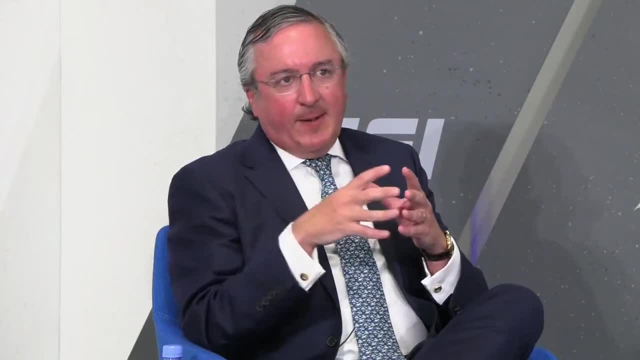 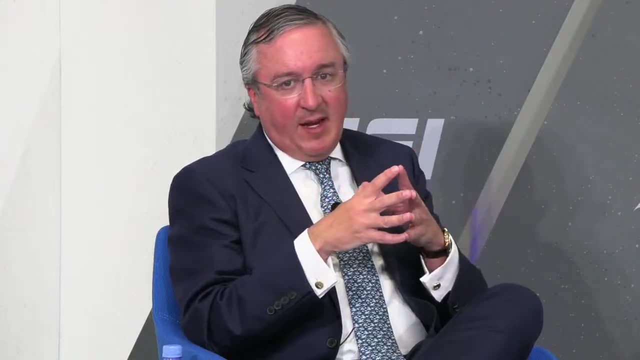 So those are areas where I think we'll give them some credit. I think, as Colin said, though, too, this is not something that if we continue to see the growth- and we've seen significant growth for these AI-enabled devices since 2018, and if we expect to see that growth, 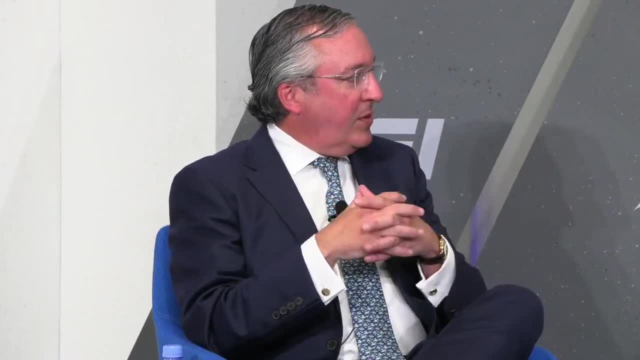 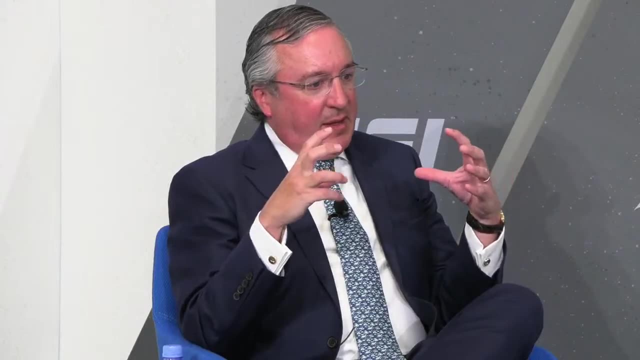 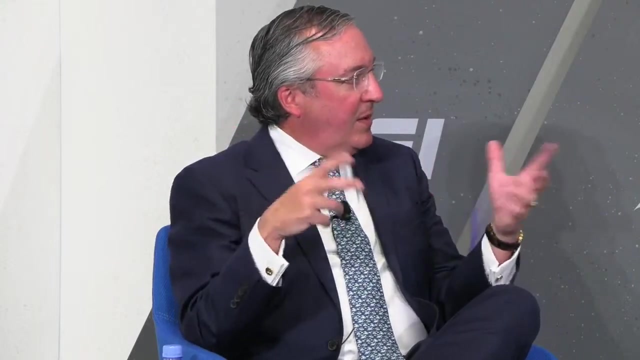 which I think we do. leveraging third-party reviewers, I think, is a great opportunity here. I agree. Having groups come together to develop standards and clinical specifications makes great sense. I don't think it makes sense for competitors to be able to dictate whether you're yay or nay. 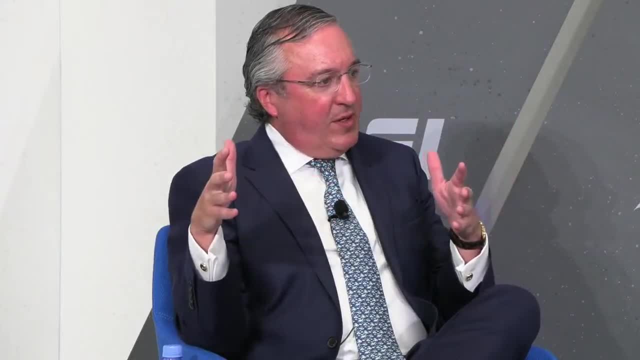 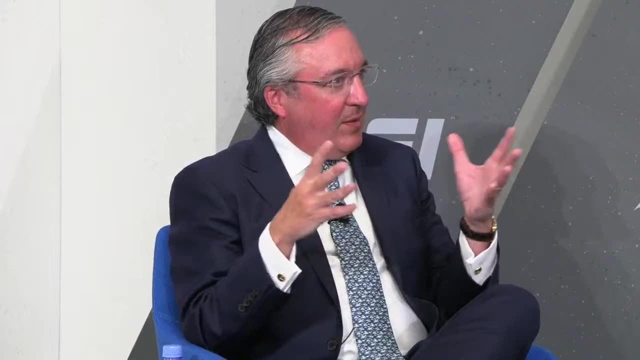 But having those groups to come together and then having third parties who can have the capability to follow those specs and to validate companies are doing it. that's how it works. Thank you. Broadly speaking regulations work in the EU for medical devices. 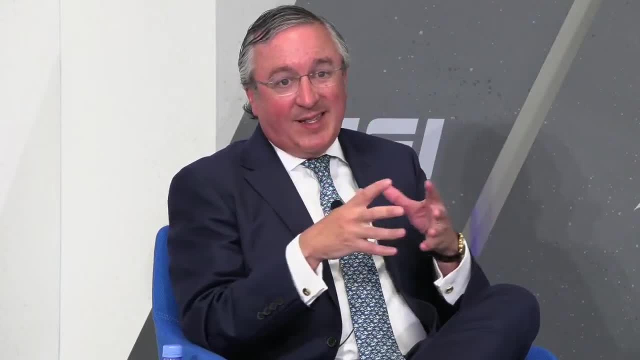 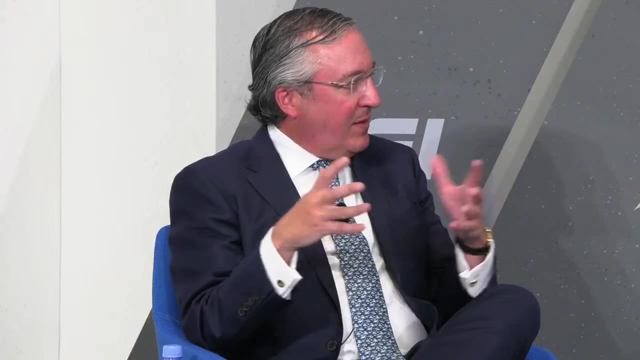 FDA has the authority to use third-party reviews here in the United States But Congress kind of put some really tight screens on that. that has limited its applicability. But I think this is a great area where that would certainly benefit the patient and benefit the ecosystem as well. 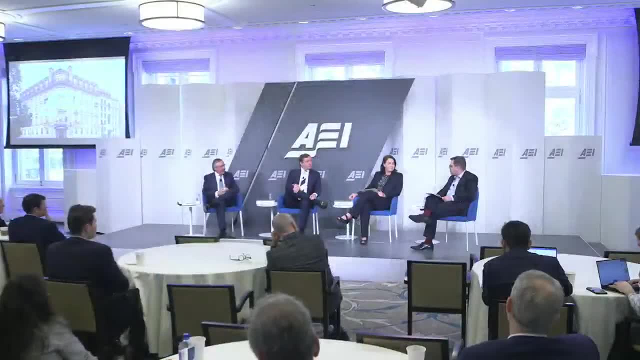 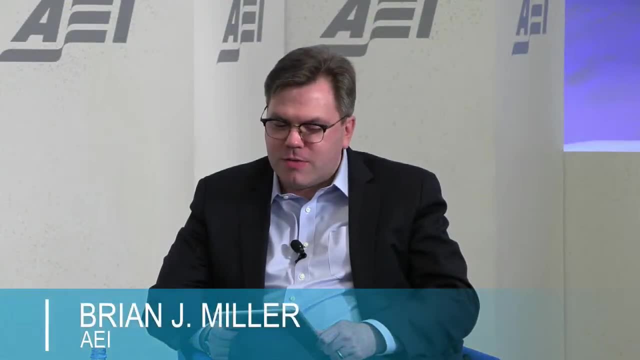 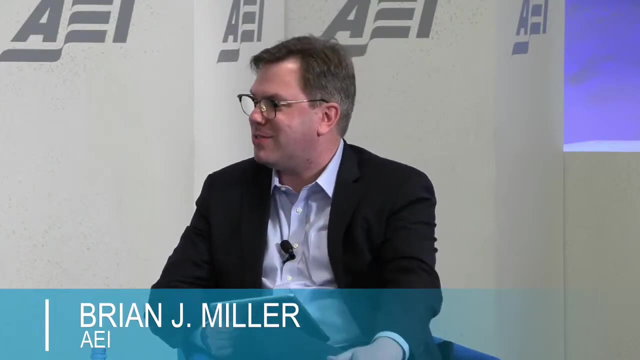 And not having to resubmit your application for version 5.3,, version 5.3.1, and version 5.3.2, probably makes sense for both the innovator technology company and also the FDA reviewer is going to be bored. looking at that just from a pragmatic perspective. 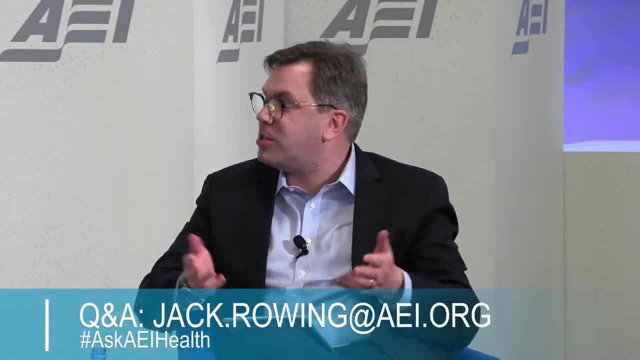 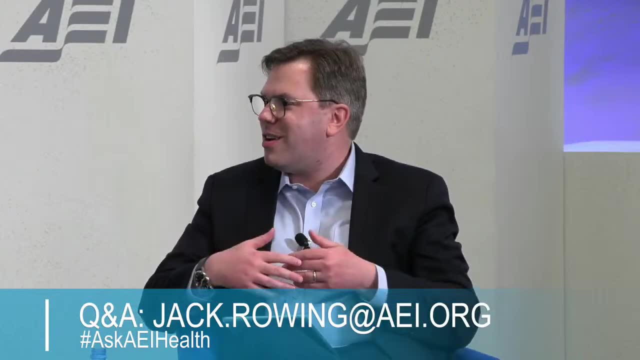 And the FDA doesn't have enough staff. You can only hire so many orthopedic surgeons, so many PhD biomedical engineers, whether telework, in-person work, partially remote work, The FDA is not going to be able to get enough staff to review all of the software that's. 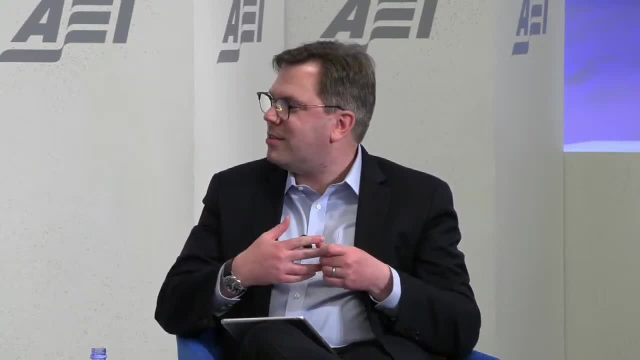 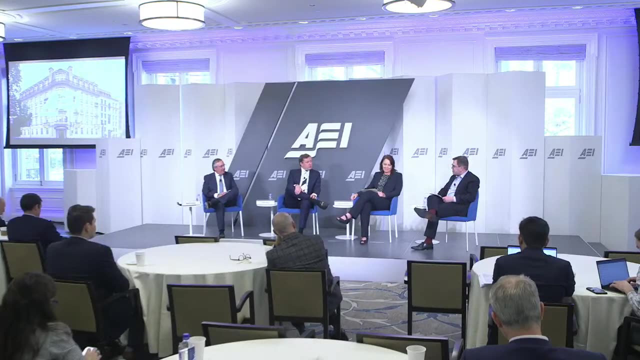 going to be classified as a medical device? Yeah, I mean, we should be hoping for an avalanche, right? This is. we hope that they will be overwhelmed, right Yeah? So a couple of questions, One I see from my physician colleagues. 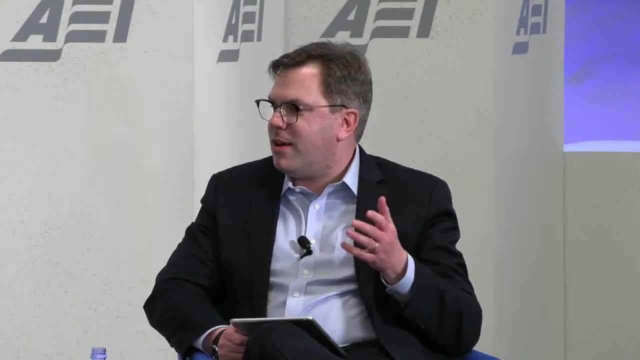 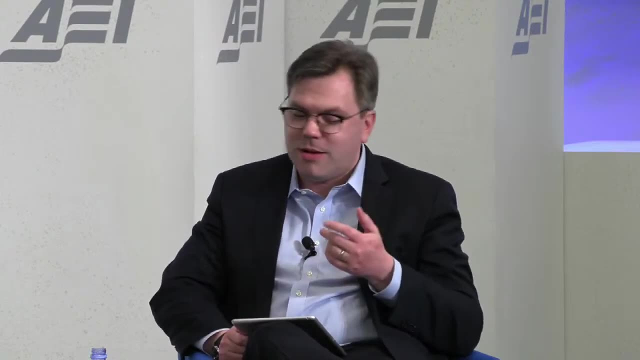 that there's a lot of anxiety about tech. Now I grew up out west so for me technology and disruption is sort of normal, like I'm used to it as a kid. I remember getting phone directions, Then I remember MapQuest. 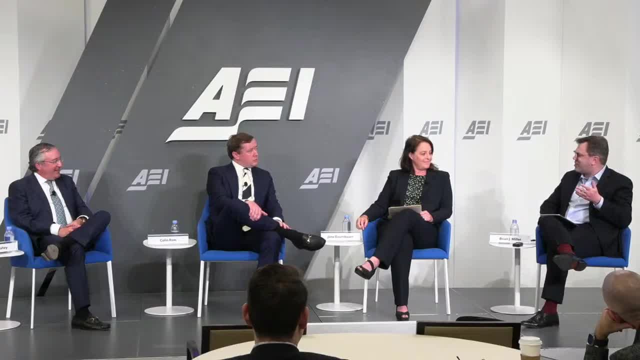 And you print out the directions. And then I remember you, You had touchscreen navigation in cars was a big deal. And then you got Google Maps. And now Google Maps plugs into your car because you don't even need the navigation in your car. 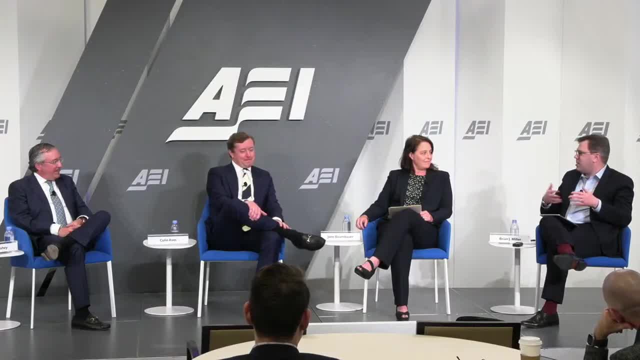 So for me, these transformations in all parts of life, be it from how I get around town to email, to calendars, to address books, is normal. But in the medical profession it's really scary for a lot of physicians And liability is one of the biggest questions. 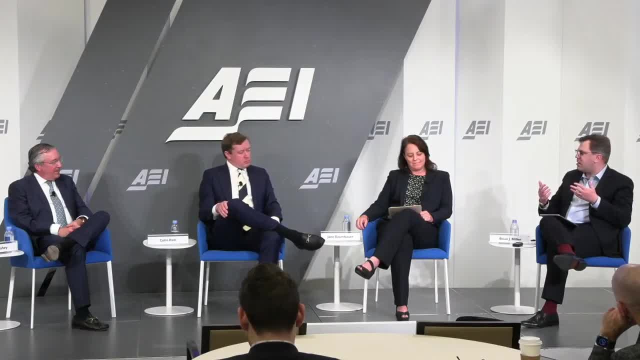 So my question for you, Jane, is: where do you think that this intersects with medical liability, And do you think that FDA and FDA review of some of the higher risk products in particular serves as a liability shield for physicians? Yeah, OK, so for physicians who are using an AI tool. 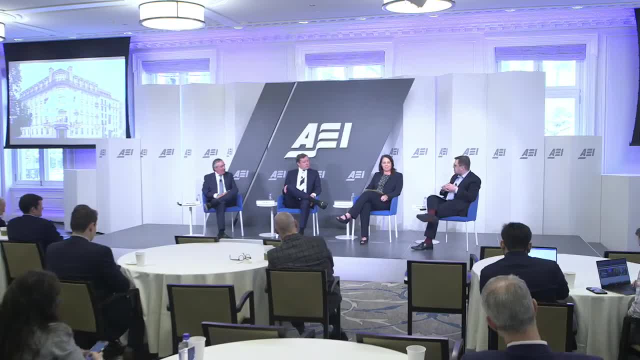 I think the basic principles of medical malpractice are still the right ones, But these new tools might introduce some kind of tricky line drawing exercises. So in general, a doctor just needs to comply with a broad sense of what is acceptable in their field. 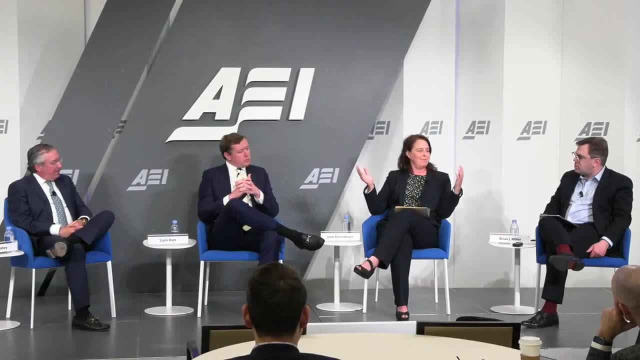 It's a sort of custom standard, And that makes a lot of sense, I think, And so I think over time you will see some cases where a doctor used a tool that was clearly not ready and they should have known it, or maybe it wasn't even FDA cleared, or something like that. 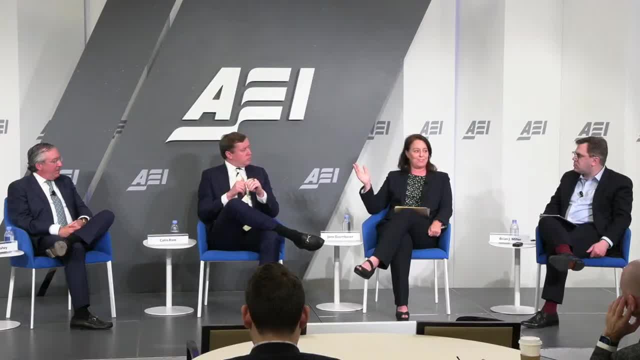 They might be held liable, But, over time, I think you'll see cases where a doctor failed to use an AI tool, And so the basic question, though, seems to me to still stay the same, which is whether they were engaged in reasonable care as compared. 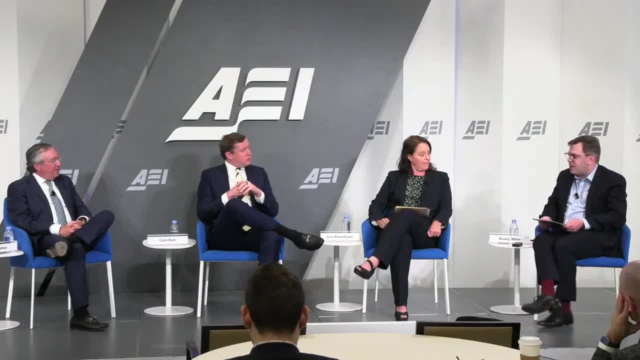 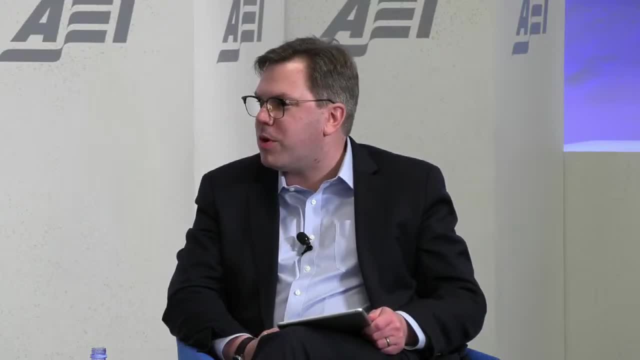 to their professional colleagues. You said something actually really interesting there, which is that the standard may be that the doctor didn't use the tool or use the tool inappropriately. Yeah, In fact, you've seen that there are some cases where a doctor can actually be held. 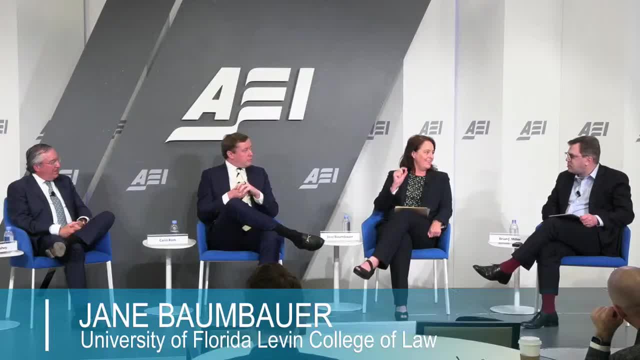 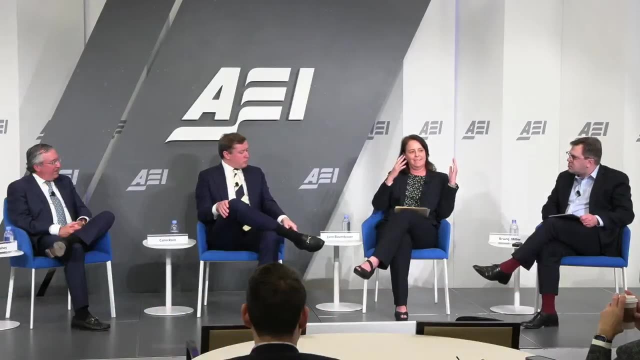 liable for not prescribing off-label a prescription. So the standard for doctor care is not necessarily the same as the standard for FDA. The standard is simply whether the doctor failed to be within either the majority or a significant minority of doctors, And so that's a big question. 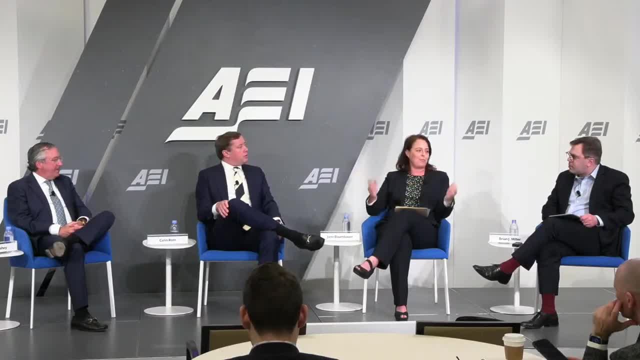 And so I think that's a big question, And I think that's a big question for the FDA, and I think that's a big question for the FDA as well. who would think that this is an appropriate, you know, one of the appropriate ways to go? 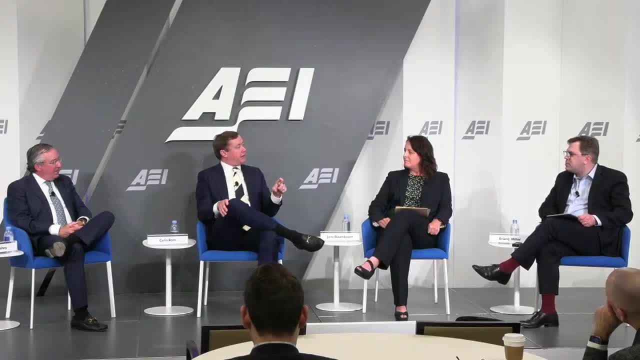 Go ahead. Yeah, I mean you can look at as part of that conversation though that we're having now that technology is here today And there are situations today where it could constitute malpractice for not integrating some of these AI-based technologies. 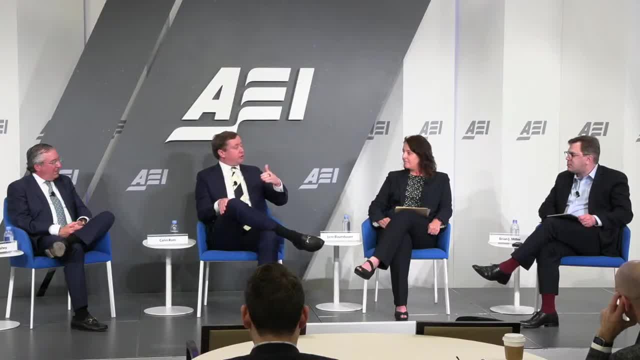 like mammographies or colonoscopies, where they have to go back into a subsequent or additional colonoscopy. So I think we're seeing that a lot today And, to your point, a little bit Brian, culturally one of the things that we found really interesting about this. 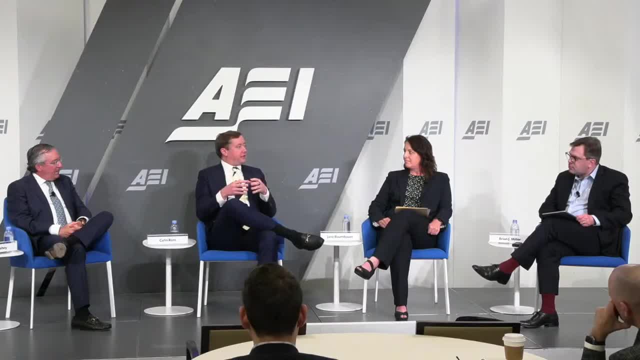 is. you would assume, some of the more high-tech or more advanced hospitals and hospital systems are the ones that are first to integrate this technology, And what we're actually seeing is kind of cold outreach from some of the more rural patient populations and provider groups asking us: what's here today? 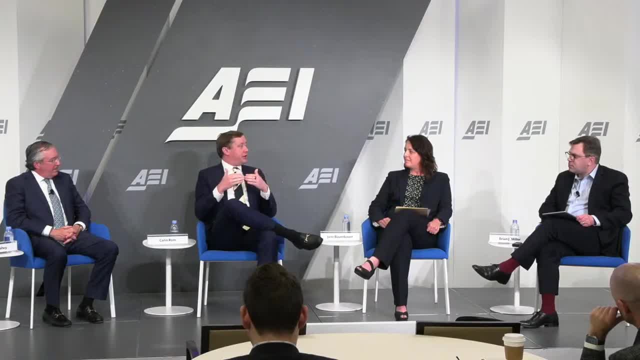 What can we do to help facilitate better care and better technology to make sure that our organizations are going to be capable of taking care of the patient populations, as we have a huge dearth of providers in our area or in our network? Sorry, just to add, I'd say, the main question. 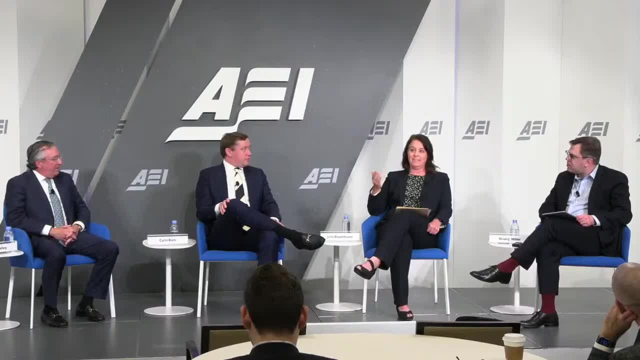 is whether the reliance on a tool was either reasonable or whether non-reliance on a tool was unreasonable. And the same should actually apply to direct-to-patient or direct-to-consumer- whatever you want to call it sorts of applications as well that in some cases, 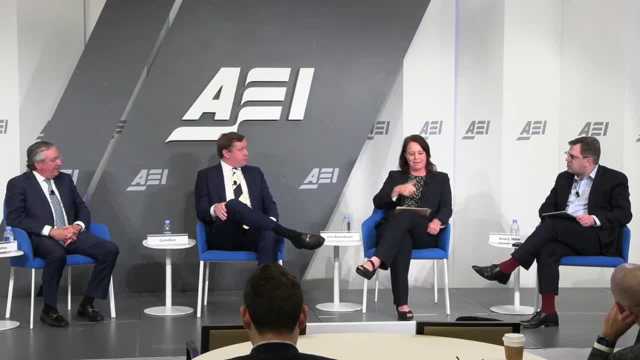 we might want responsibility. So between the three- the patient, the doctor and the producer- shifting responsibility and liability will depend to some extent on whether, in the particular context in which the tool was used, it was erroneous for the user to rely on it. 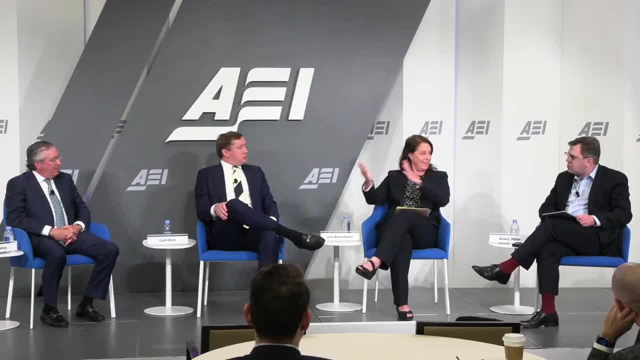 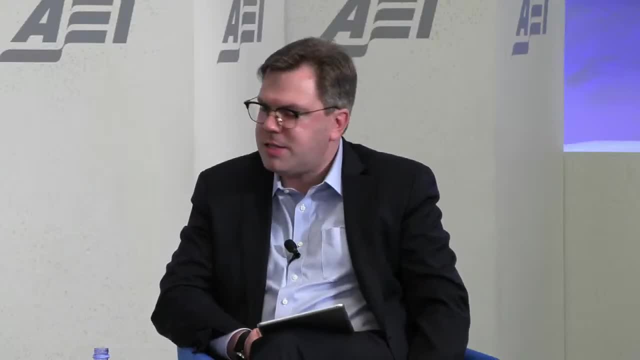 erroneous for the doctor, or if their reliance made sense, then maybe that's when the liability needs to shift to the company. So it's interesting we talk about tech changing the standard of care. So in the ICU, if you're on pressers. 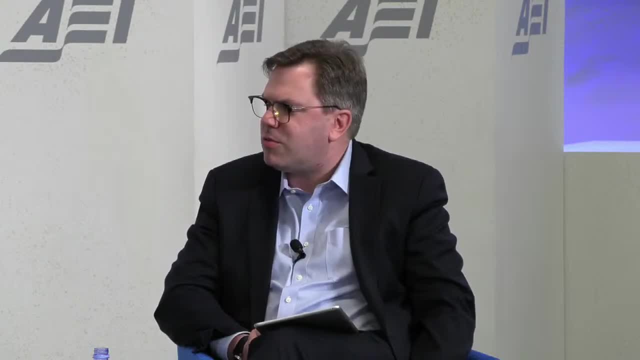 to keep your blood pressure up because you're critically ill. they have to place a central line right And because it's a continuous infusion, it has to be delivered centrally. And that's risky because central lines go in places where there are big veins, where there are other important arteries and nerves and things, so you have to get in the right spot. If you accidentally cannulate someone's artery, that's really bad and they have to go to the operating room with the vascular surgeon emergently. So, as you can imagine, this is high risk. 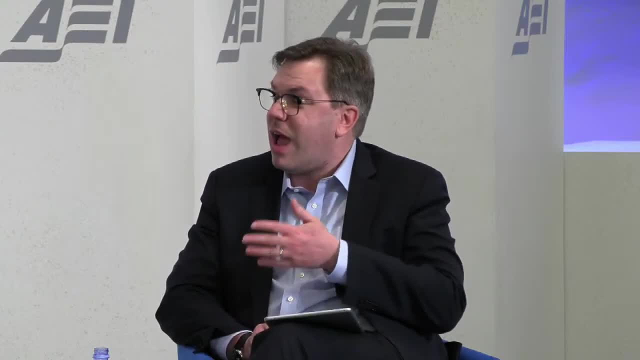 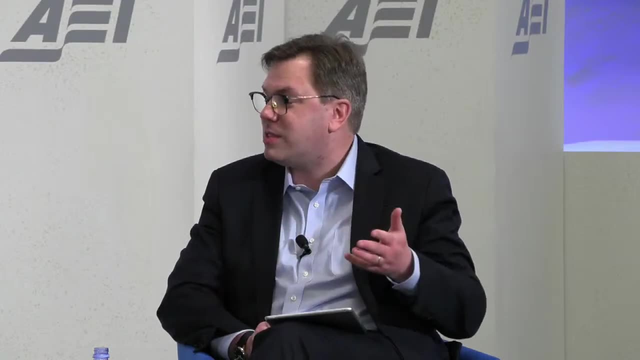 And 30 years ago, 40 years ago, they didn't have ultrasound to do that, And now the standard of care is ultrasound. And so if someone tried to do that without ultrasound, you would run screaming into the room asking them what they're doing, because the standard of care 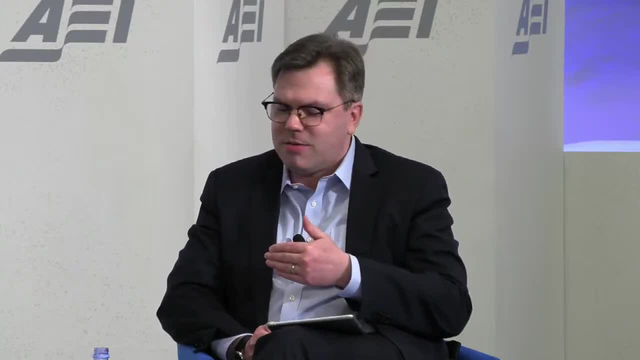 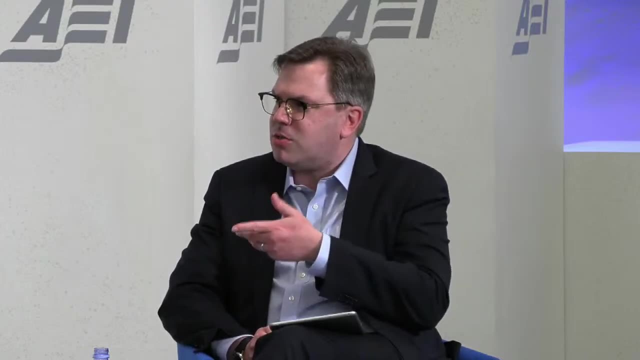 is you have to use ultrasound. Not using ultrasound is negligence And I think a lot of these tech tools will eventually get to the point where they're so integrated with care. And, Colin, you mentioned rural hospitals. If you have a staffing shortage, you have travel nurses. you can't afford travel nurses. you have part-time doctors, you have temporary doctors. you have a budget crunch. you have a population that travels two hours in a blizzard in the middle of the winter to see you. you have a limited resource environment. 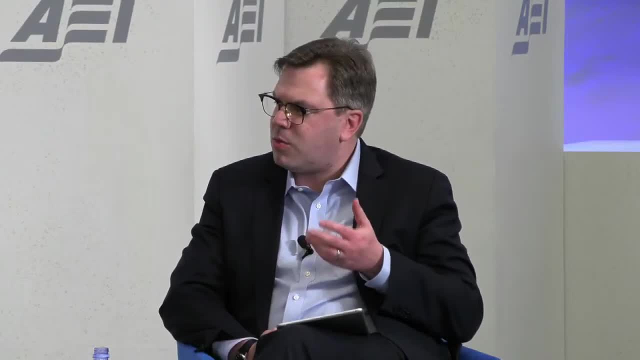 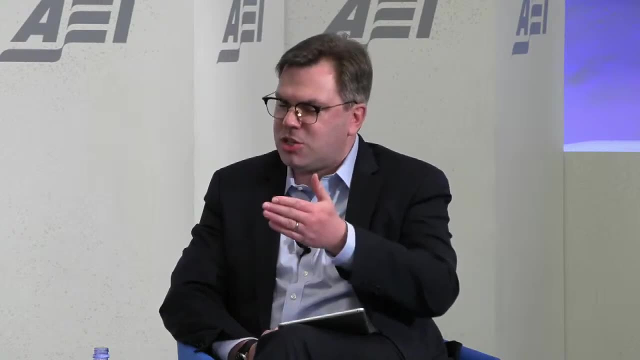 And the most cash-strapped environments are the ones that are going to have to be created, And so they're going to be looking for technology to be that additional adjunct or accelerator of the doctor, nurse, pharmacist or whomever is actually there. 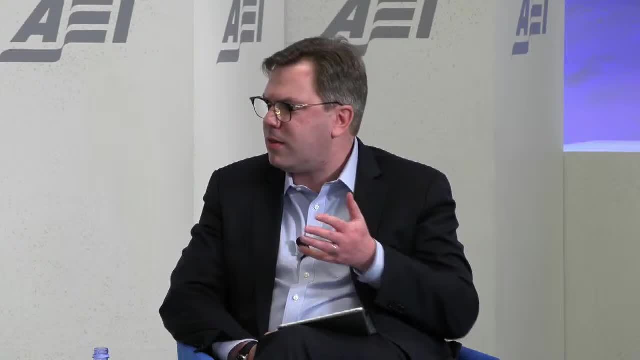 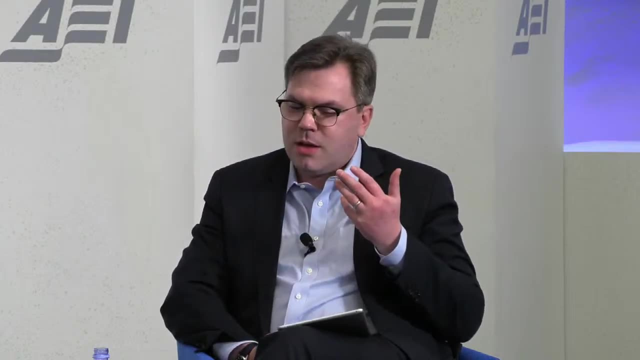 or is going to be there, And so when we think about adoption, the financial stress that rural delivery systems experience will actually make them probably some of the most advanced delivery systems. But the question is, what is the barrier that you see in the Medicare program? 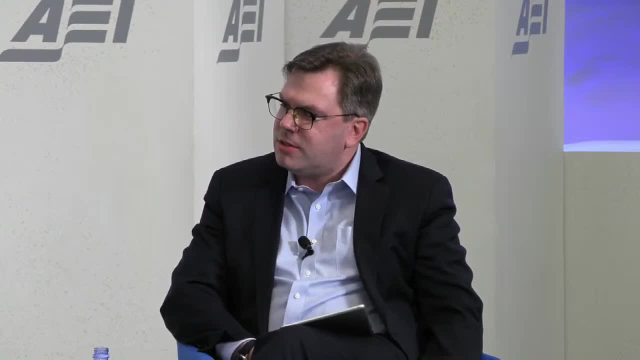 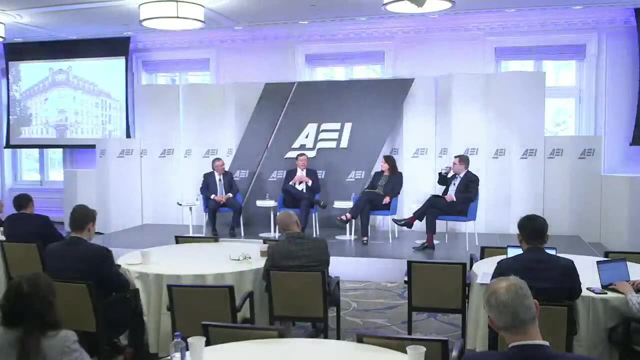 and in reimbursement for AI and automation. Well, I think we're seeing two things. One is just the general gray area from the regulatory perspective. We don't know what it's going to look like in terms of long-term reimburseability. There's a little bit of difficulty. 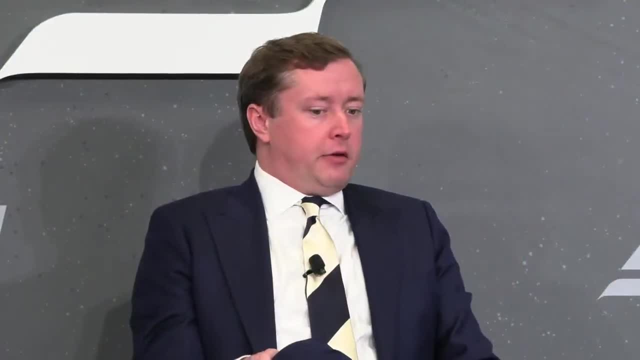 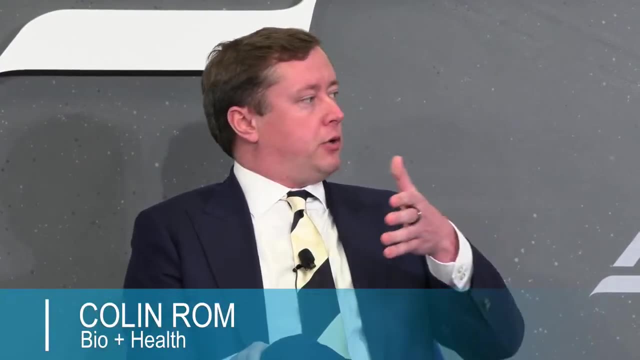 from kind of a cultural perspective to your point earlier of, like physicians aren't sure whether this is the right next step or whether this technology can be integrated, because we don't know what the future regulatory structure is going to look like and how that will basically impact practice. 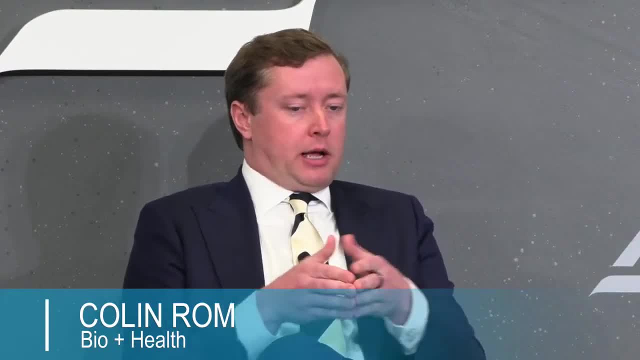 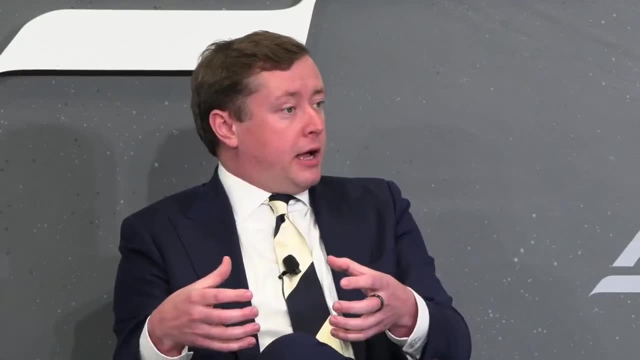 So one of the things that we've been working with regulators on is kind of: what does the future look like? How do you reimburse for care that's either delivered or rendered directly by an AI service or model? Or then, what are the downstream impacts? 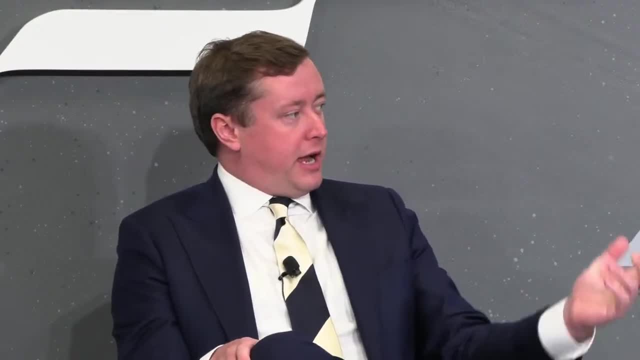 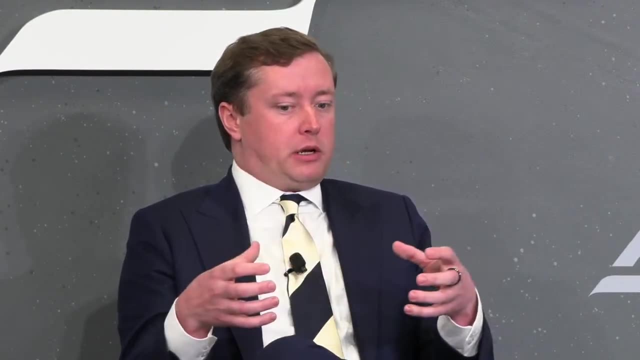 And I think one of the things that we're seeing is that, to your point- and we had a meeting with some of your folks on your team about four or five months ago where they were talking about what are the ways that we can- 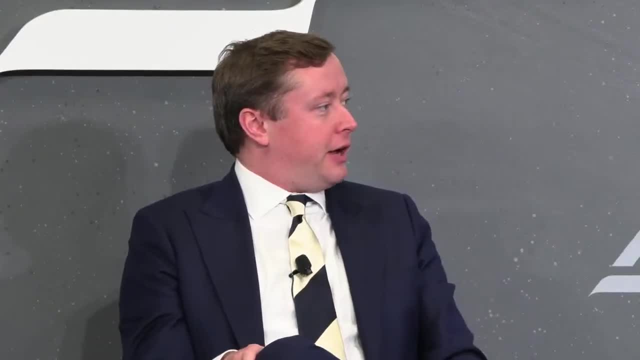 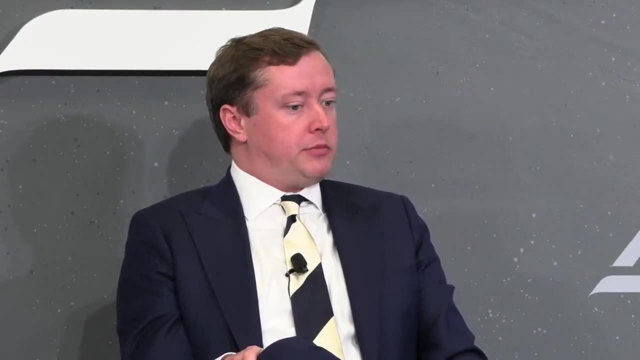 leverage technology to have that be the initial entry point into the health care system, And I think it's not just Medicaid where we're seeing a lot of this too. It's a lot of difficulty when it comes to tech companies and startups trying 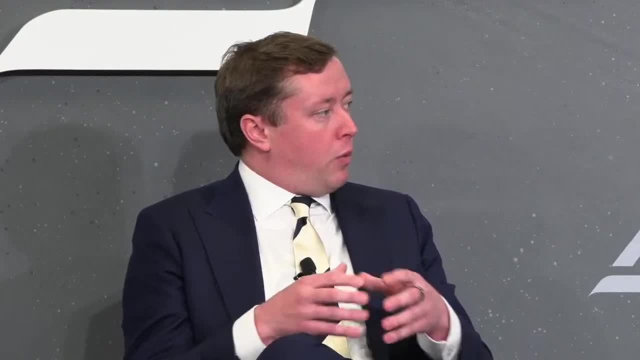 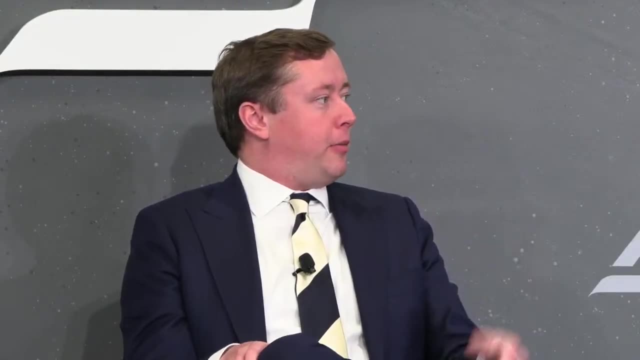 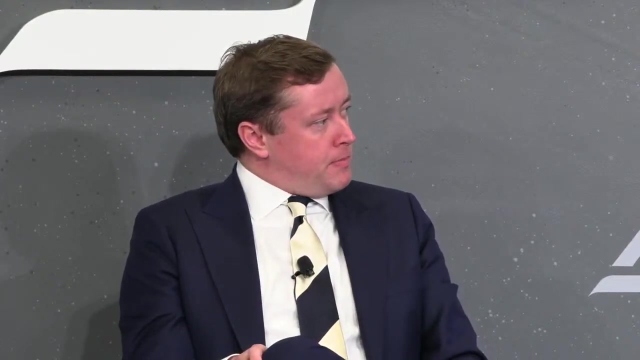 to help better integrate into the Medicaid program, and thinking about what that impact could do to ensure broad access to this technology and also have a better, cost-effective care model for these patients that are largely underserved and aren't having better outcomes over time. So a question that I was just thinking about earlier today. 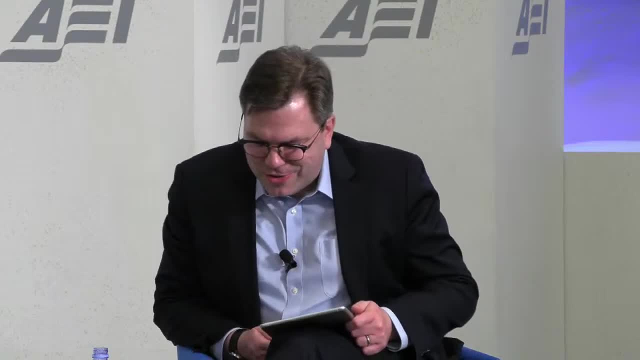 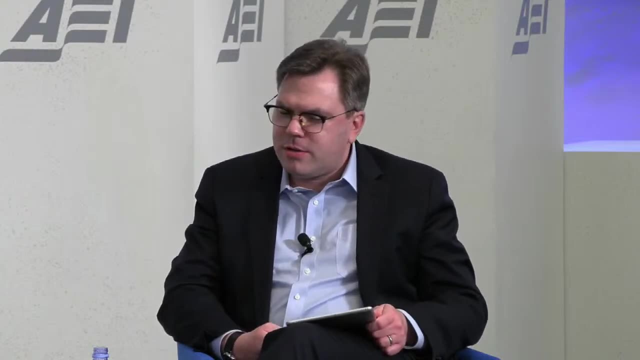 after I had a lot of caffeine. is, you know, like in the Medicare program, the Medicaid program, whatever the payer is, there's a conception that it is a person providing the service, And everyone is always trying to become the person providing the service. There's always another professional that's trying to become the person providing the service right. First it was doctors, then we had nurse practitioners and all kinds of other health care professionals want to be billing health care programs, But technology is different, Because it can do so with more efficiency, potentially. 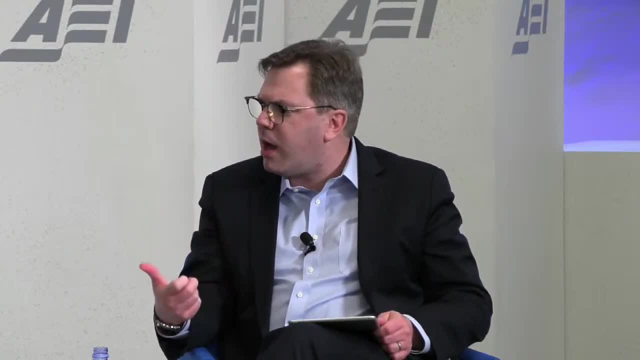 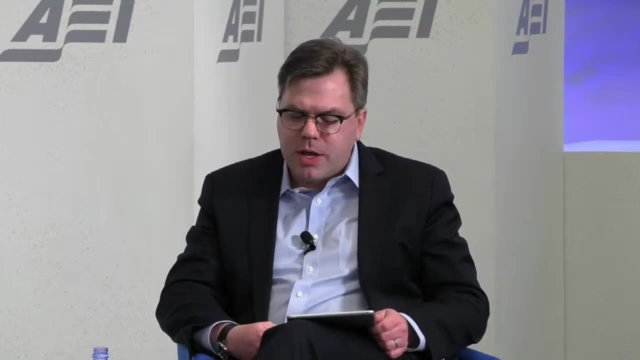 in some settings- Not all settings, but in some settings Maybe higher quality, Definitely potentially better safety performance in some settings too, And so I guess my question is from a service perspective, like if you're an innovative technology company. 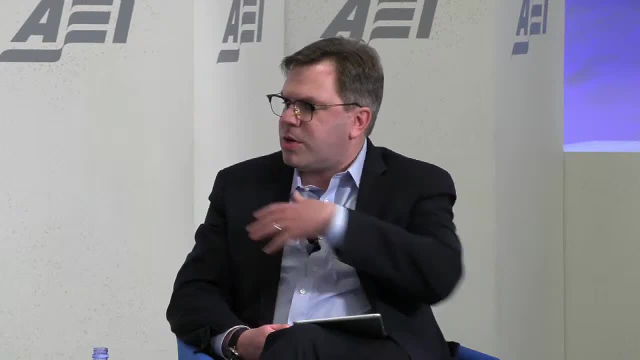 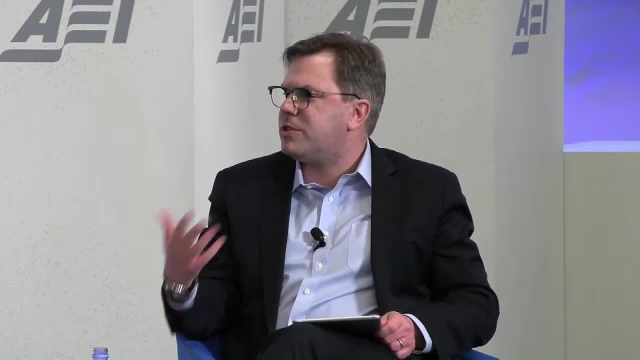 do you think that an innovative technology company- and this is a question for all of you- should be able to bill a payer for just delivering a routine medical service? So if I have a urinary tract infection or I have pneumonia or I have high blood pressure and I 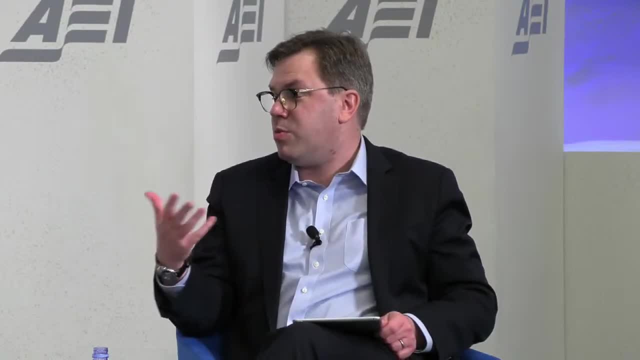 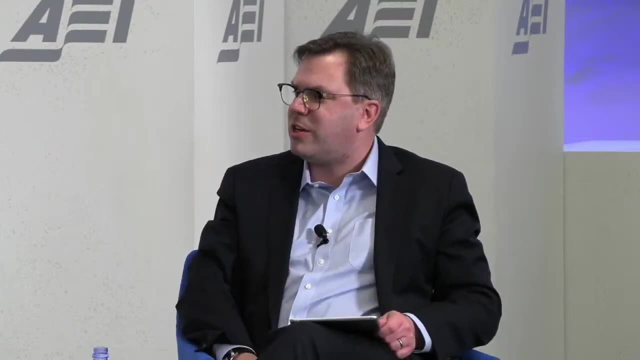 can have software diagnose and in theory prescribe- I mean, I realize there are state law issues there, but let's say it could- or titrate my blood pressure medications. do you think that the technology should be able to bill for that service? 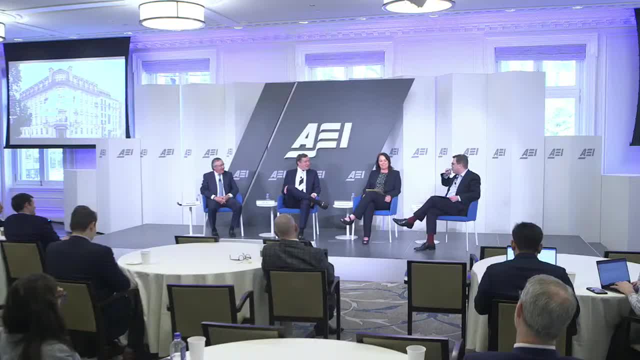 Because we all turn and look at Jane. Yeah, The reason I put it that way is because I think you know it's just a matter of time, So I hesitate to say one way or the other. is, on one hand, yes, of course we want good enough treatment, maybe even 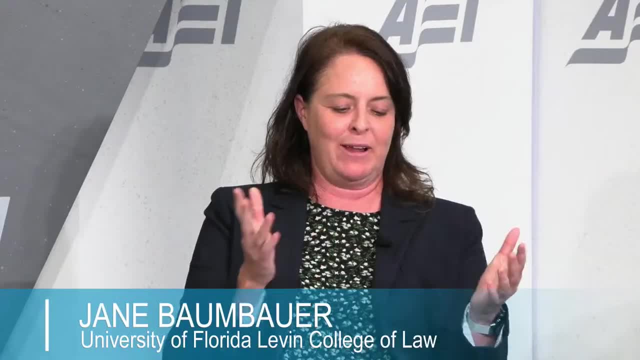 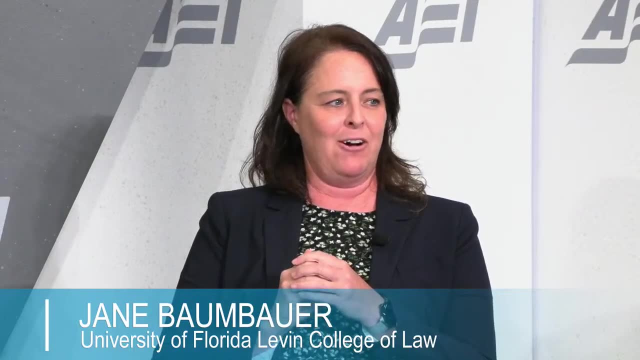 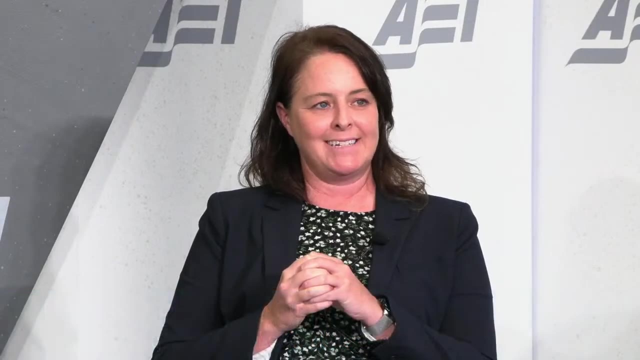 treatment that is as good or better than the treatment we have today in a human-run clinic. Of course, we want that to be able to be offered directly to patients, including those on Medicaid, without whatever cost burden there is. The reason I hesitate, though, is 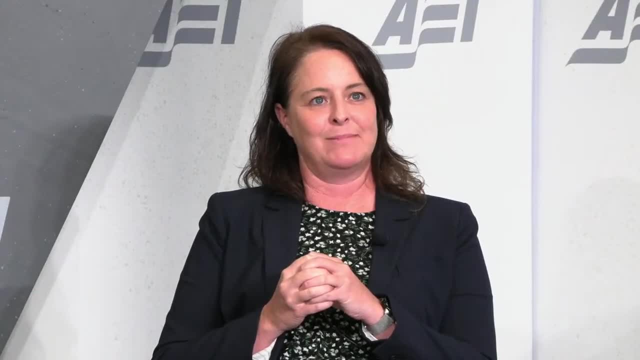 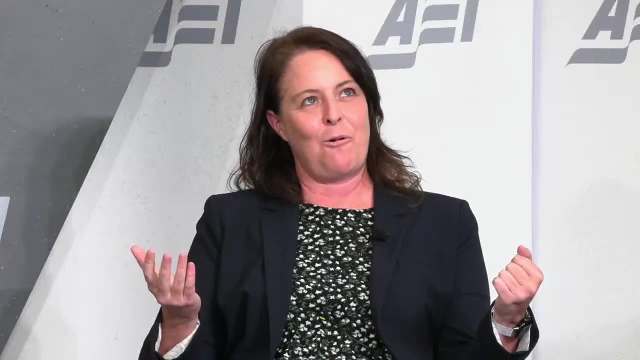 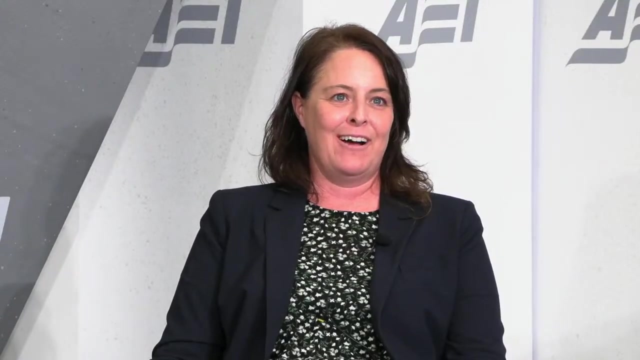 that you know Medicaid and Medicare programs, you know the secondary payer just sort of masks a lot of the costs and I still see- perhaps more than my colleagues here- I see some potential for a direct-to-consumer- not patient but consumer- market. 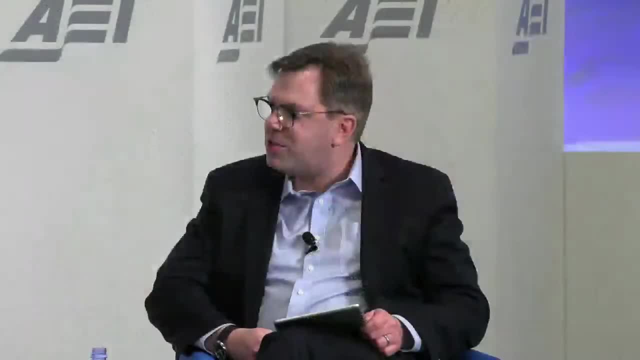 I'm a fan of direct-to-consumer also. What was that? I'm also a fan of direct-to-consumer. OK, right, And so if we think about like- because in health policy we always talk about paying for value and you know like, 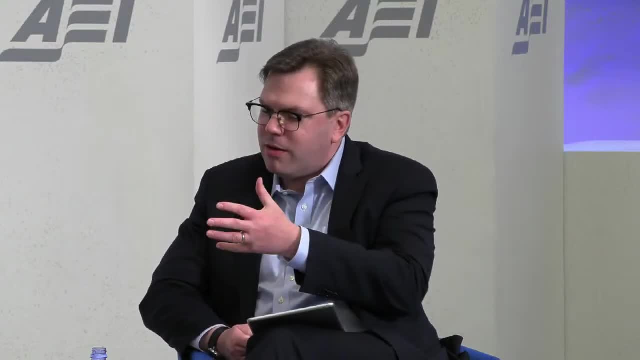 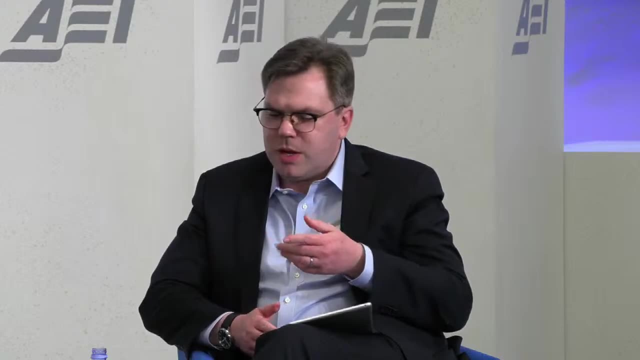 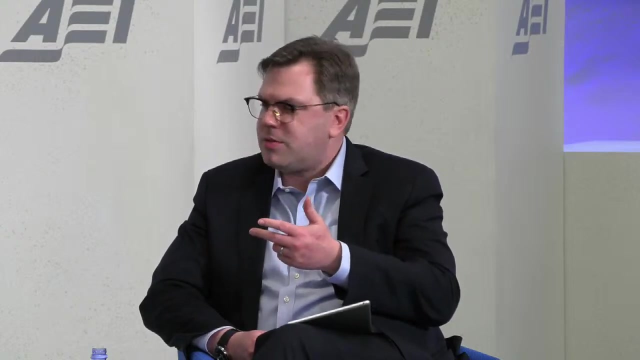 that's benefiting patients. but if we really want value and we really actually want to benefit the patients right, you need appropriate competition between technology, technology-assisted human service and pure human service, because you know we have a shortage of what is it? 100,000 doctors. 90,000 nurses, we don't have enough CNAs, we don't have enough patient care techs in the hospital, we don't have enough telemetry techs, we don't have enough pharmacists, like the list goes on. 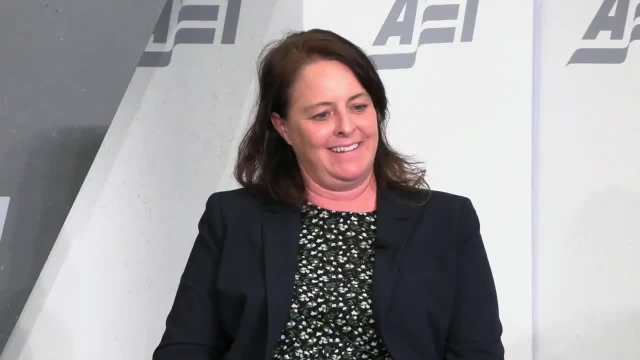 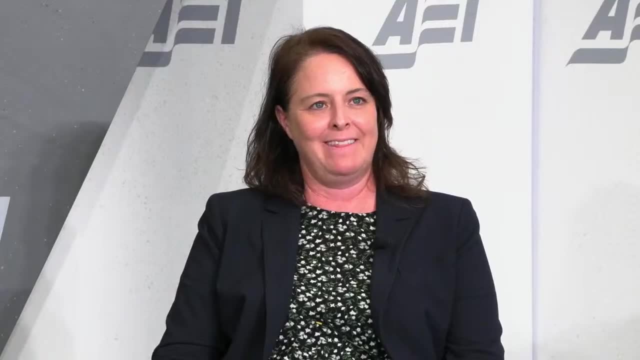 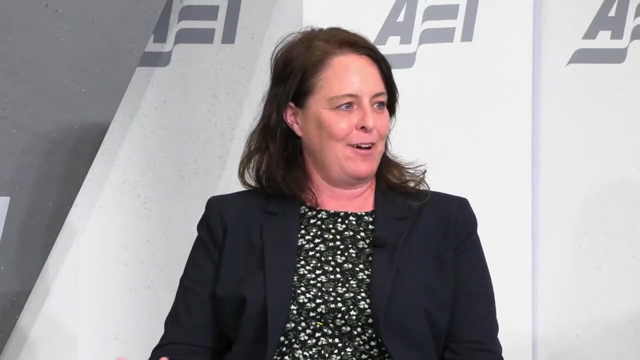 Right and there's very little risk that these that, like AI, is going to take over all of these jobs, And the legal profession is going through this too and there will be a need for clinics period, But there is a vast amount of unserved, you know. 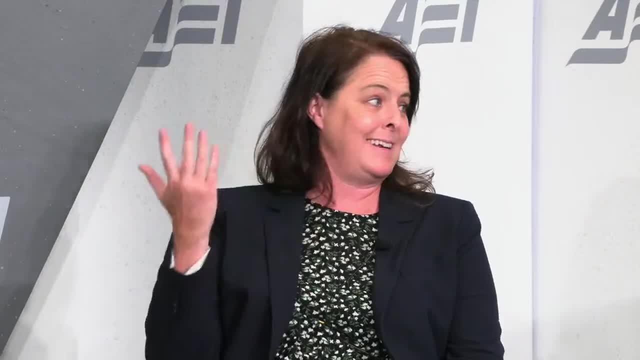 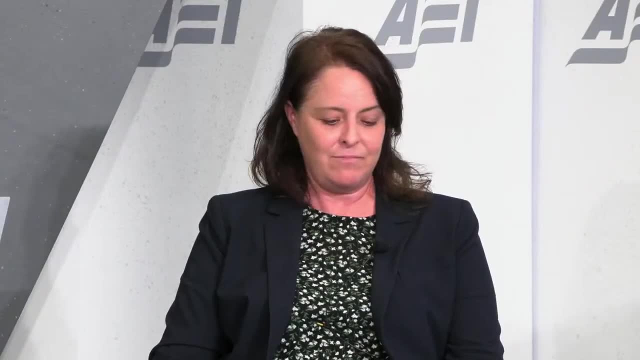 health needs, including by people who have insurance and you know privilege and who just don't have time or whatnot. that should be served by a direct-to-consumer market And a direct-to-consumer, or even rather direct-to-consumer through a payer. 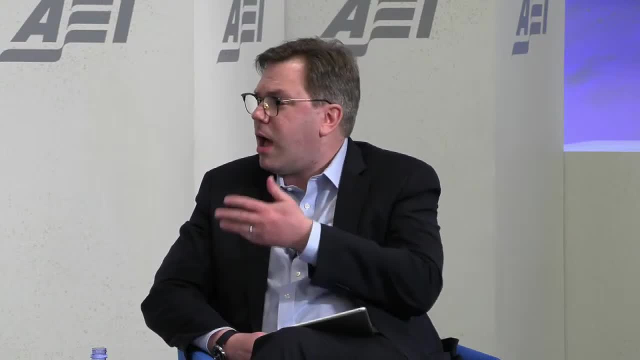 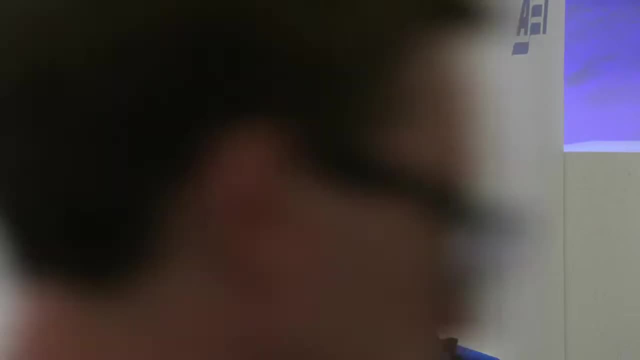 technology could massively expand access to care, high-quality, safer care for the poor, for the middle class, because wealthy patients are always going to be able to afford to get access to care. It's the average American that we need to worry about. 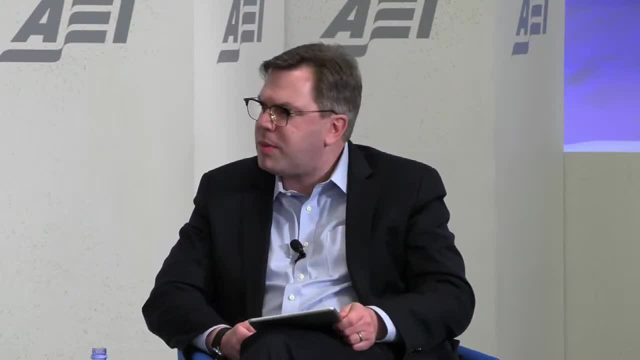 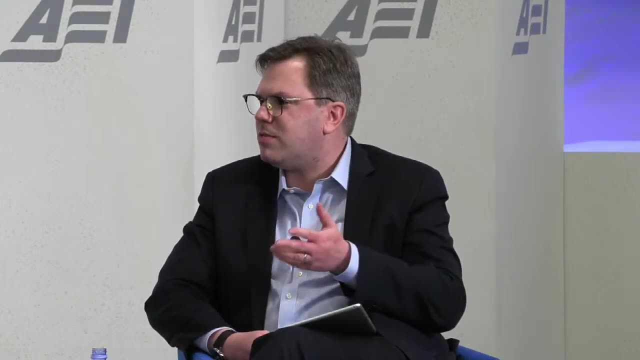 or the working poor. That's the patient population who benefits the most. Right, that's the patient population who benefits from the most. So is there a way that we can promote paying for the value and efficiency of technology? because, at least my personal view, not the view of any of my affiliations- 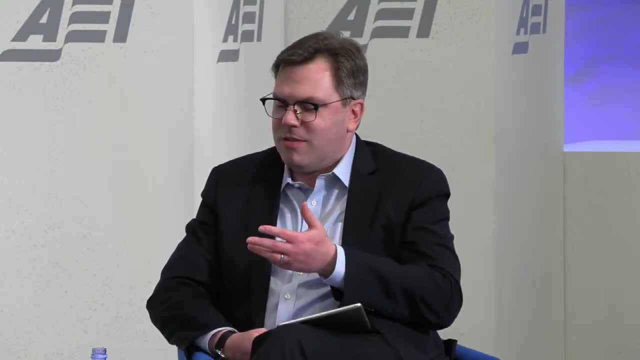 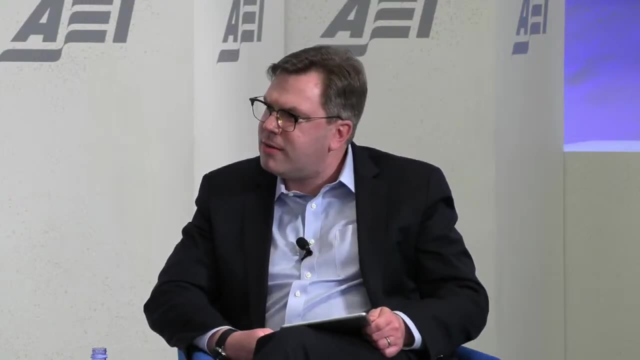 obviously is that we are not valuing technology and paying for that efficiency and democratizing access to care for the average American. Yeah, I mean, I think maybe to take a step back a little bit from this. there is also a concern from some. 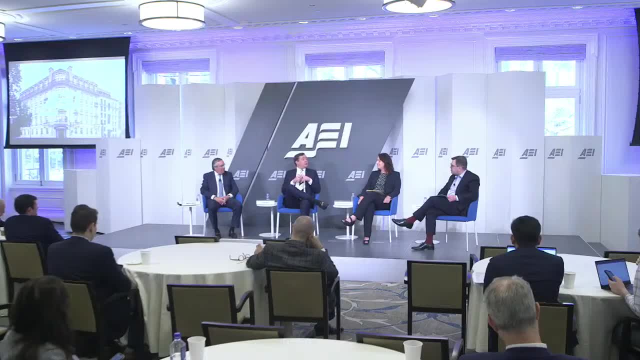 of the innovator companies that largely, like no one, wants to be first to market with an AI doctor service. right, That's going to bring on the most scrutiny, regardless of, you know, the interesting part that we have. that may be a little bit different. 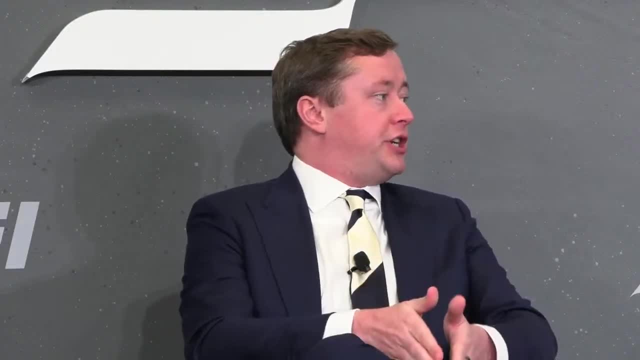 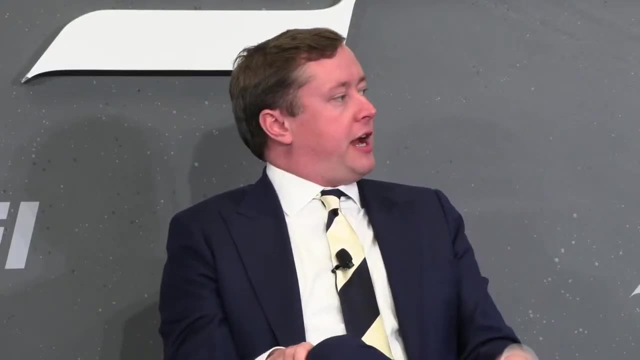 from the traditional voice in Washington is right. We see technology every day that is a decade out from patients and it provides a really unique and interesting perspective. but also it is a little bit scary or a little bit different to explain to someone on Capitol Hill or a regulator. 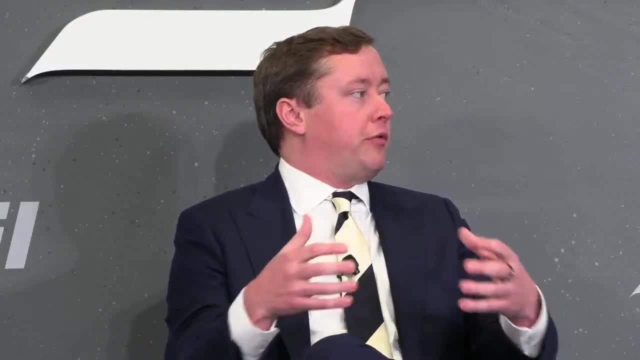 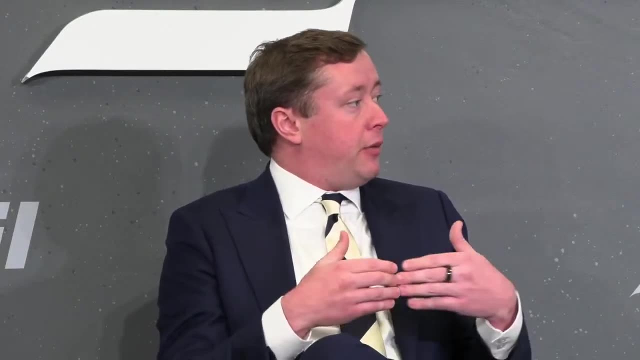 of what the idea of an AI co-pilot with every physician or provider looks like and what that potential impact could have for the lowest income patient populations, And that's the area that we look at the most of like. imagine a world where we have a patient. 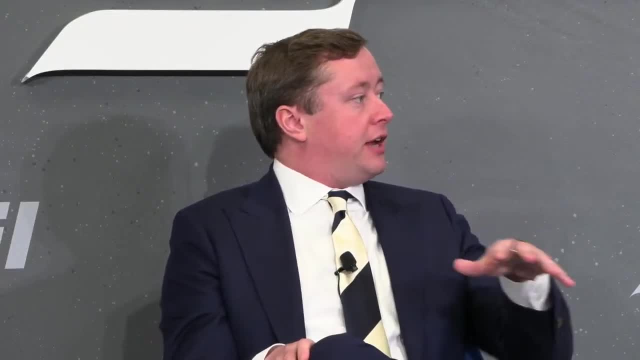 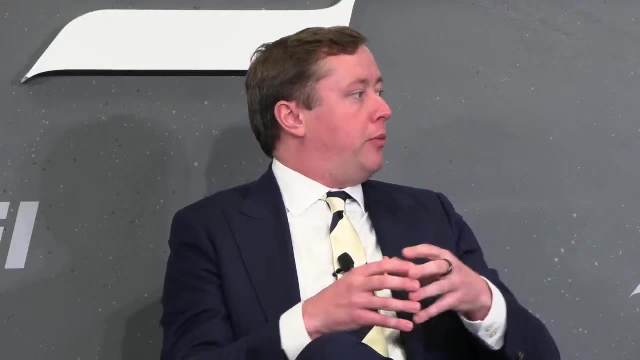 or a system where every patient has access to not just a provider in the rural or underserved area, but in their pocket or with them at all times, is the highest level, most capable, most advanced version of technology that can assist them throughout the whole process. 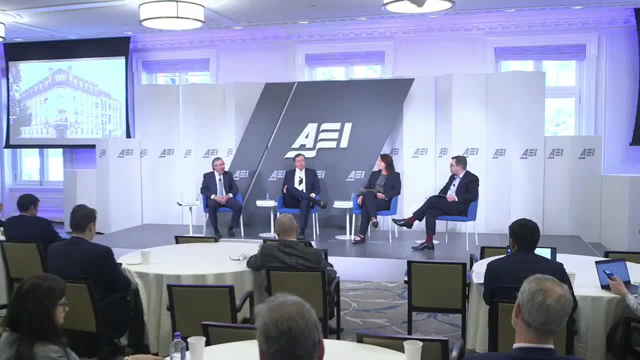 And customized to them personally. Yeah, And listen, I think that's. the holy grail here is, if you're delivering objectively better outcomes with lower cost to deliver, that's the opportunity, And with the labor force is what it is, then I'll just share. 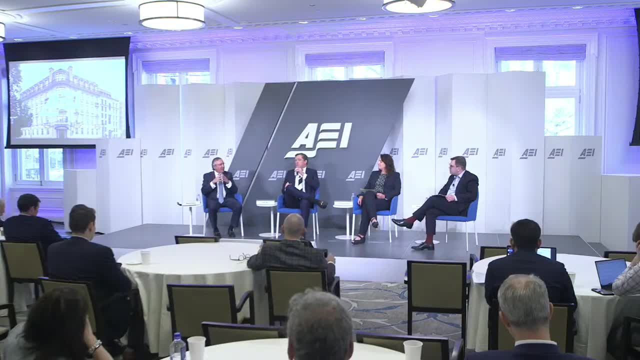 you know one example, A recent memory, in the last 10 years, you know, there was a medical device cleared that automated the delivery of anesthesia in the hospital setting The anesthesiologist did not. it was safe and effective by FDA. 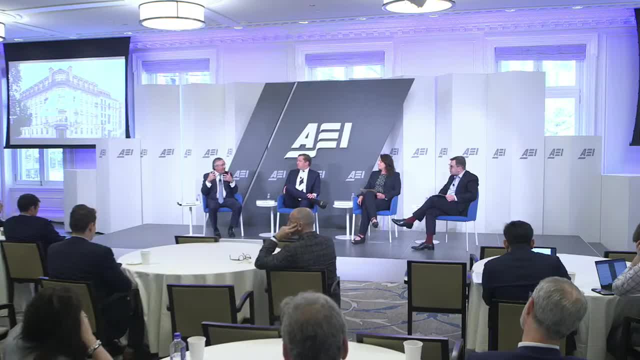 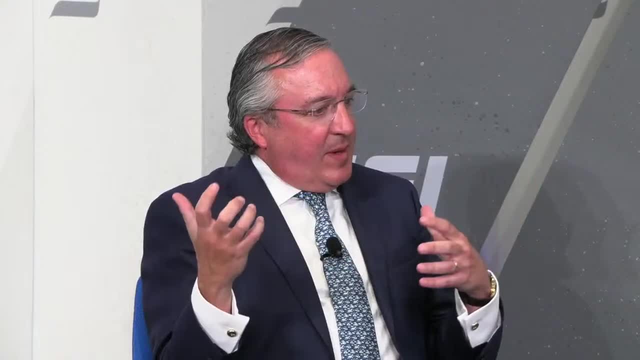 but from a market adoption standpoint it faced real challenges because it was displacing labor And I think you know our members are looking right now to how does this help inform the physician and the delivery of care. You know, what you're talking about is downstream. 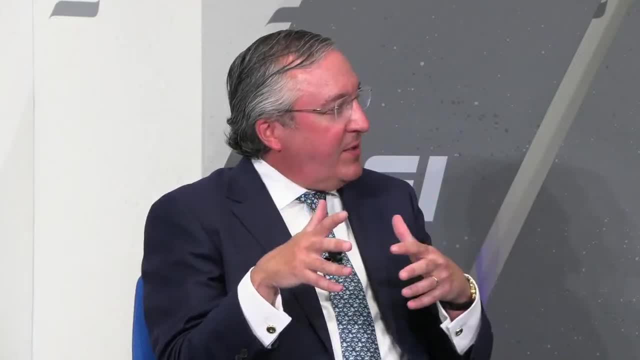 We want to get there And again, I think it's going to depend upon what the technology and what the price point is. Yeah, I mean I have two high schools and two school daughters now, but when they were little we had great health insurance. We had primary care docs but we went to the med clinic because I'd rather pay 60 bucks out of pocket get those tests done, And so I think there are absolutely models that have worked for the right. you know tests and others. 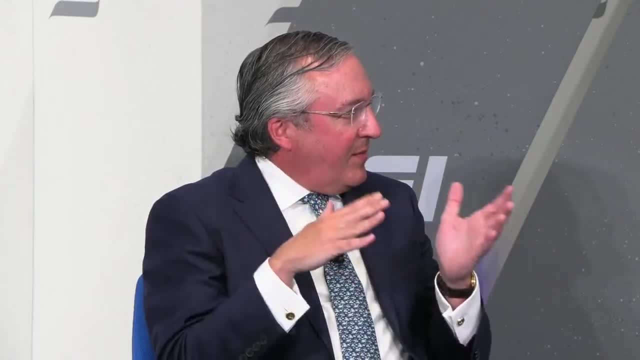 that the out of pocket is going to be fine. But as you go up that kind of severity of sophistication it's going to be cost prohibitive probably to do that And I think one of the things you know CMS has done this. 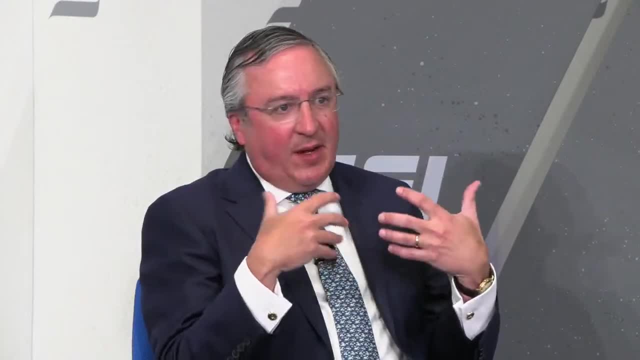 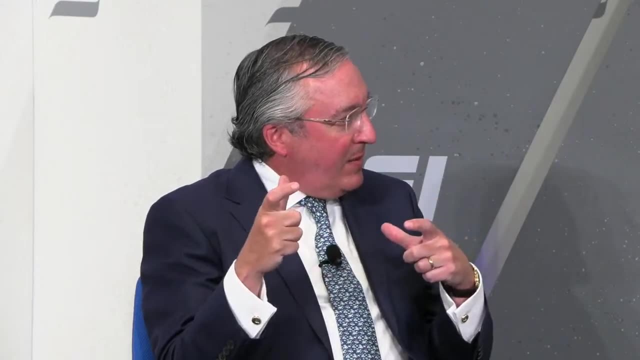 on onesies and twosies, when there's been technologies kind of primarily AI based in medical devices, And I think one of the things that they've done is they've done a lot of research on the technology side of things, where they have rewarded the value there. 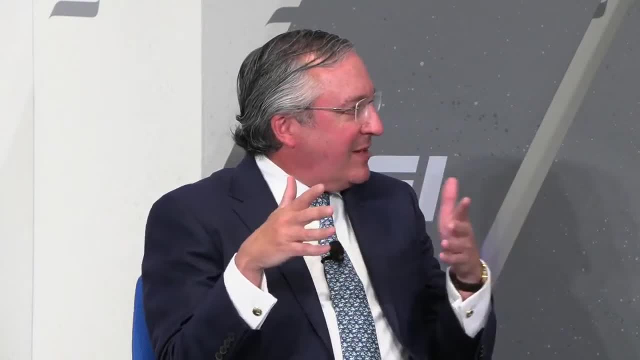 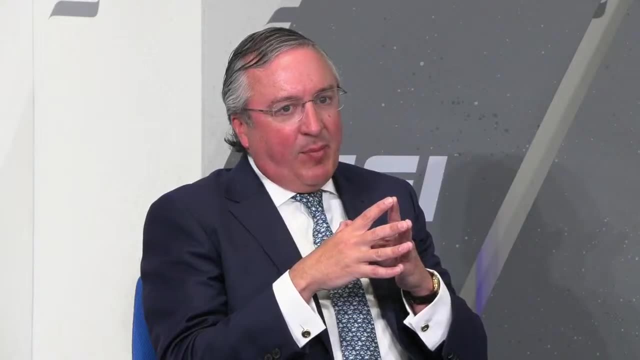 with the new tech add-on payment. But again, once that that lasts for about three years and then you're kind of lumped into an existing DRG usually. And so what can be done that properly incentivizes technologies that maybe not have the same labor intensity to it? 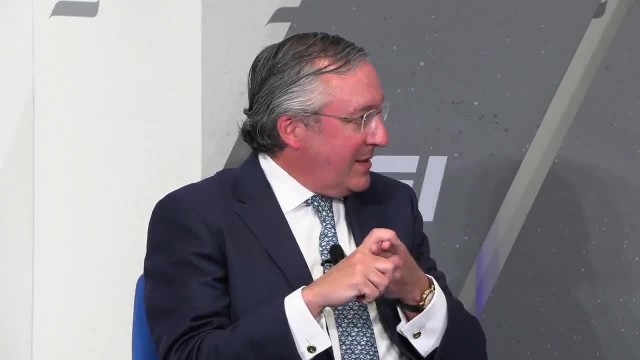 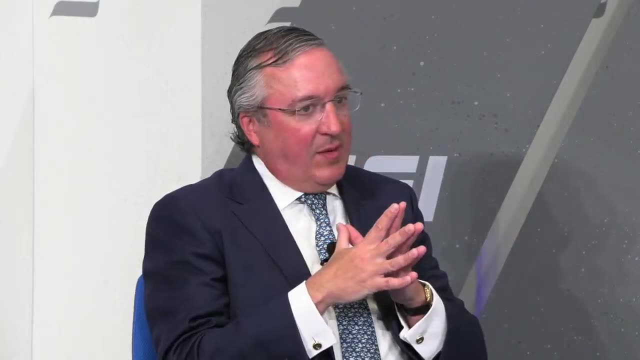 but there's significant investments on the technology side, on the data analysis side, on the computing side, that accurately rewards that value. And so the question is: what can we do to make that value in the marketplace? Because you know, unless and until, we kind of think. 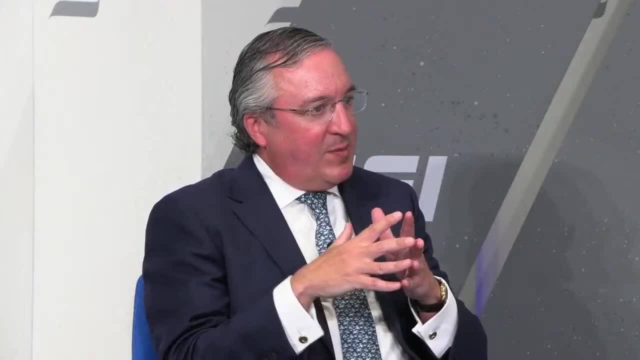 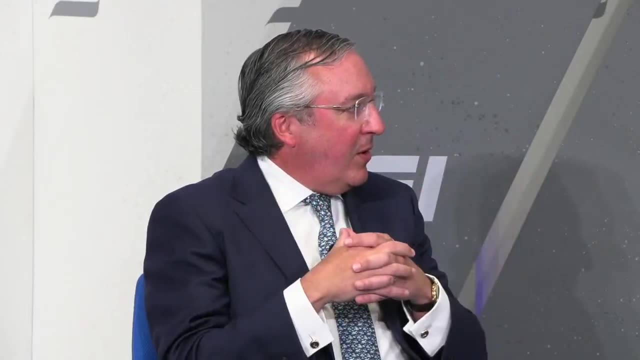 and again, this is not going to be done tomorrow, But you know, having this conversation, I can tell you if you get through the regulatory process. but if you don't have that value associated in the marketplace, none of your folks and none of the VCs are going to be putting. 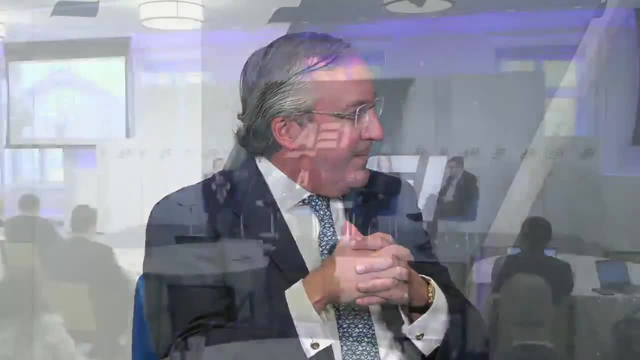 money into it and therefore they'll all go the way of the dodo and we're back with the same healthcare system we have today. Right, And I think the thing that at least I've always thought about with technology and healthcare is: 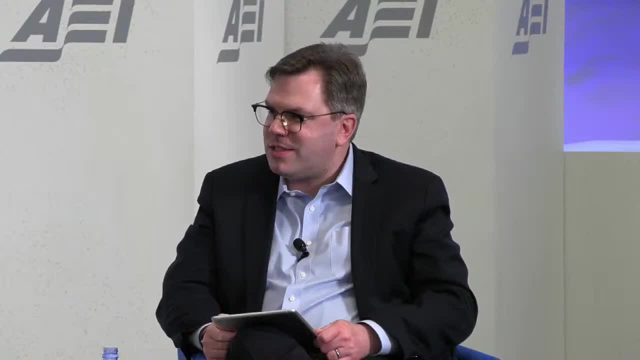 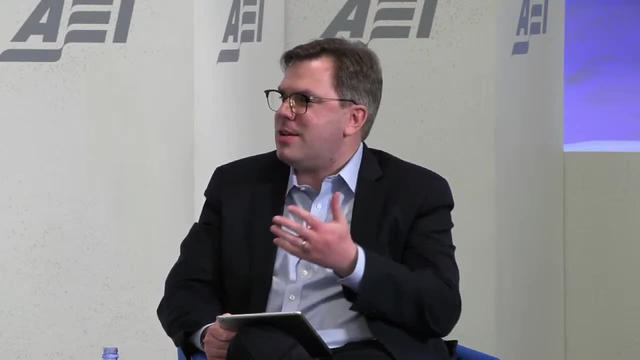 is that people don't realize that the current purely human system in many circumstances can be highly unsafe. right Like patients don't see those bad events that happen. There are bad events that happen every day in hospitals across the US and it's not. 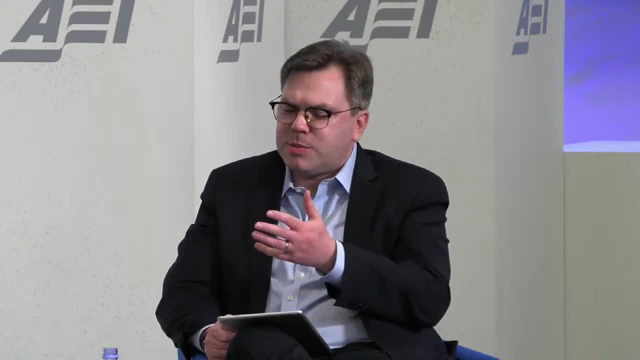 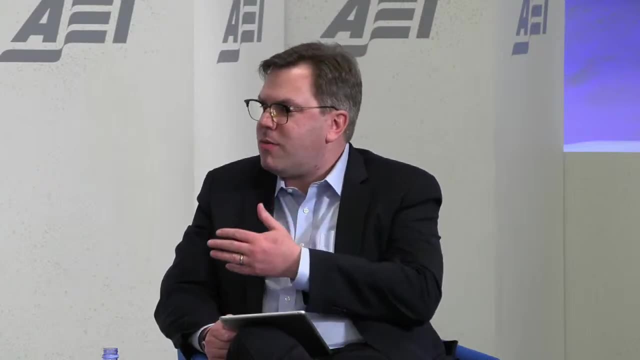 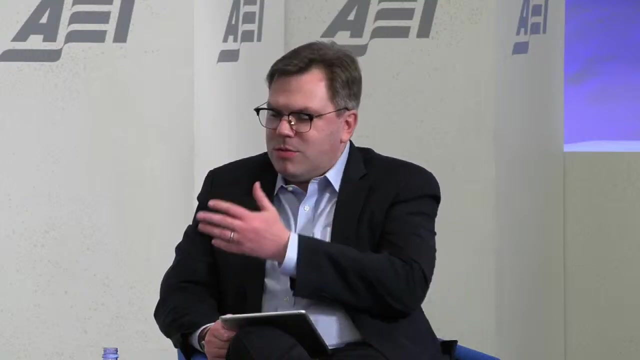 because doctors are bad people or nurses are bad people or hospitals are bad companies, Like there are good clinicians, good staff and good companies trying to do a good job, But when you have 1,000 tasks that are manual, cognitive, procedural, process, just by chance. 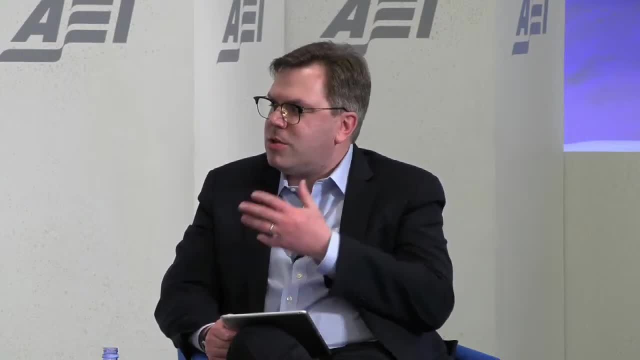 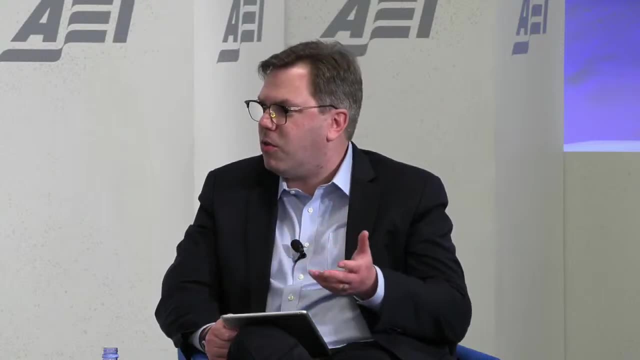 alone, some of them are going to go wrong, And so if we can automate some of those tasks and decrease that cognitive burden to allow the staff to function at a higher level and be more efficient and effective and safer, right that will be better for patients. 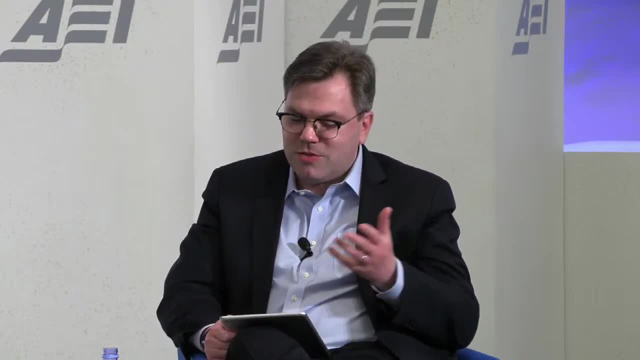 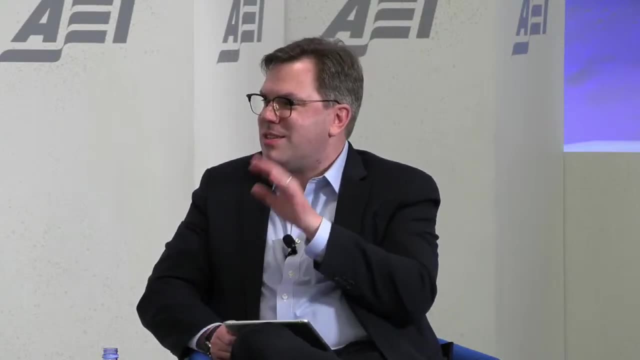 Like the average. you know there was a study in JAMA Internal Medicine a few years ago And you're like why is he citing academic literature that no one cares about? And they did a time motion study of internal medicine residents who spend a lot of time. 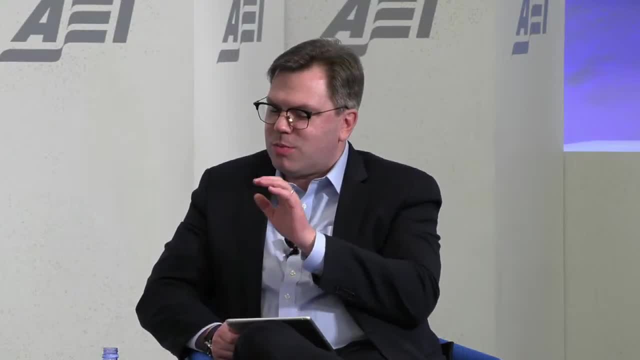 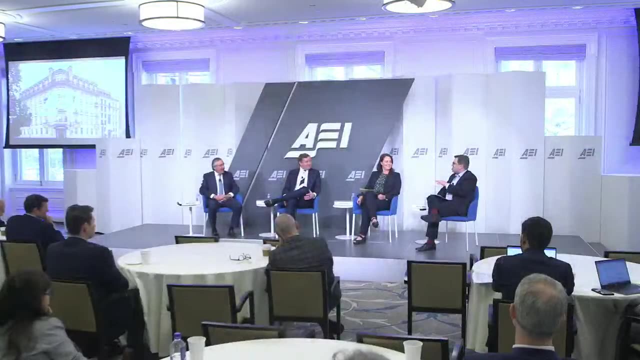 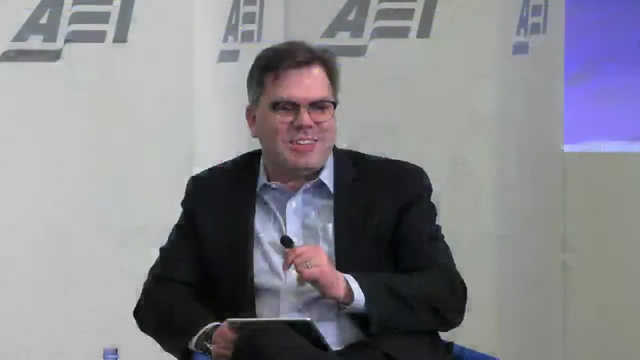 in the hospital, like 80 hours a week. Anyone guess what the percentage of time was spent on direct patient care? 25 minutes, 15 hours. Out of what percentage of time? 20. 13. 13%. So if you're spending 13% of your time actually talking to patients who are high, risk who are hospitalized with serious illness: cancer, pneumonia, blood clots, alcohol withdrawal, whatever it is. that's, by definition, probably not customized and personalized. It's not because the doctors or hospitals are bad, It's just because the system is designed to make them do everything. 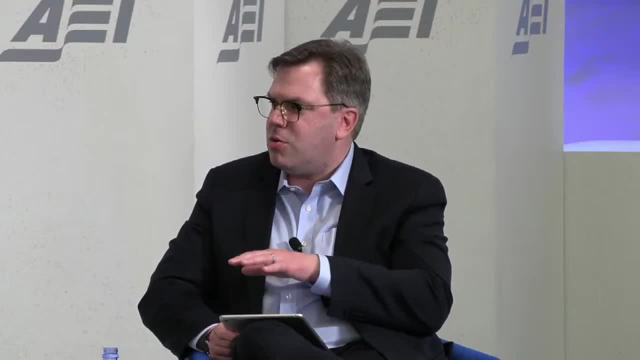 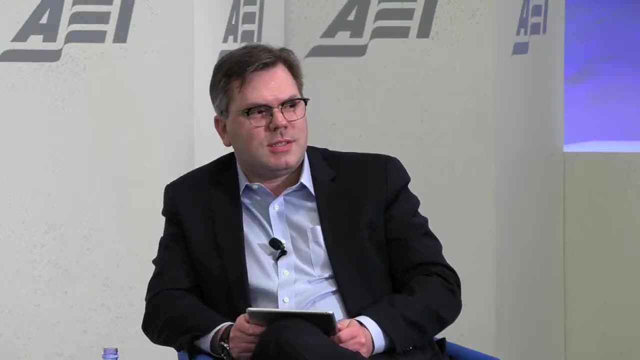 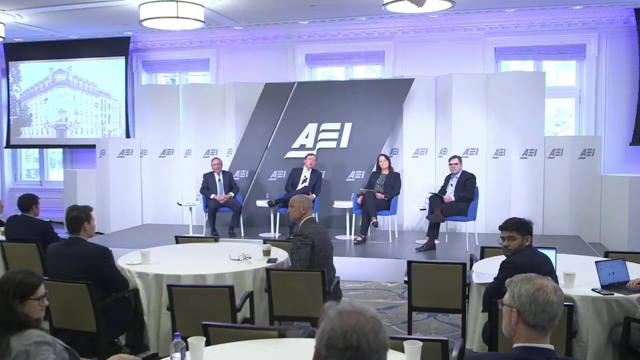 So automation and AI in medicine has huge, enormous potential, And with that, I'd like to open it up to questions. This is a great conversation. I appreciate you all doing it. I'm Carl Polzer And background: I work on a lot of issues now having to do with low-income workers. 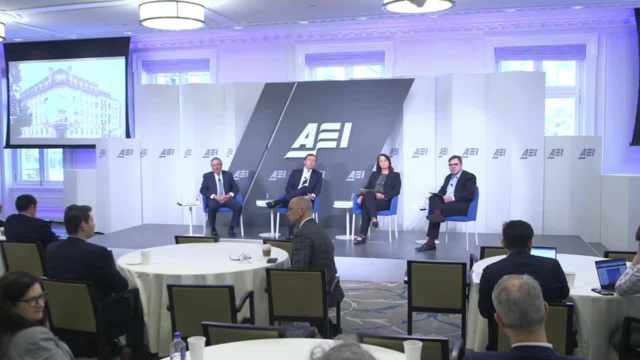 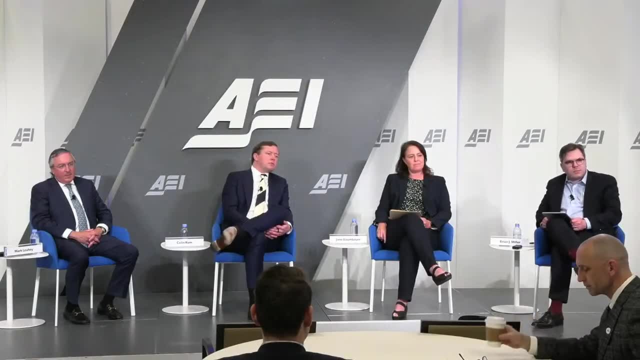 But my background relevant to this is I. for 10 years I was the head of policy for a major assisted living association here in town. So a couple weeks ago there was a front-page article in the Post where AI used by three major assisted living companies was forced upon, allegedly. 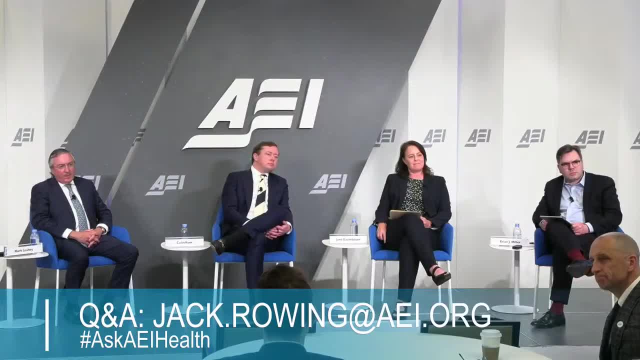 facilities and substandard care occurred, and now they're all in court, okay. So my question is- it has to do with: can you can a machine build? I mean, all these machines are coded by people, The codes are developed by people. 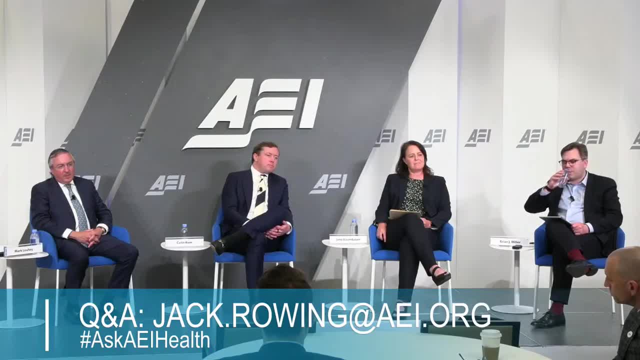 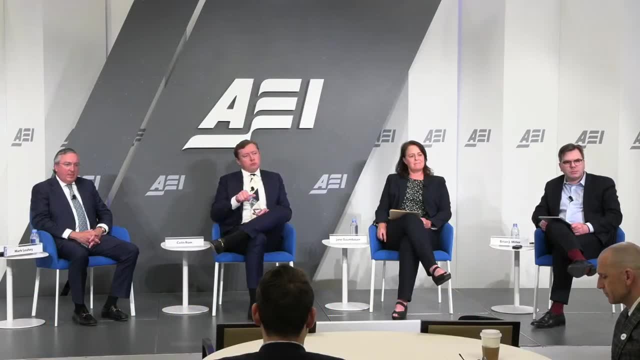 The codes are authorized by people and they're applied by people, So there's human interface at all phases. So when these, is there a whole like cottage industry being developed? now, when these cases go to court, In terms of what you're talking about, 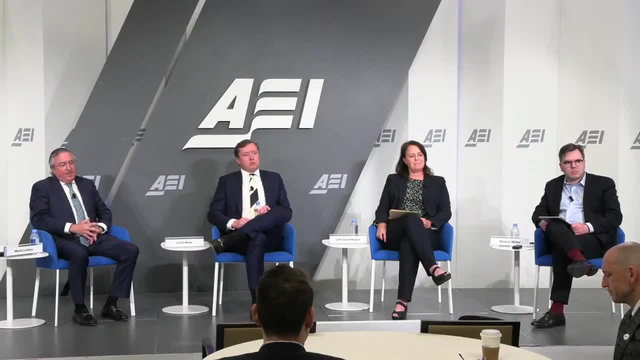 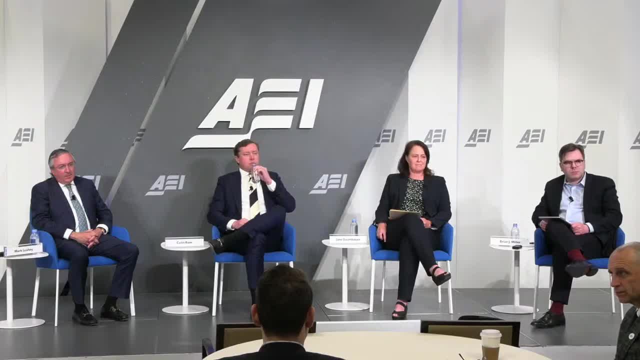 the 맛 fáins about how the AI was developed, applied, etc. I just wondered about, and for the purposes of regulation, what kind of documentation should be required and made for regulation through the company And accessible in in regard of who did this? 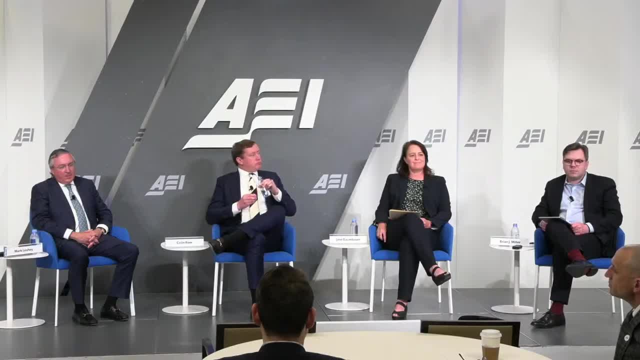 What is it? What is? how does the machine work? Who is responsible? Does that make sense? Well- No, no. Yeah, I guess. maybe that seems more like the administration of healthcare. Yeah, I guess maybe that seems more like the administration of healthcare. 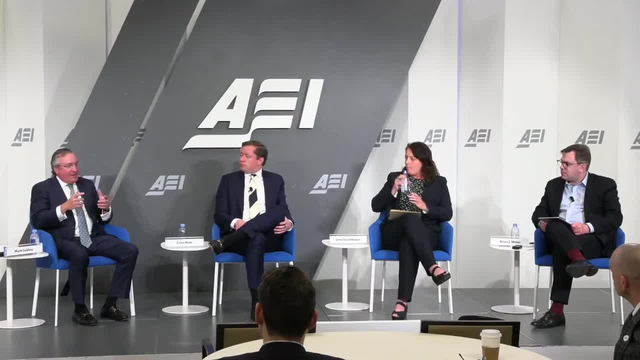 So the our devices are going through this facetious division, through and they're getting authorized and again a lot of we hear about ai is garbage in, garbage out, but again we're. you know closed system algorithms, you know very tight screen. fda is reviewing it. so i think from the device stamp and this, this seems like more of administration. so i'd 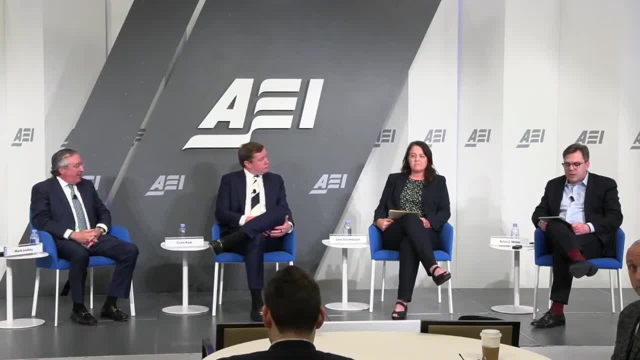 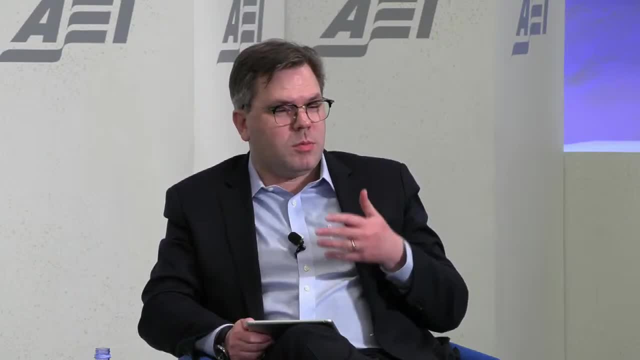 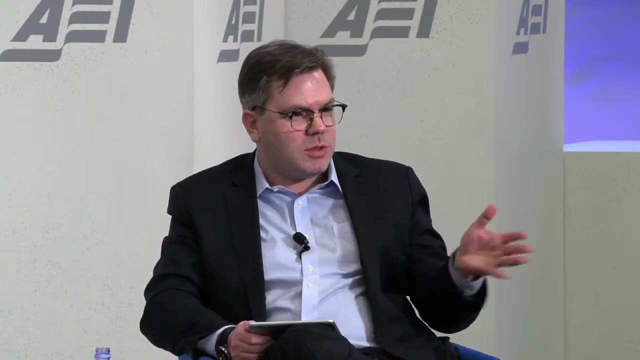 say this is probably outside the lens. yeah, i mean thinking, putting on an administrative hat, if you think about it. so tools, processes and people are put in place. there are systems that are put in place by people, used by people. they have a process by which the people who are working- 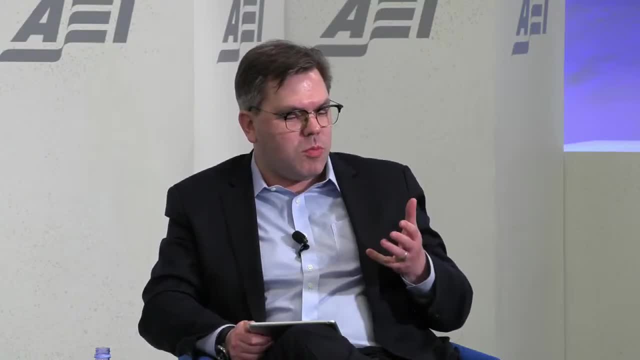 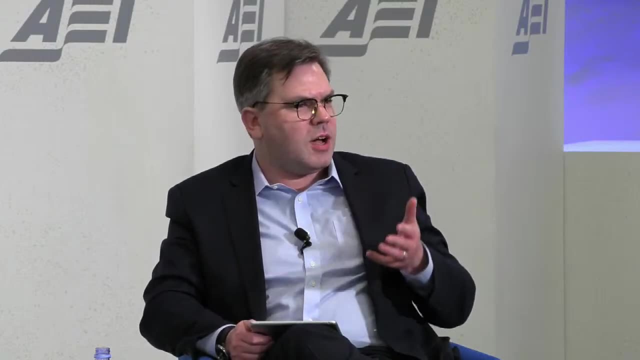 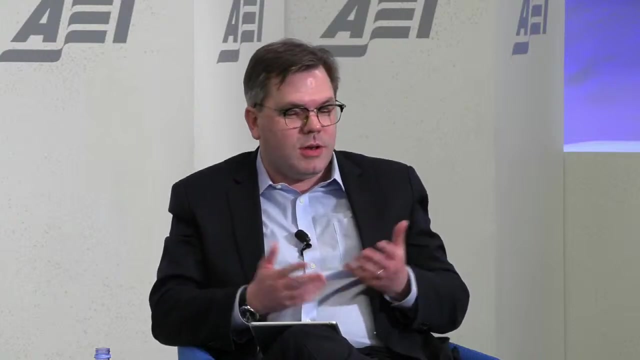 in the facilities have to use that technology. if the people who put the process in place made a failure of judgment, there was not enough autonomy and downstream in order to question the technology, or they were. the technology itself was not appropriately designed. like any of those elements could have gone wrong, i can't speak to. 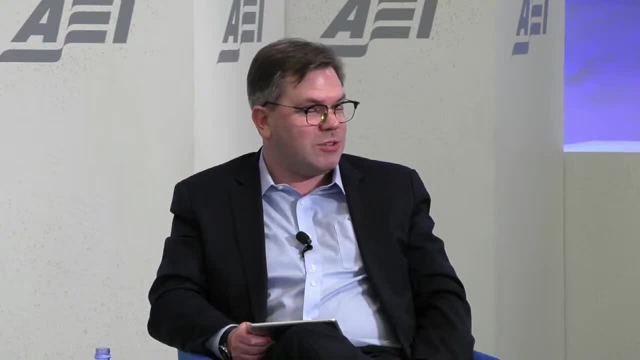 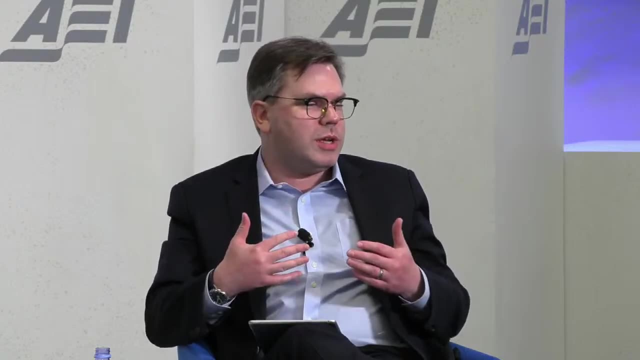 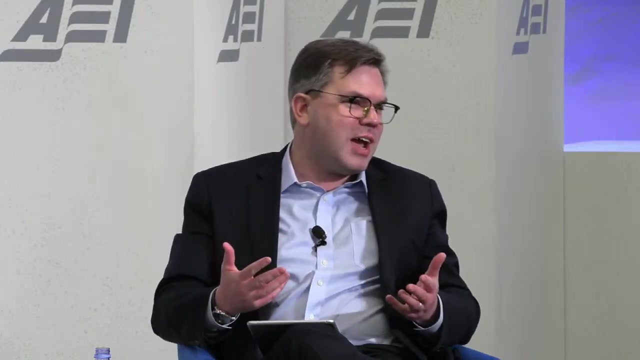 the, the, the specifics, but it emphasizes the fact that we still need humans. so even if we automate lots of processes, there's still a huge place, an important place in medicine, health care, writ large for human judgment. we're all still going to be employed. we might be still doing slightly different tasks. 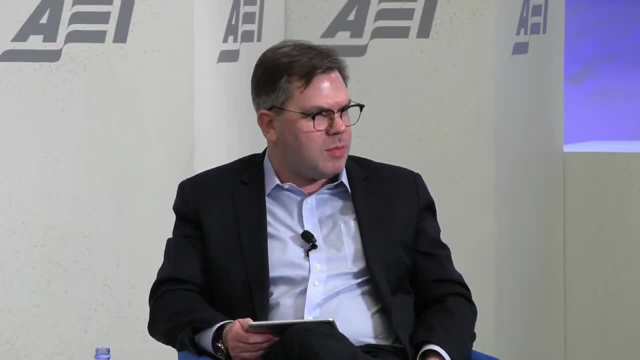 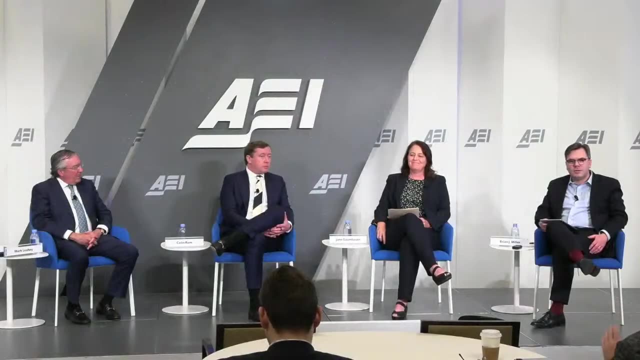 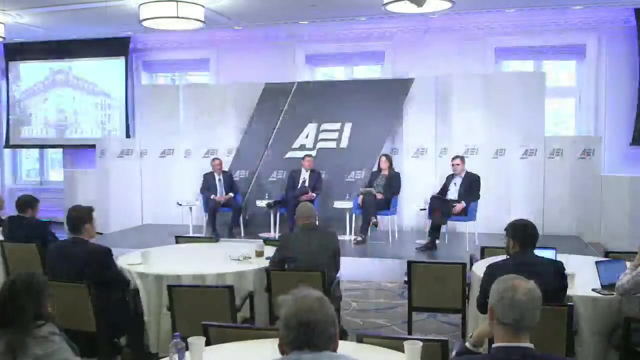 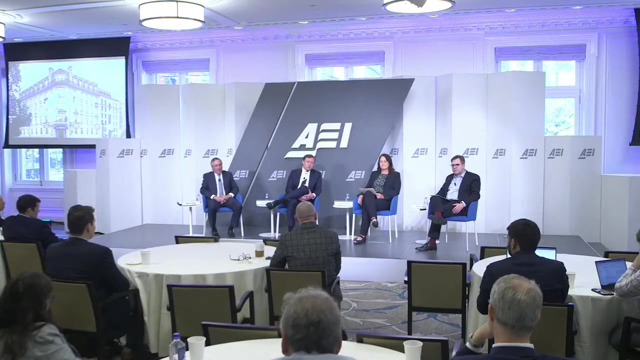 but it sounds like that's a case where there may have been a management and process issue. good question, this is a question for for colin, but i'll weigh in. um colin i- i believe i've heard correct me if i'm wrong. i believe i've heard your principal, mark andreessen, talk or advocate for an open. 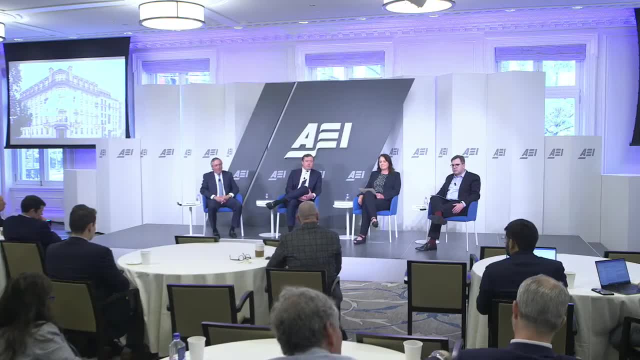 source approach to ai. yet the products that we're talking about here today- you know, life sciences, drugs, devices, diagnostics- that you're clearly investing in- typically get the most out of the world and the most expensive products in the world, but usually get developed in a very proprietary. 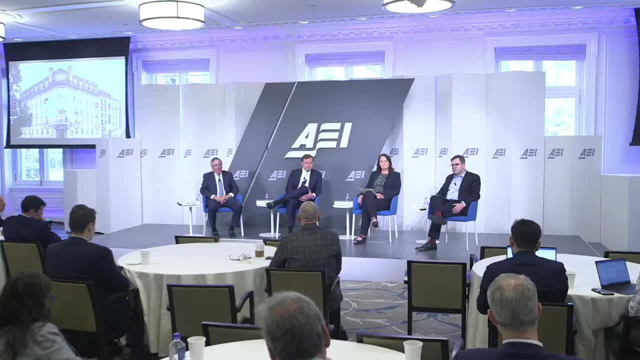 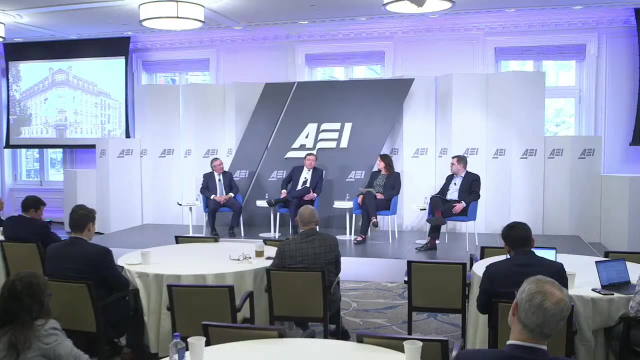 fashion. you know exclusive licenses, um, you know proprietary, know how carefully drafted patent applications that don't lead your competition to you know the crown jewel of your technology. so on its face, that seems like an inherent, unbridgeable gap. yeah, talk, talk about that a little bit, sure, so. 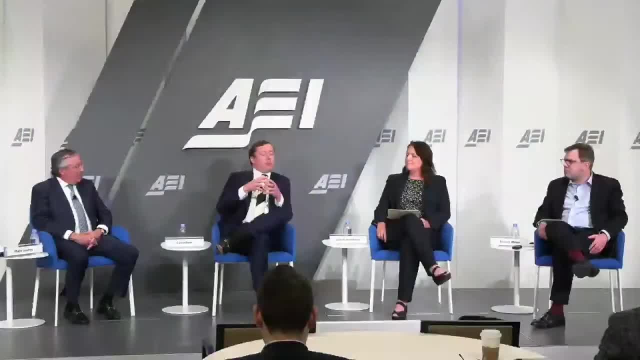 i think there's kind of two ways to look at it. i think the broader thought process that we're having across sectors, not just in the healthcare space specifically, is that a lot of the conversations that are coming from regulators around, or not regulators, but rather some of the bigger 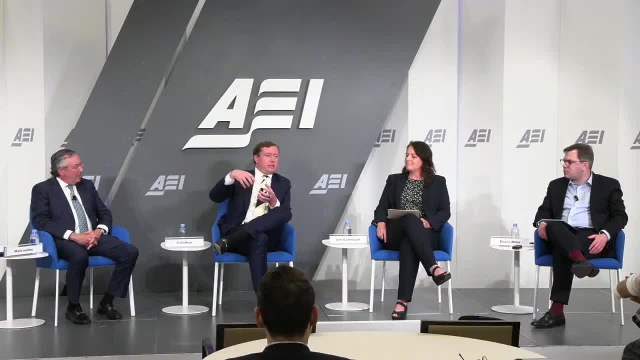 tech companies are. everything should be closed source because the idea of access to these large models, it could get into the hands of the wrong people. These things might create a system where there's a different level of fairness or bias, And I think Mark's thought process around this is putting these things out in the open. 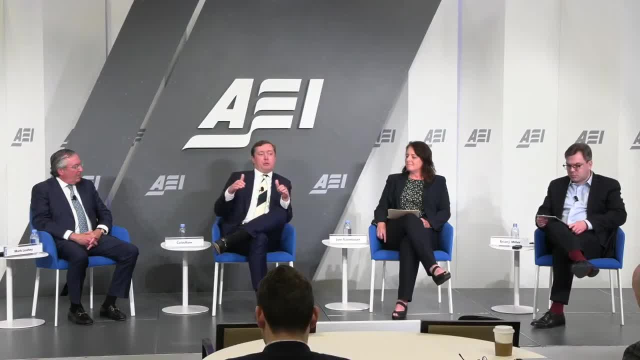 allow for organizations and different tech companies to be able to basically regulate and keep track of one another in a way that they would have certainly more expertise than any organization in the federal government will be capable of Now. with regards to the applications in healthcare, it is a little bit different to your point. 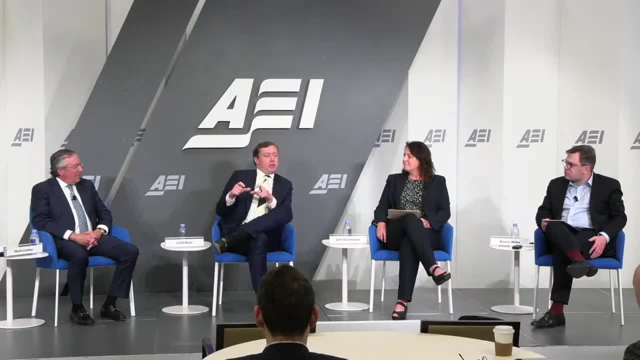 and I recognize exactly where you're coming from. I think the way we're thinking about it from an open source perspective is largely for the applications outside of the healthcare sector, because of how they carry health data, HIPAA requirements and things like that. 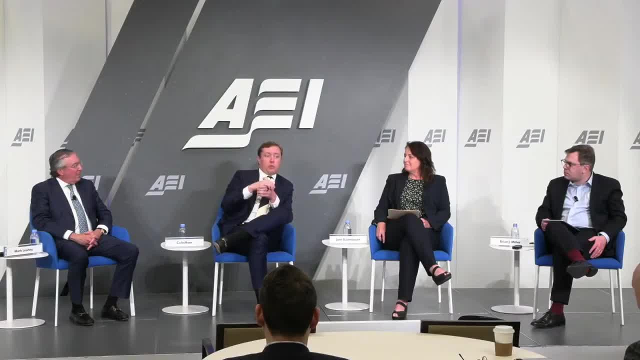 So that's been. I totally understand kind of the difference, but I think with a lot of it. some of the conversations we've had with some of the big research institutes also apply, though, to open source in terms of there's technology that helps determine or look at different. 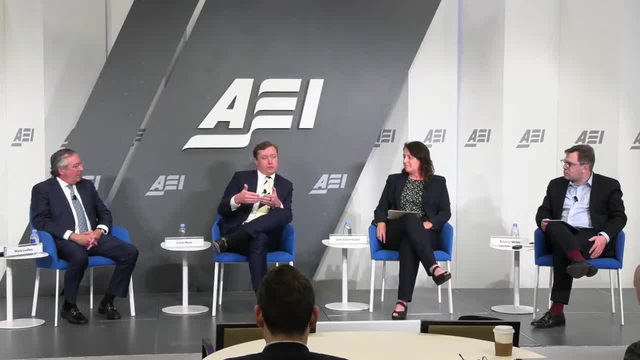 ways that proteins fold and how those could be applied to cell or gene therapies, or even how you could think about how certain cell or gene therapies work directly with someone's personalized genome or what that looks like. So sometimes those models are actually shared between research institutes, and that's something. 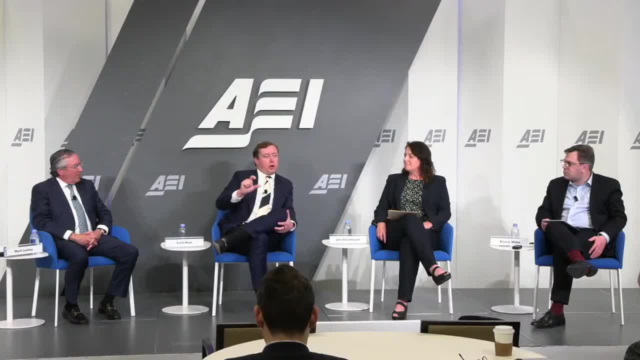 that we're very much in favor of, But some of it is just like smaller applications versus these big, almost enormous LLMs that have access to the entire internet, for instance, and how they're trained. So it's dependent on the application largely. 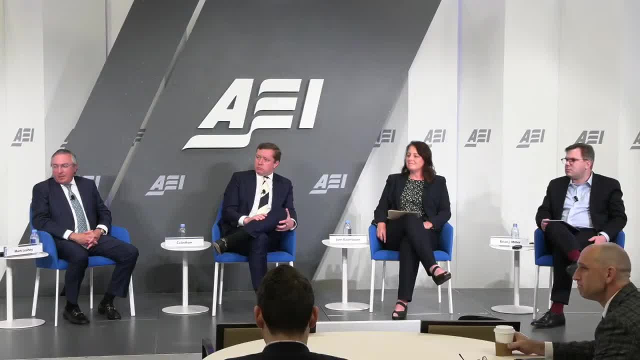 JP Hogan, I'm trying to figure out whether this is more a drone question or a first response, but in hearing this I'm wondering: are you at whether AI maybe could prescribe something that could be delivered by drone, but maybe it would be a limited like two- or three-day? 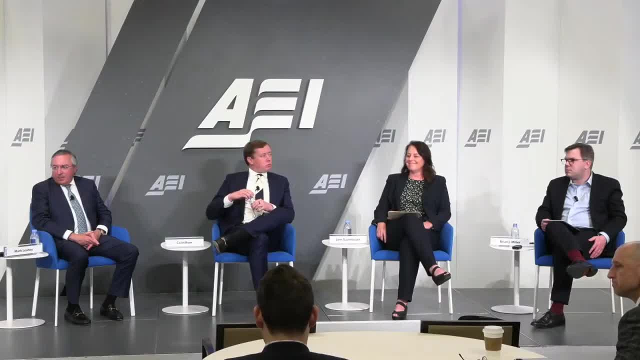 dose. So that's Yeah. I mean you can't have time to get to a doctor, So you have the rural, So whether that would go into, you get a couple days to get to a doctor, but you can get something. 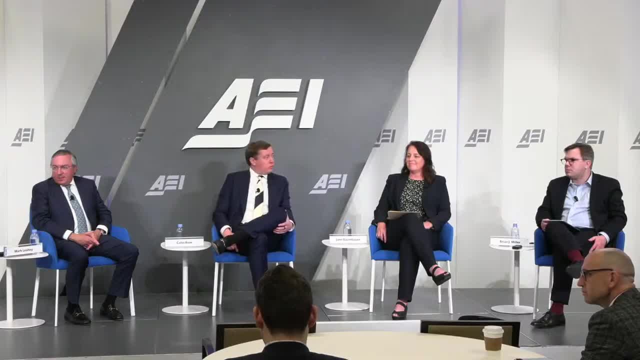 by remote drone or just wondering where some of that is falling, where the doctor would still be in the system. but you might be able to get something AI-generated for a day or two, if just as a fallback. So I'm just wondering if are the discussions already there for remote deliveries and emergency. 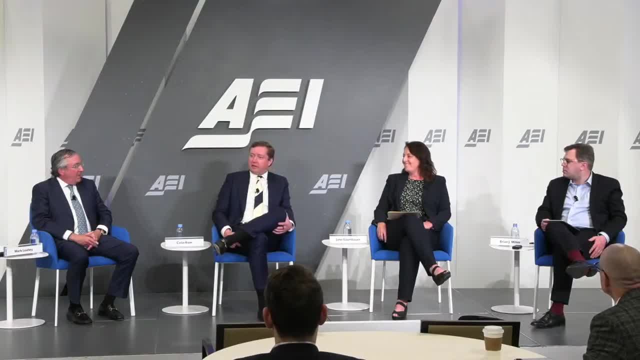 I can't speak to that. We haven't invested in anything in that space, but that's certainly something that is interesting that we can look into. I mean, I think there would be a scope of practice like: can the machine practice medicine? 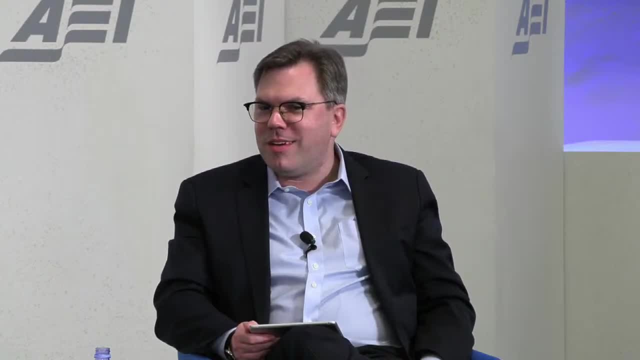 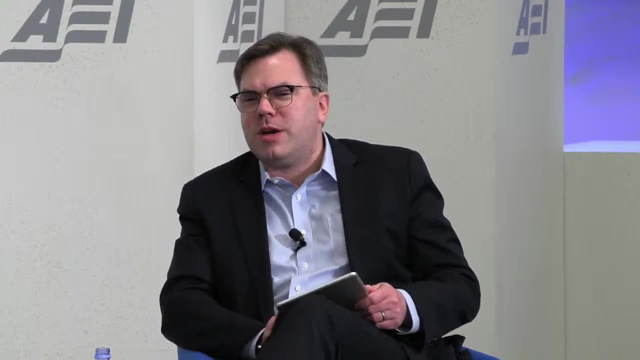 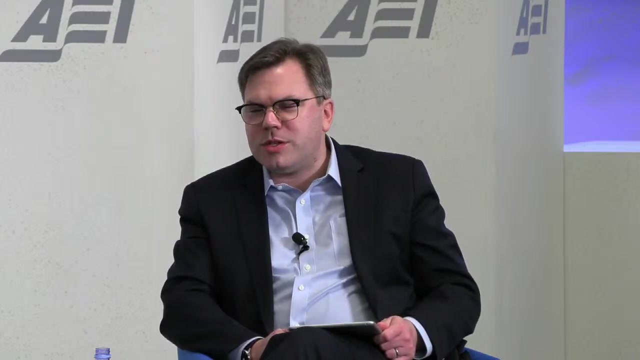 I am obviously not a state medical licensing board, nor would I want that job Sounds stressful, But you can imagine. eventually it gets to the point where technology does have some scope of medical practice- A limited scope. The question of course then is: where does technology and FDA regulation intersect with? 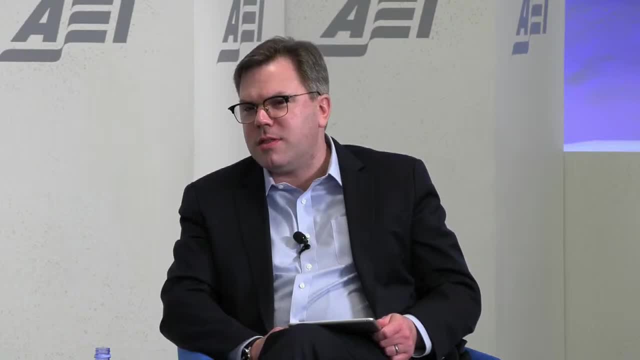 medical licensure for autonomous care. I don't think that that question has been answered by anybody. It's an important one, though, because you could imagine- maybe not today, but sometime in the not-so-distant future, years down the road- that that scenario could actually happen. 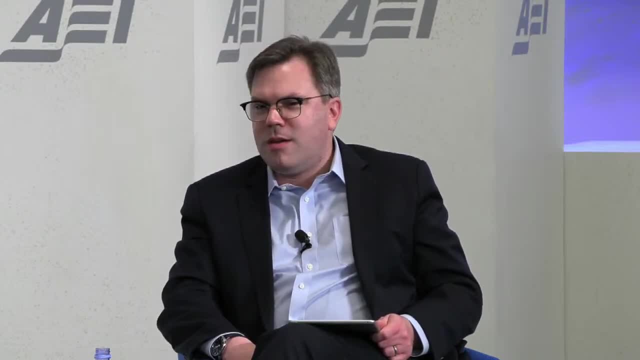 Right, Because, again, from a labor perspective, we're not going to be able to be training several hundred thousand extra- nurses, doctors, pharmacists, et cetera. So we have to think about ways to either augment and improve their efficiency or have a bridge. 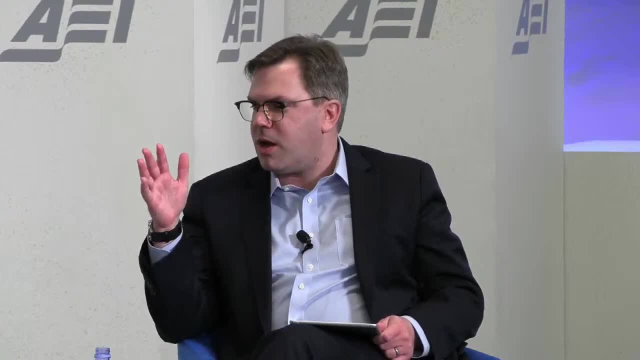 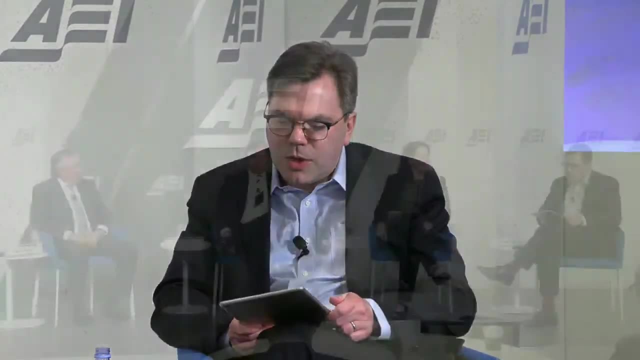 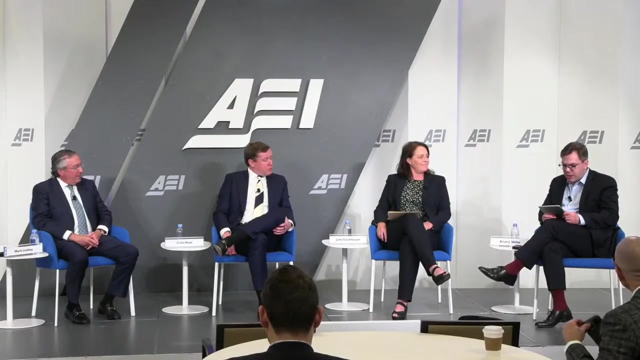 before people reach them, or upskill the doctor, nurse, whomever, and then have technology augment the rest. So another question that I was wondering about. well, I got a couple text questions here. One is OK. the question is: can we ask to discuss medical data marketplaces as referenced? 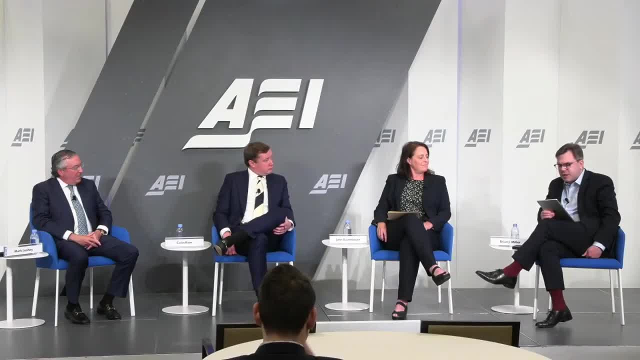 by ARPA-H and the FDA Specifically, how should these be rationally implemented to preserve privacy and also encourage innovation? And are there other examples of non-medical but regulated data marketplaces that could be considered DR? So I'm not familiar with that particular portion of the law, but I can speak a little. 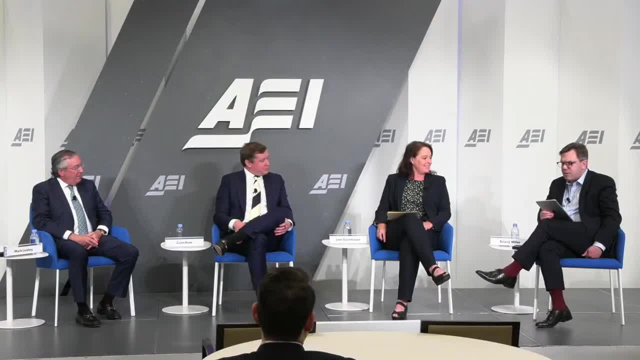 more broadly about health privacy- DR. Yeah, I think the question is about balancing health privacy and HIPAA with innovation and what happens when your data gets decentralized and put into essentially the cloud or a study pile, DR. Yes, You know, It's really sort of my entree into writing about health law at all. 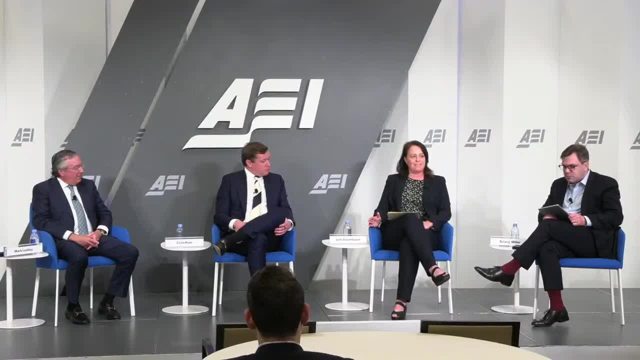 And you know it served an important purpose when it was developed. There was a gap in kind of basic confidentiality norms among doctors and clinics. that got, you know, sort of solved or, you know, HIPAA sort of brought in a new culture of being. 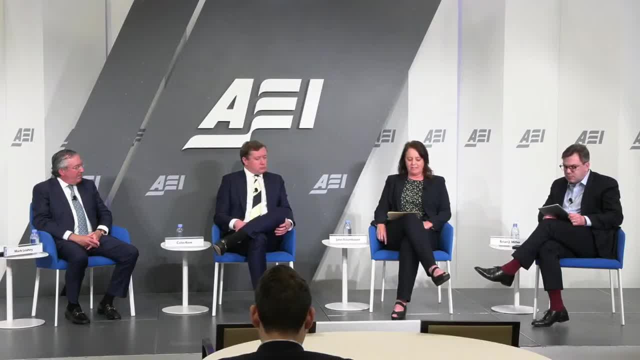 careful about discussing your patients and just sharing data willy-nilly, DR. At this point, I think it does more harm than good. So I think the things that HIPAA could learn from you know non-regulated or less regulated fields are, first of all, possibly reinterpreting what de-identified data means. 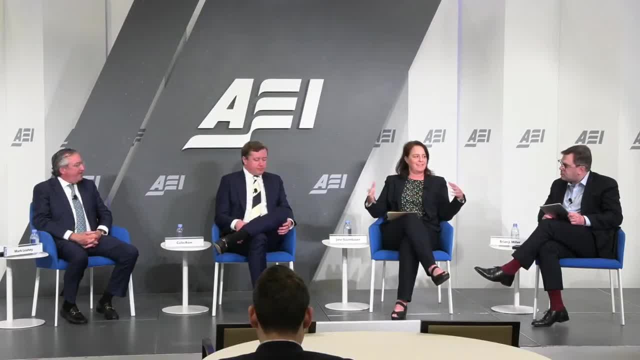 So that you know if it's de-identified data, then it can be shared and used and exploited for good purposes, research purposes and whatnot, And that maybe needs to be moved more DR, Right DR. I think it's more toward like a use or purposive test rather than a could, a bad. 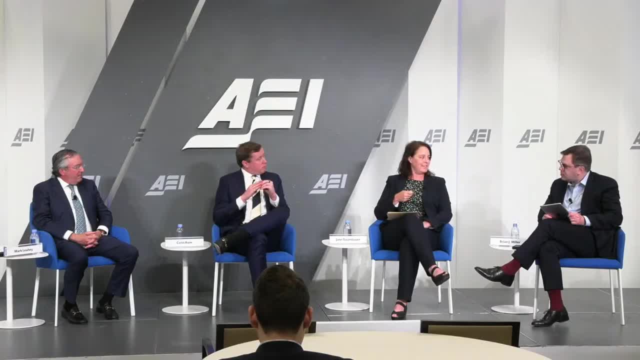 actor theoretically figure out which patient this is, And then mix that, of course, with access and security requirements and whatnot, And then, likewise, I think, the consent and control model of privacy will, I mean, especially if the de-identification problem isn't solved. 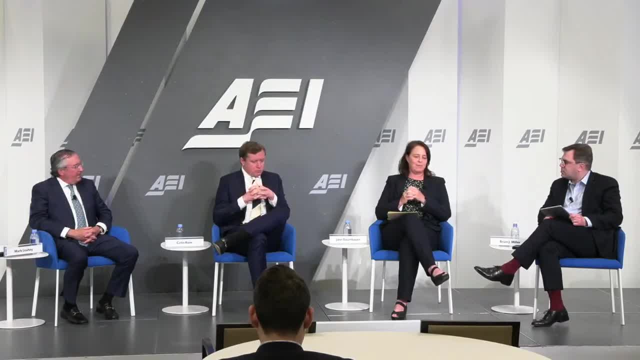 The consent and control model is just going to be too cumbersome. It either means that data is highly siloed and not being used effectively for lots of competing startups to create really useful health technology, or it means that patients will be constantly bombarded with permissions. 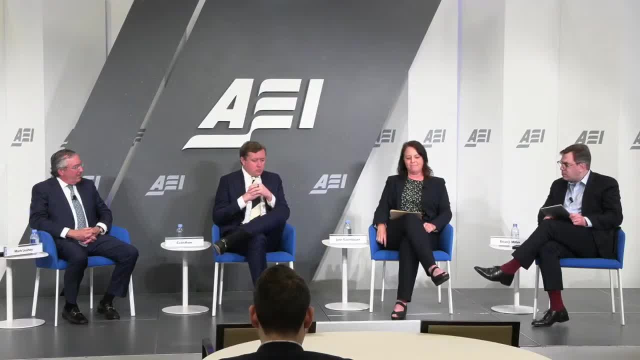 And HIPAA has also been a shield for bad, you know, has been a ploy Or a ruse for what's really actually sort of proprietary interests. So we were talking about electronic health records industries not being willing to make their systems interoperable and citing HIPAA as a justification for that. 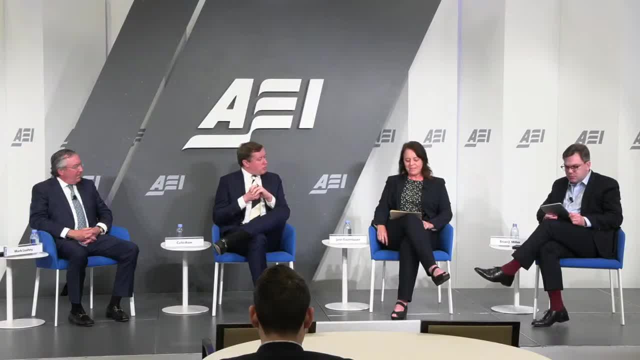 Hospitals, too, might have the same issue. So I do think it's time to move to again a sort of use-based, purpose-based, risk-based approach, That's, the approach to privacy. So I have two questions here, One of which is probably for Colin and one of which is for Mark. 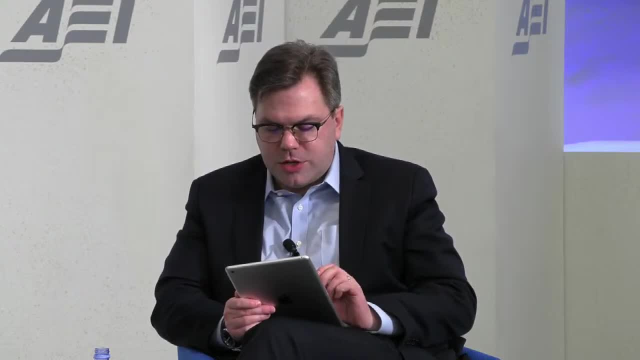 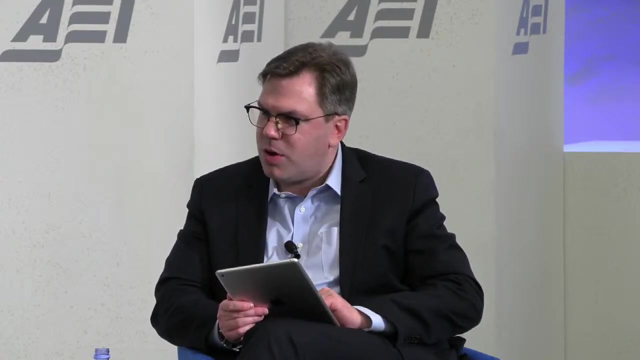 Mark, we know that EHR interoperability is a barrier to execution of AI-driven tools To some degrees. hospitals really want to capture patients' data and technology rather than promoting competition, innovation, entrepreneurship. What do you think that policymakers can do to combat this problem? 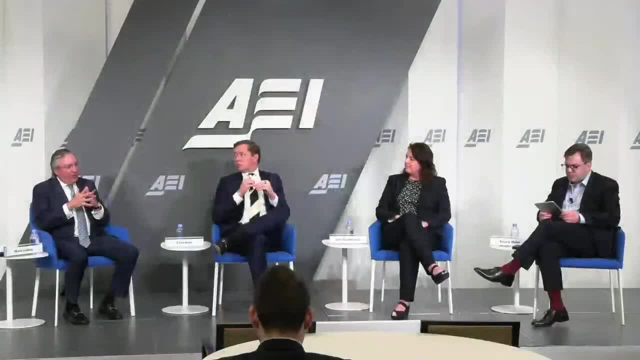 You know it's interesting because the question was set earlier about open source et cetera. I mean in the medical device space a lot of our companies have worked to make their devices interoperable with one another. You know the hospitals 10-plus years ago would show a picture of an ER with all the 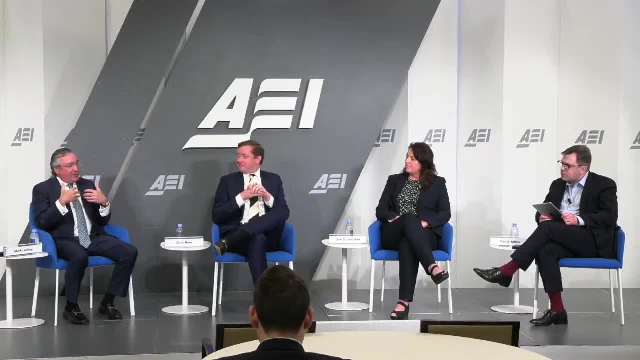 wires and saying you all need to talk to each other because this is inefficient. So our companies may have made great strides to make sure devices talk with one another- interoperable. But it was interesting We had a conversation with the hospital CEO saying, OK, well, we've done this to kind. 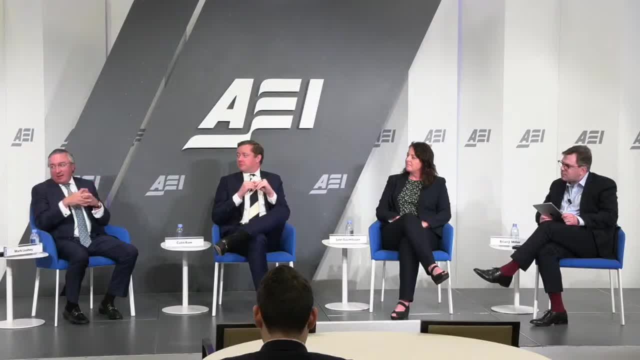 of meet your needs. Leveraging big data has been a goal for many for a long time. What can we do to make sure that your EHRs are interoperable at Cerner and Epic or even within one IDN and another? And it was kind of like crickets, because I think the reality is they don't want to see. 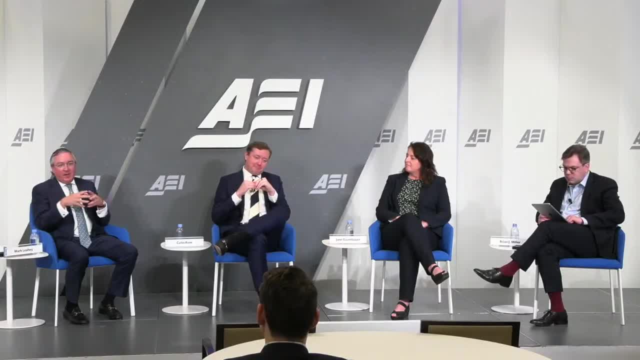 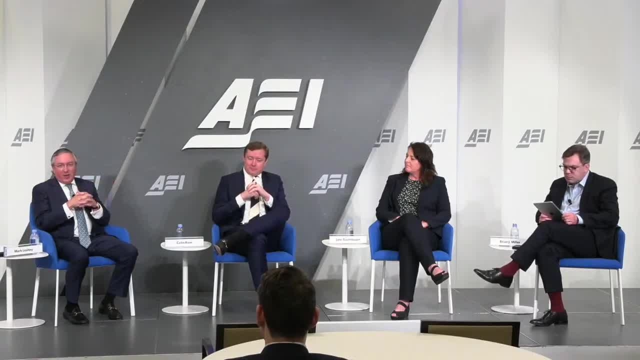 it's a good thing, And I think that's what Seema Verma said at a HIMSS meeting a few years back. Basically, it's the patient's data We're going to. you know, drive in that direction one way or the other. 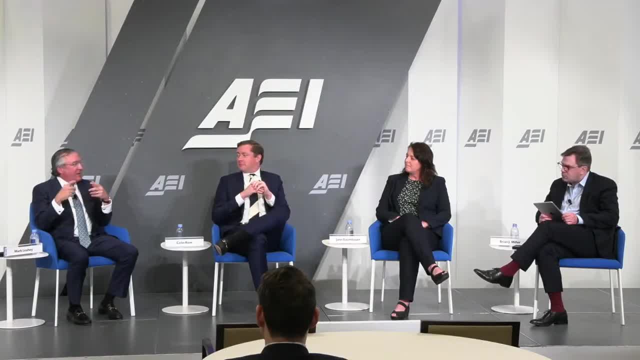 But for a variety of reasons, maybe HIPAA and others. I think there's a bipartisan interest to have EHRs be interoperable and leveraging that data in a useful way. But it hasn't got to the implementation phase yet And I think you know there are certainly tools in the toolbox if folks want to compel. 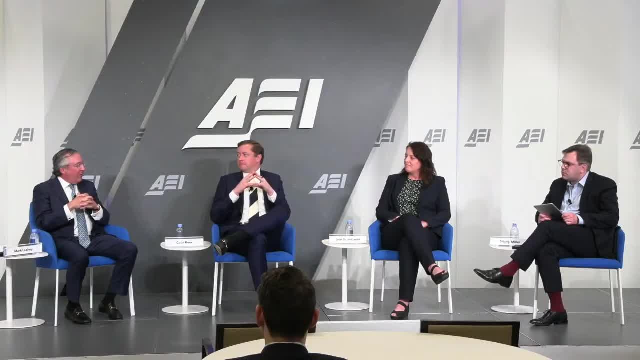 those final kind of locks to be unlocked for the greater good, But thus far we haven't been able to get there. Yeah, And I think that's also one of the to your point- one of the areas where open source in healthcare can be a real driver of benefit for accessibility for patients and accessibility. 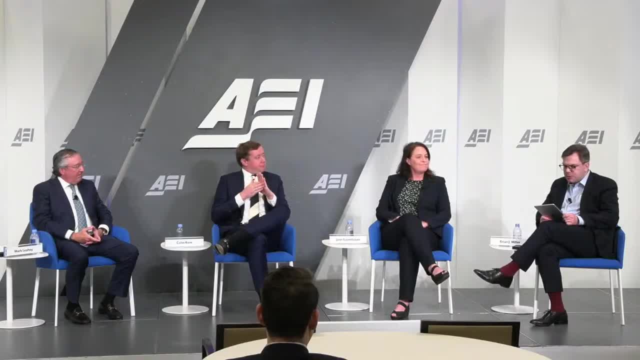 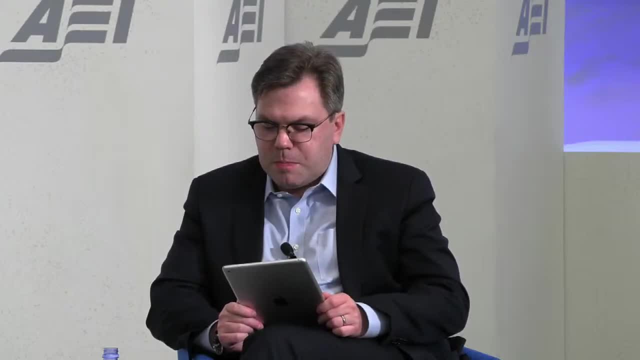 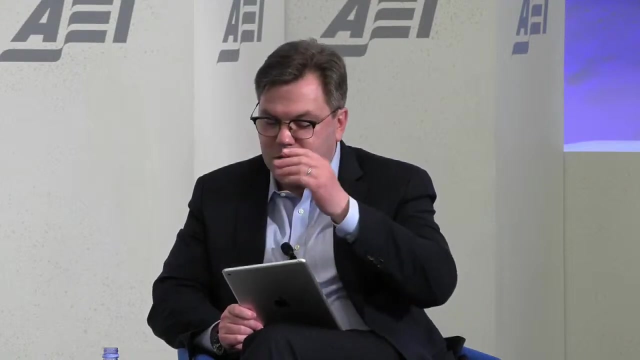 for their own health information. So two other questions. One question for Jane, Stipulating that someone develops an AI urgent care doctor that could assess less skilled practitioners Like nurse practitioners of physician assistants effectively, So essentially upskilling them into the full MD. 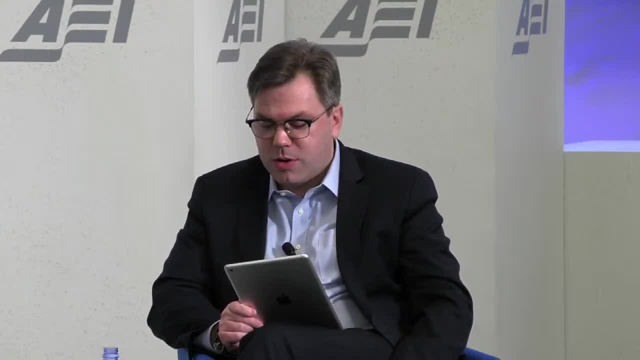 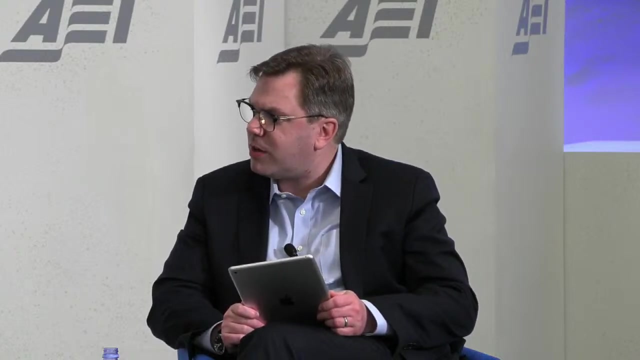 Something like GitHub's co-pilot for an NP. What are the existing regulatory requirements that they'd have to cross to market the model? And is this the FDA and then? or is this something that falls just on the liability of the practitioner right? 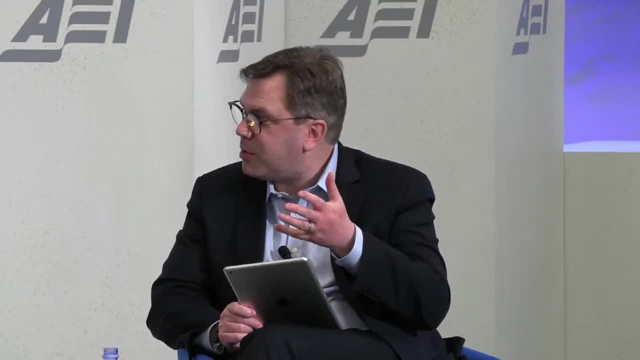 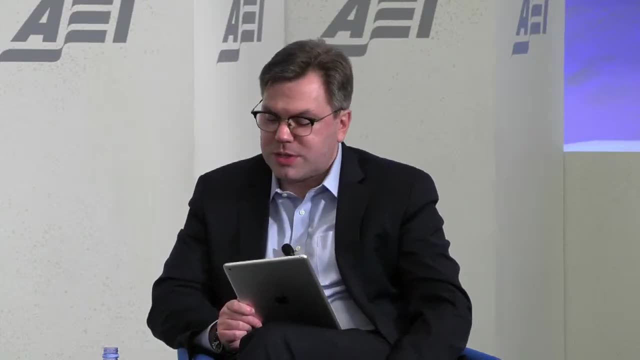 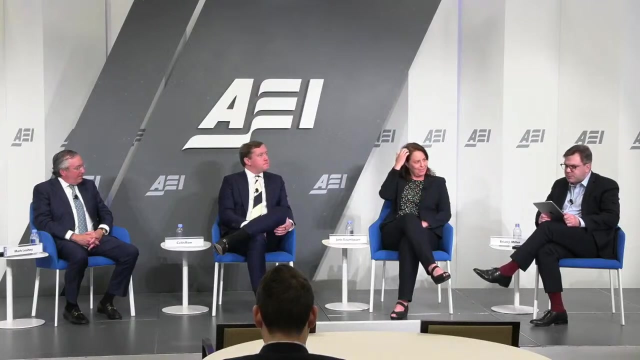 Does it go to the software manufacturer Or software developer in this case, And does it go to the physician assistant or nurse practitioner, Or is that to be decided? I think it's a little bit indeterminate right now for the reasons that you were teeing up. 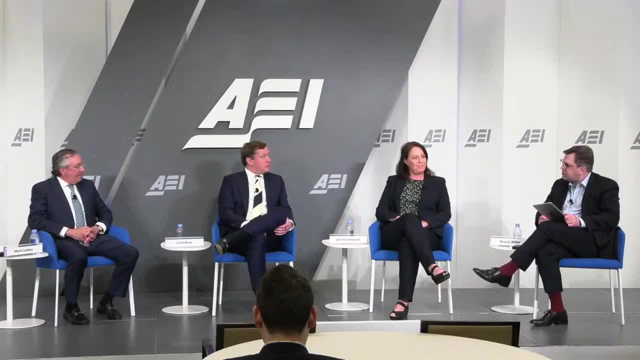 That, at least right now, if you go to a clinical setting, you are being seen by either a doctor or a nurse practitioner And in any way, someone authorized to practice medicine in the state, And so then their decision to use That software could be a source for a few liability, or it could be a hook for liability. 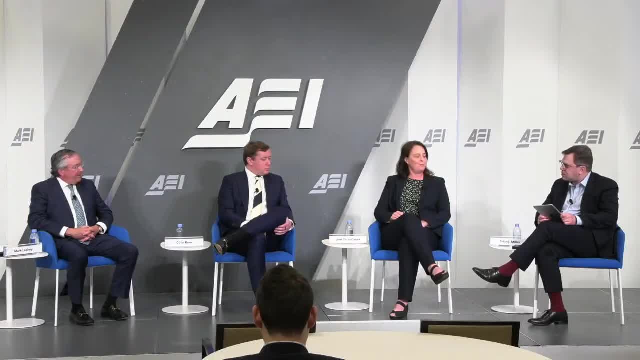 later, if they're harmed The product too. the producer could also be sued and would also presumably have to have already gone through FDA clearance. And so we're looking at potentially two layers of regulation. where, historically, doctors were, Doctors did not have to be regulated by the FDA, and vice versa in terms of drugs and devices. 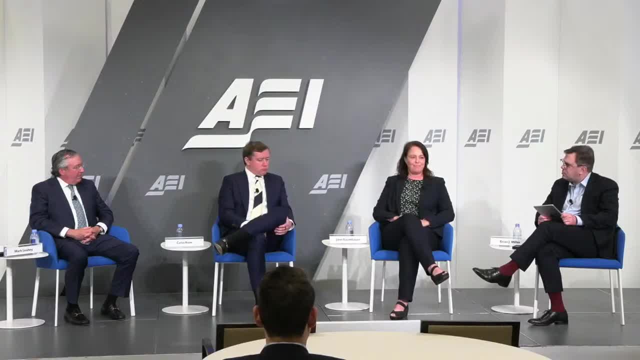 Of the two systems, for reasons that I've probably already made clear or telegraphed. I think the doctor approach or the state common law approach has actually honed more to the risk method and the X post liability method that I tend to prefer. 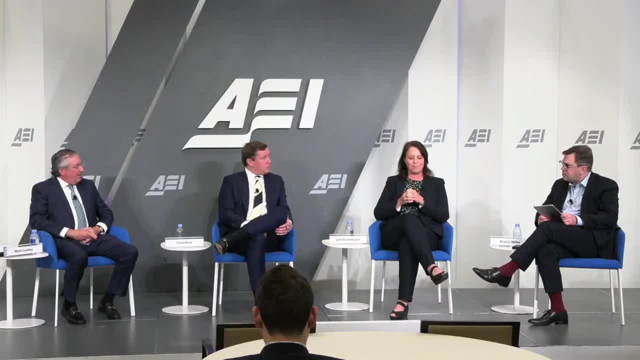 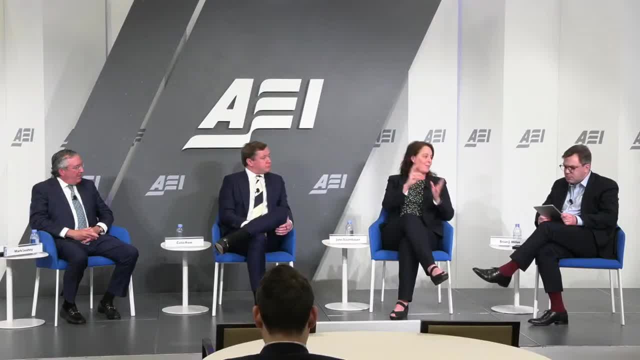 I think that's a good point. I think that's a good point, But it's not clear at all yet how. I mean- and especially once you take away the doctor- that the scenario you were asking about, where you have an in-home MD AI app or something, then we're really in unknown. 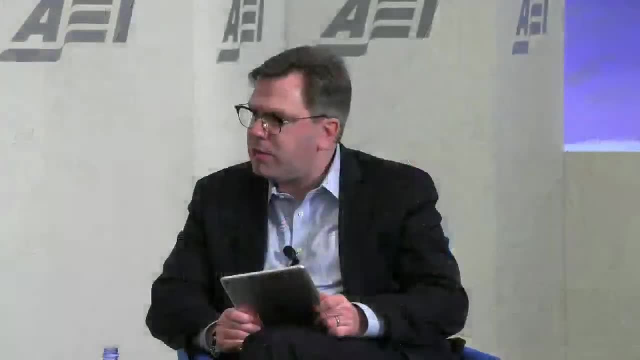 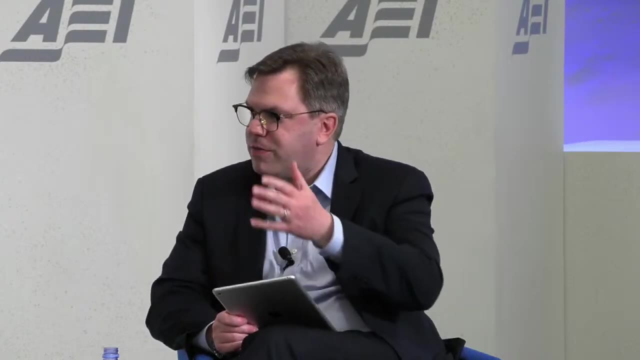 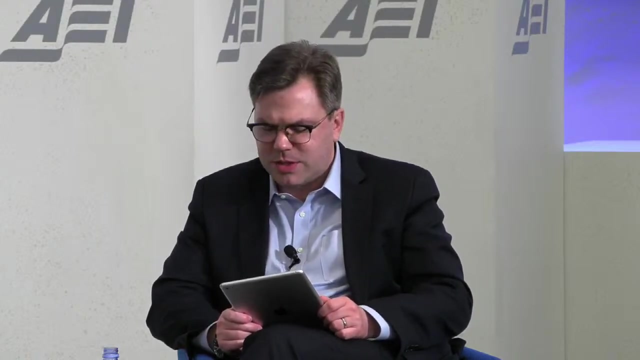 uncharted territory. So the follow-up question I think would be for Colin, which is: does that technology company need to run a study showing that this model- the nurse practitioner, physician assistant plus the co-pilot, Yeah- effectively matches the answer of a panel of expert docs presented with the same circumstances? 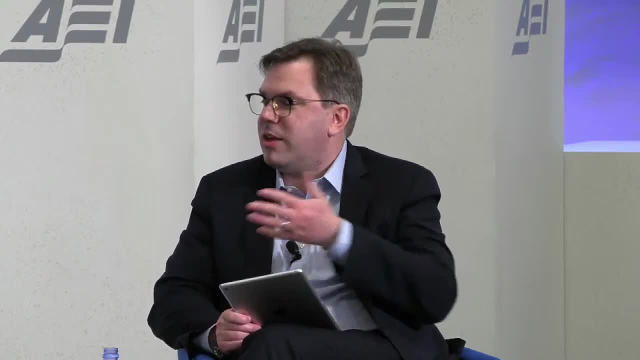 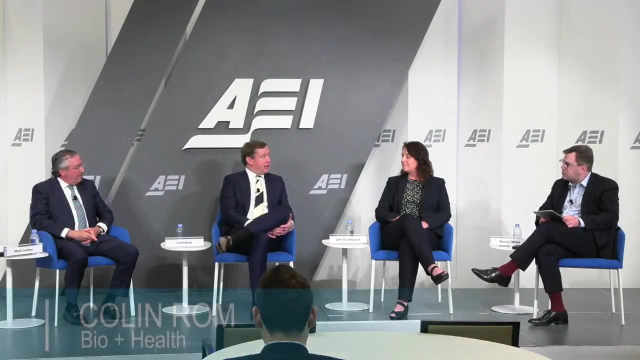 or sort of the evidentiary burden not clear right now. Yeah, I mean, I think one of the things that we've heard from a lot of both developers and then also regulators at the state and federal level is: what does the actual licensure or approval 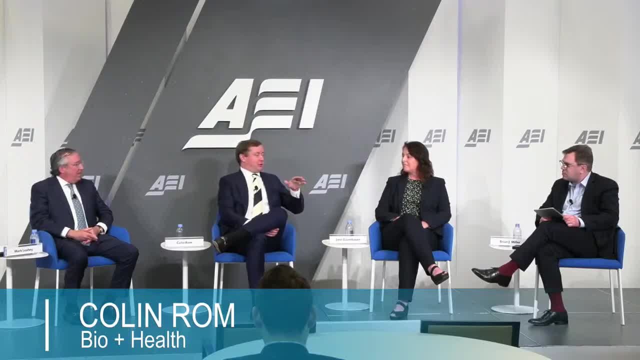 process look like, And especially if there's an idea of like there's a current regulatory structure. but in the event that there are technologies that can basically pass a licensure board, for instance, in every state, what does that look like? 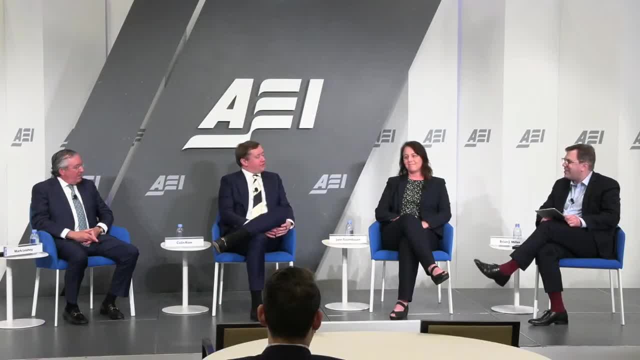 Right, I think it already could pass the USMLA, Yeah. And so there are a handful of JAMA articles that came out at the beginning or end of last year, beginning of this year, that were basically saying like here's what's happening. 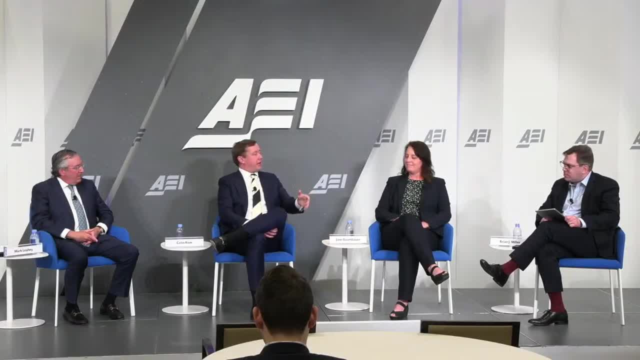 And these are models not specifically trained on datasets specific to healthcare and care delivery, So I don't think I havewe haven't figured out what the answer to that question is Until someone else goes to market first and deals with all these different regulatory. 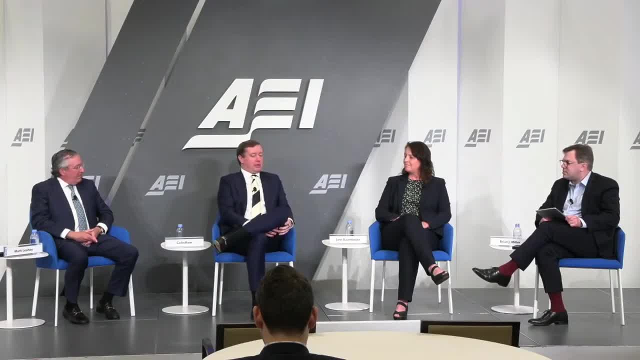 loopholes and hurdles and things like that. there's gonna be, Yeah, Somewhat of a disincentive to be the first to market there. I was gonna say thank God ChatGPT4 wasn't around when I had to take the USMLE, and then 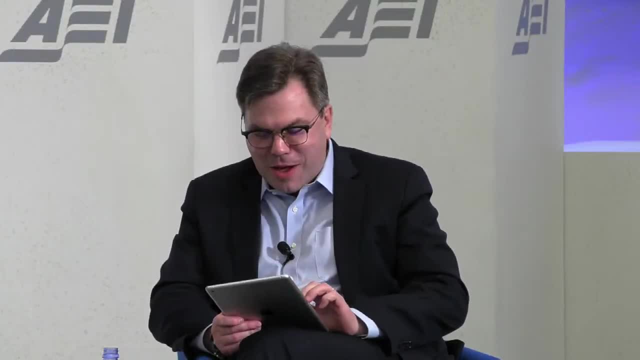 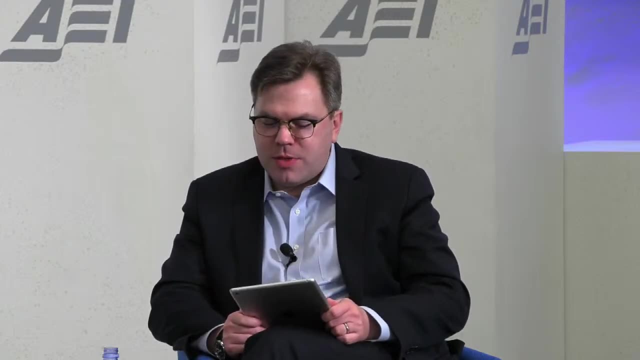 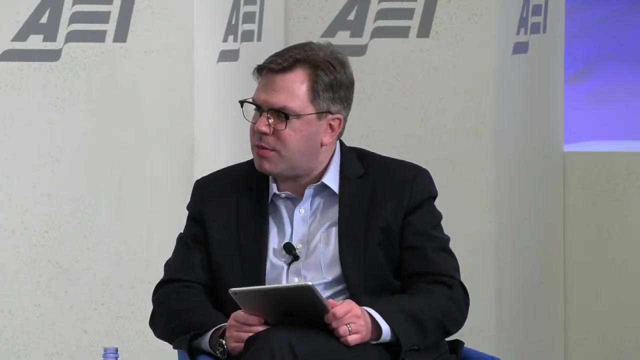 apply for residency, I would've been outscored. So one final question, sort of about FDA review. What do you think that we can do to use AI to increase the efficiency and speed of FDA review? or is this a pipe dream? 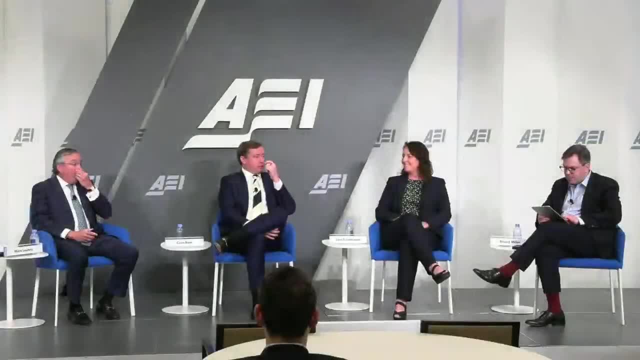 I mean personally. I think one of the things that comes to mind is It's basically creating uniformity in each of the medical product submissions, and I think that's been one of the things that Janet Woodcock has mentioned. right, Companies can submit their own, differentbasically their application clinical data submission. 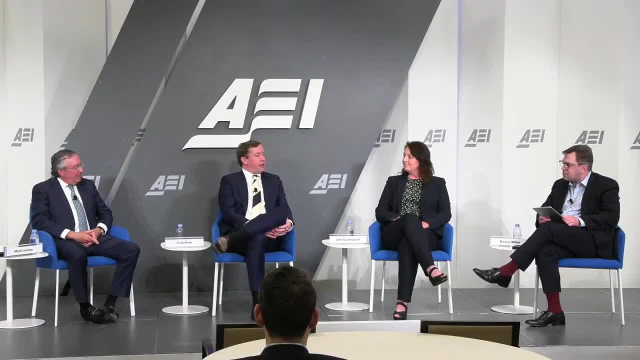 And I think creating some level of standard across each medical product center and then being able to have something that can quickly do- an initial baseline review that flags different datasets or different pieces of data that could be more interesting or require secondary or third or fourth level reviews from reviewers- could create just a faster process through. 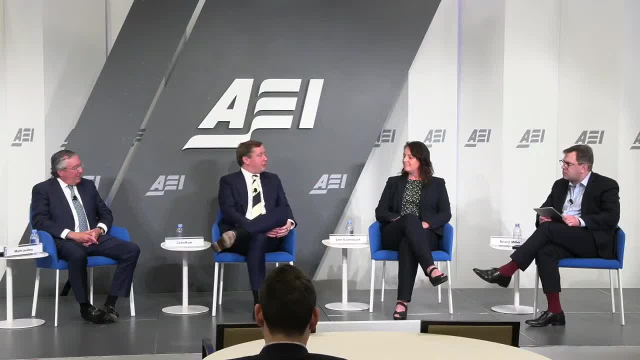 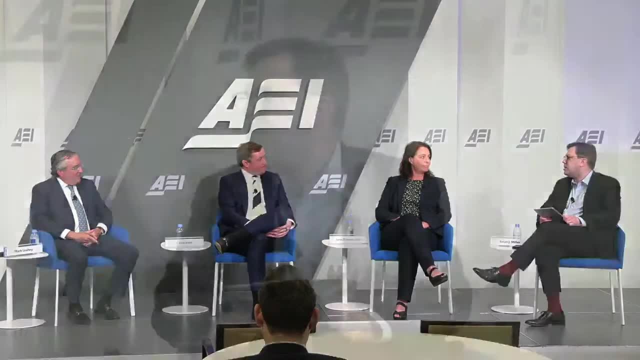 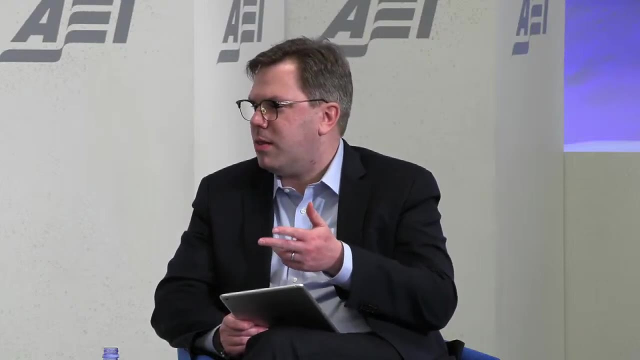 which there's. no. There's no sacrificing safety and efficacy, but rather flagging some of those more outstanding data points that could be helpful for reviewers, Or having some of the initial analysis be teed up automatically for the reviewers- the PharmTox team, the stat team, the medical officer who's doing the review- and then have 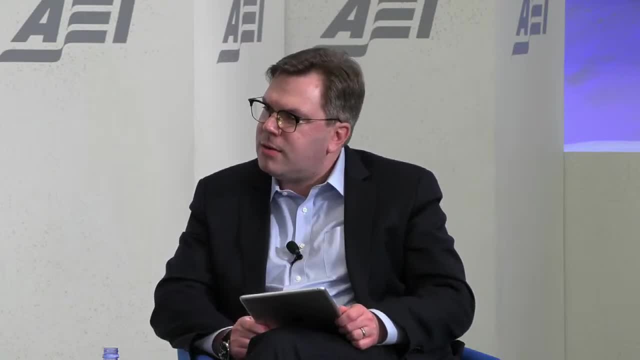 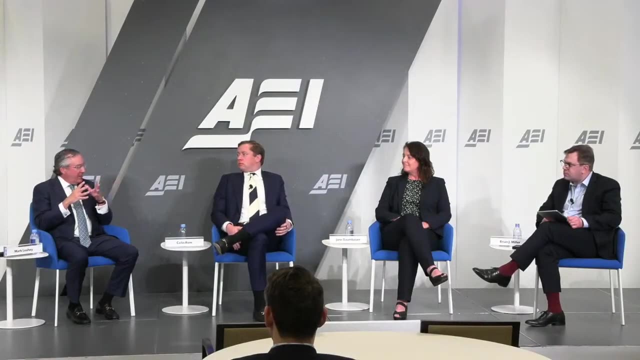 them be able to use secondary analysis on top of that. I would say too, again, quality in quality, out how this is being analyzed, making sure You certainly wouldn't want to lose the human element here. I'm not suggesting you. 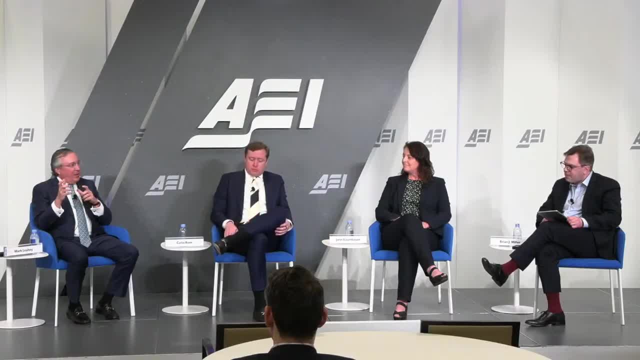 Because you could see the flip side of this. I think the flip side of this would be okay. it goes through AI. you've got a negative response and no person to go to and no reasoning behind it other than just think of a thumbs. 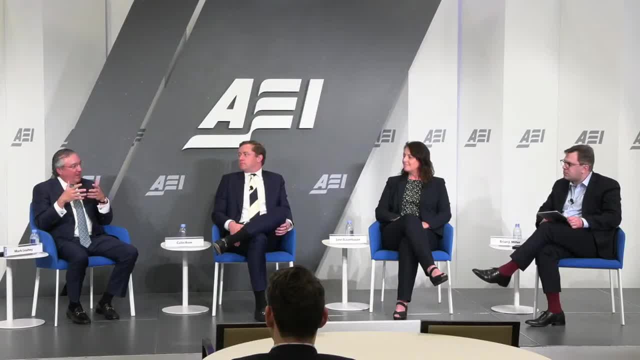 up, thumbs down, thumbs down, without maybe a nuanced review or without any information. So I think the ability to leverage technology to drive the administrative process with an FDA makes a lot of sense. Mm-hmm, And assuming we move down the road to have some of this help with the clinical and the 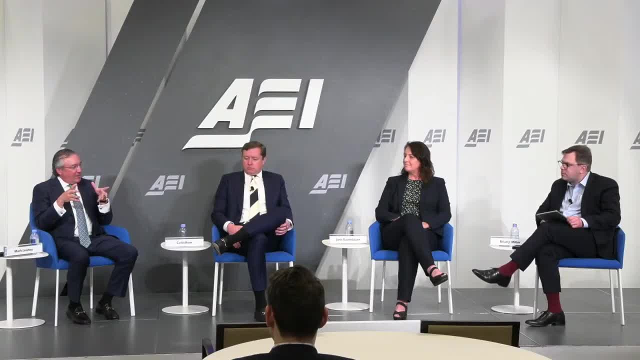 statistics and biocompatibility. I think, as long as it's quality, it's going to be helpful, because you said there is human error, but I know that the watch out has been okay in some instances. you still want to make sure there's a level of accountability to individuals. 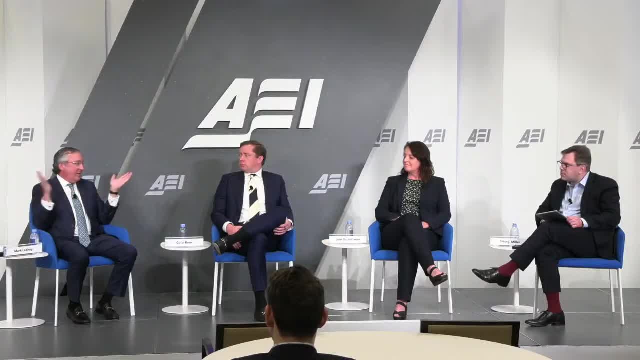 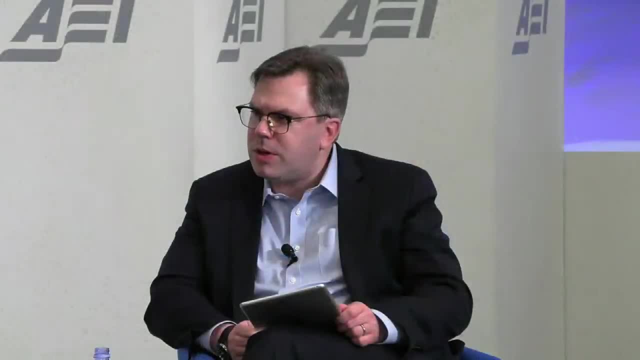 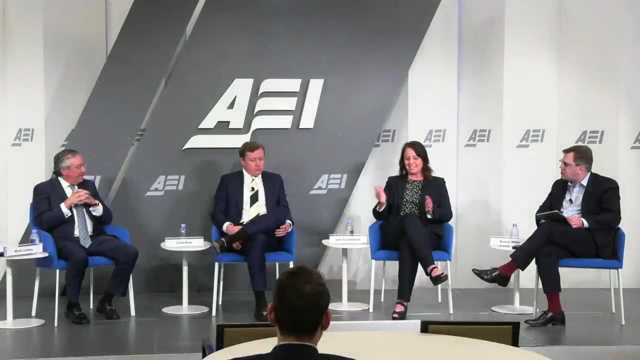 and they can't just say: well, this is what the system says, so our hands are clean and you're stuck Right. So more of an augmentation as opposed to an automation For now. For now, Although, again, at some point, the humans, I mean. this is what happened with chess. 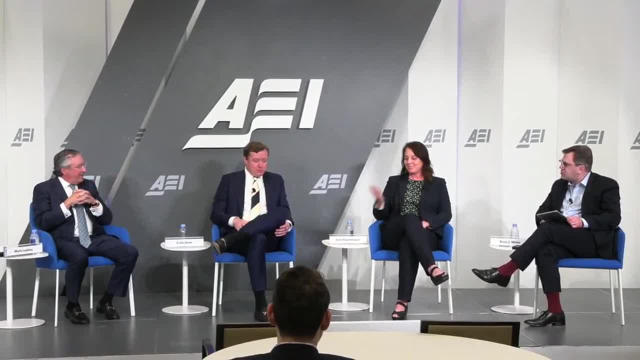 right. At some point, introducing the human review is going to introduce more error than yeah, And that's the natural evolution. and someone said whether it's drones. I mean, at some point, if this all works as we intended, you would drop a box in a third world country. 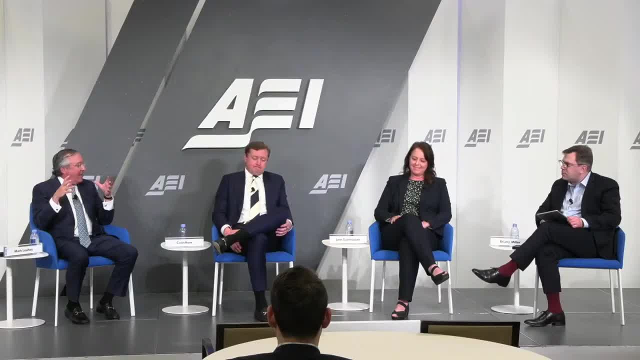 and someone walks in and they're getting diagnosed and maybe there's someone remotely and that's 30 plus years down the road. but there's great opportunity here. But if you're telling me in the here and now where FDA is going and leveraging AI, I would 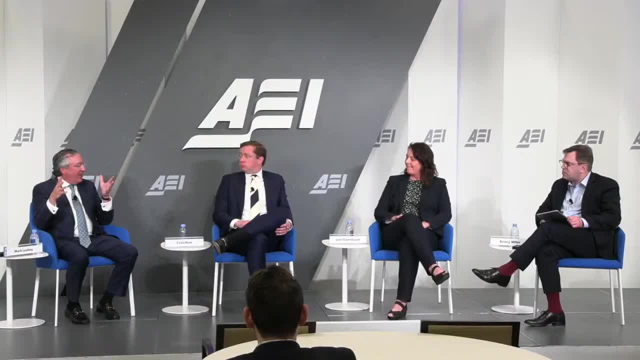 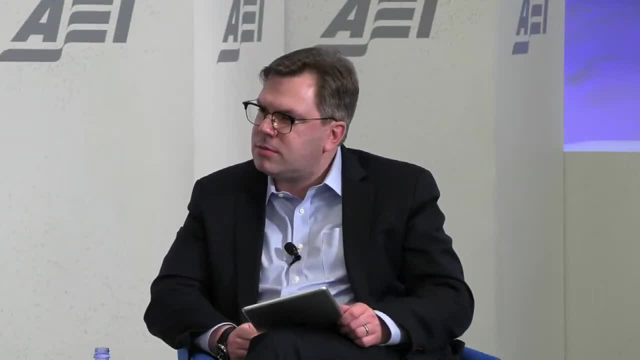 not want to say: well, our model said that you're a no-go and that's the end of the discussion. So maybe something like assessing application completeness, for example, Right, Well, you're seeing, actually in the device space with the E-Star. and to Colin's point, 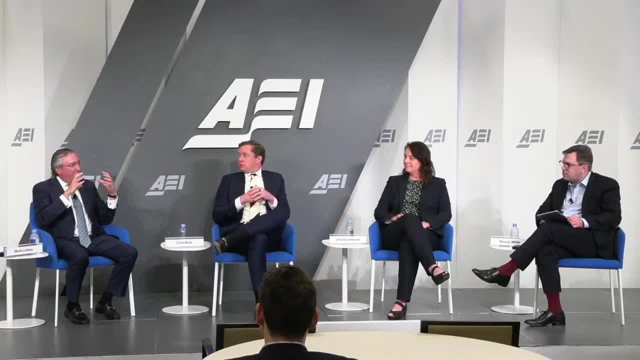 this is helpful for both industry and FDA- the reviewers- where it's a structured submission- Here's what's in. here's what's in. There's links to the guidance document And it allows you to be searchable. So there are already a lot of automated functions here that are digitizing this. that makes it. 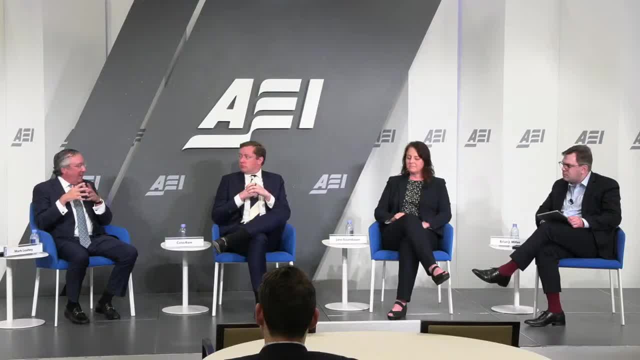 more efficient And optimizing. that makes a lot of sense. And again down the roll. could there be some decision support for the reviewers? Sure, I, just I think we want to make sure we take a prudent approach here. Agreed. 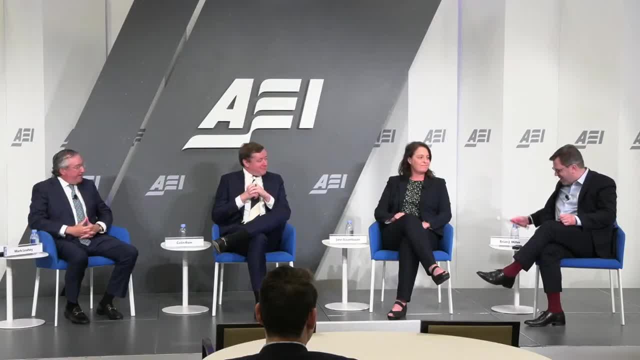 Well, this has been a very interesting discussion that has gone to some areas where I did not expect it to go pleasantly, so I'm continuing to read the questions. Thank you, I agree. I think we all continue to remain an optimist for AI and automation in medicine thinking. 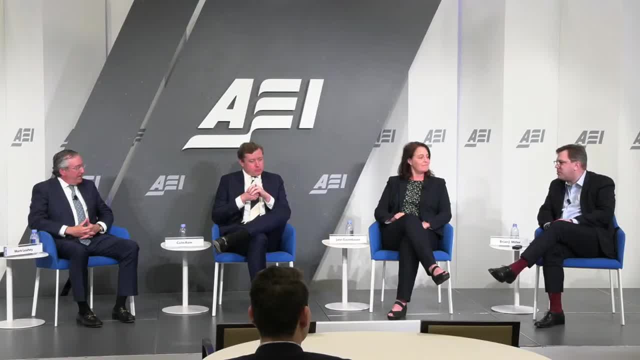 about improvement of administrative process, augmentation of clinicians, reviewers, administrators, patients and also automation of elements. I don't think we're going to be facing a terminator scenario anytime soon And I think that there's a lot of work for us to do. answering questions about helping 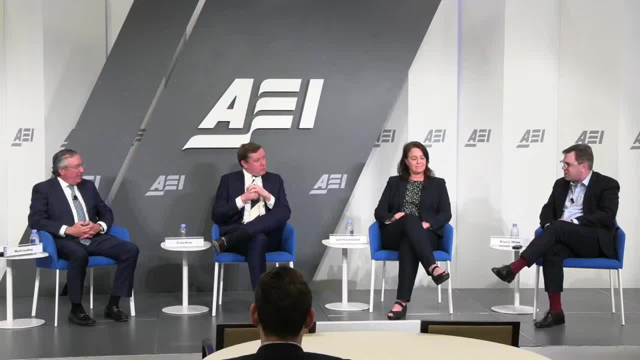 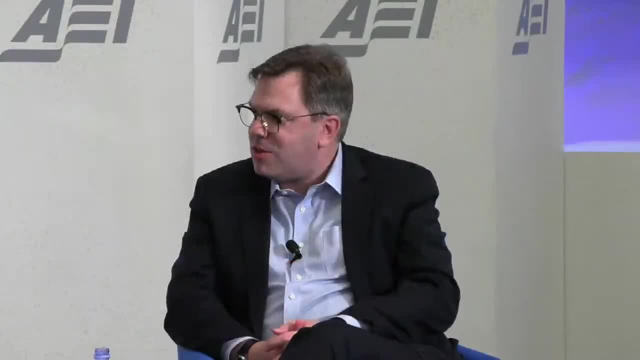 the FDA handle this space And can we do that? Absolutely, We're going to continue to handle it. What we're going to do with payment, because right now it's the valley of death in terms of getting these products reimbursed, either from payers, public or private, or in a direct 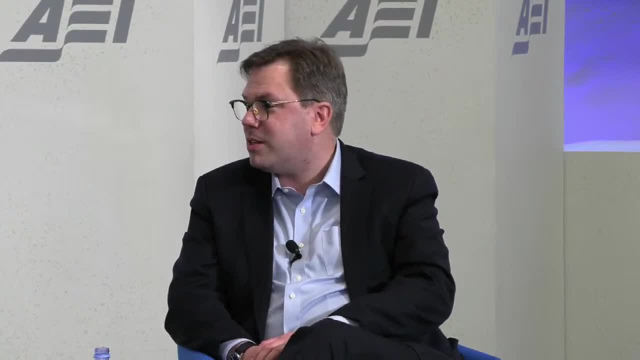 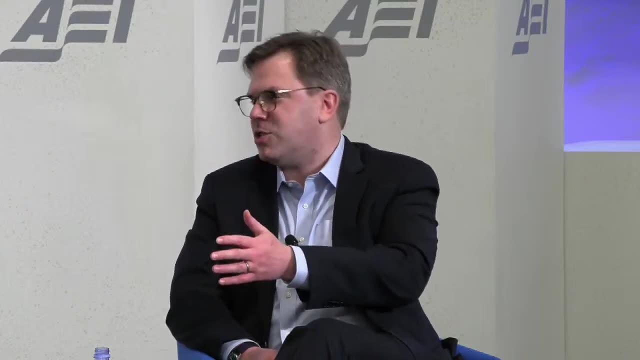 to consumer setting. And then, of course, there are a lot of liability questions to be answered, parsing between clinician hospital software developer, slash device manufacturer or even the consumer. I still think that, despite that, we're going to continue to handle it.